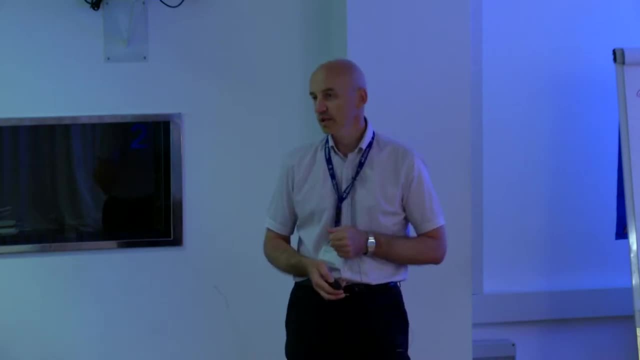 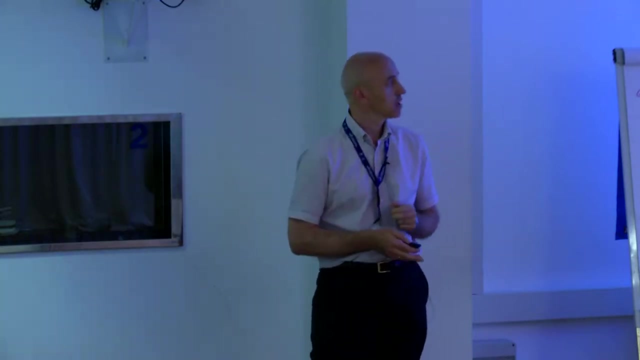 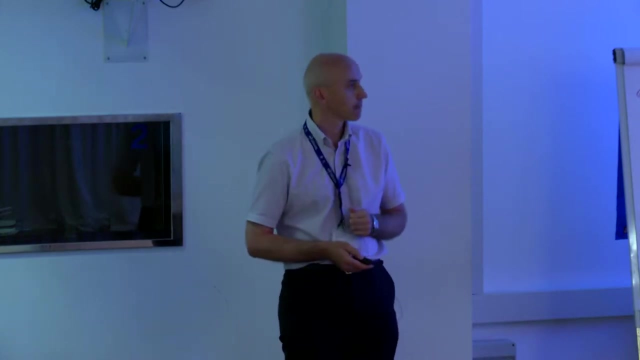 that you take the heat and add turbine and generate electricity. So you see that the the principle is there. So first of all, there is this direct comparison between research reactor or reactor in general and reactor which generates electricity. Now, to understand how this system works, you need some. 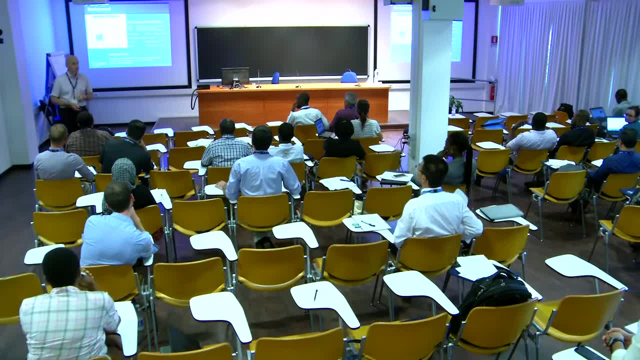 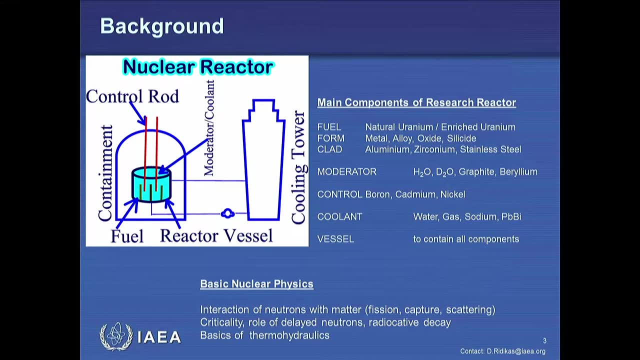 basic knowledge of nuclear physics and, if you want to go in more detail, some nuclear engineering. So you would need to understand the interaction of nucleus with matter, understand the process of fission, capture scattering. You will understand the concept of criticality role. 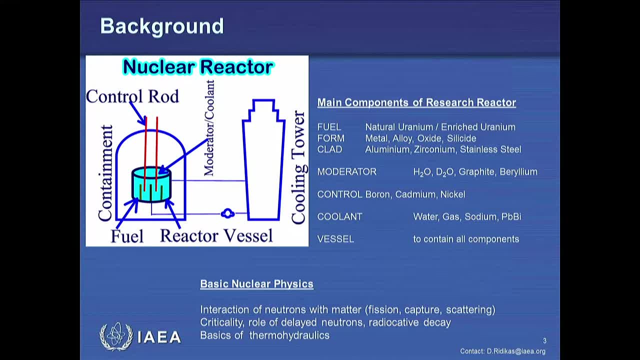 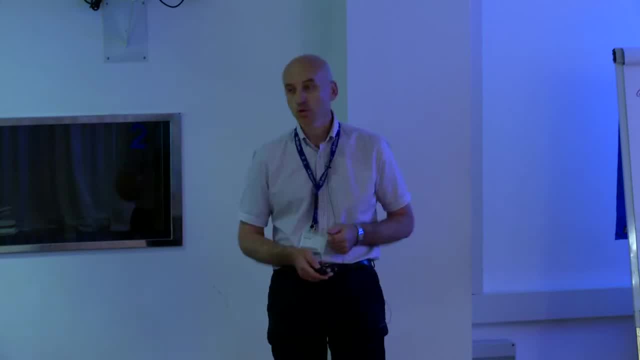 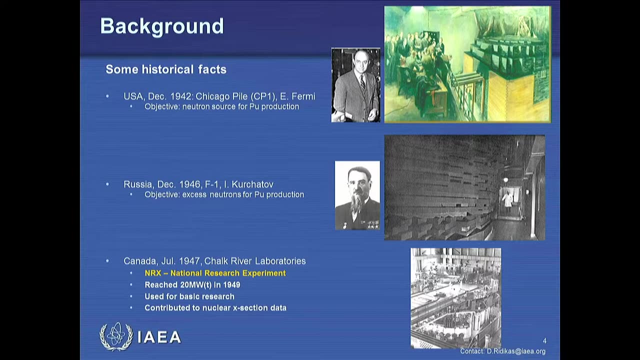 of delayed neutrons, radioactive decay and also basic of thermohydraulics, because there is a heat exchange, either just to cool the reactor or go from higher temperature to lower and turn the turbine for electricity generation. History is equally very important, because this is. 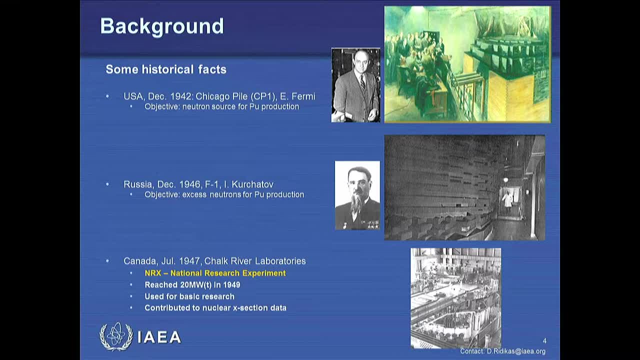 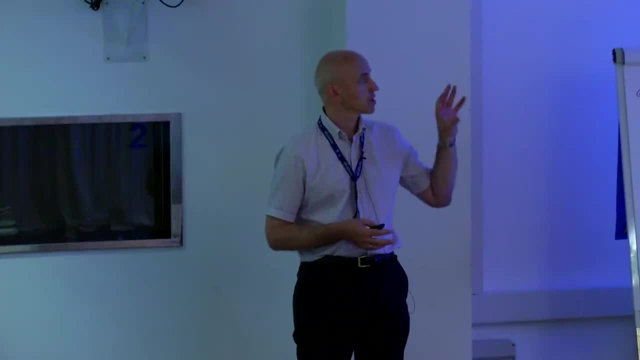 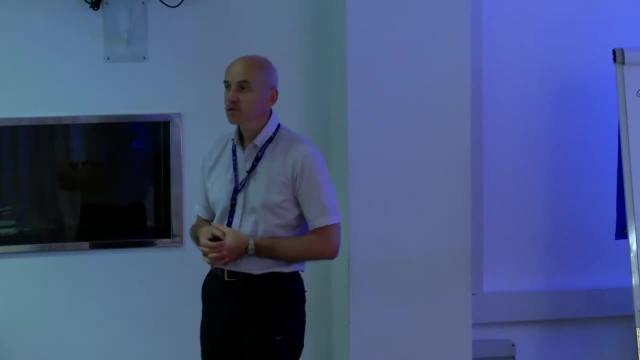 where all reactors have started. So the first two important people, Fermi and Curciato, working in the former Soviet Union and US, worked on a project related to creation of nuclear bomb. The research reactor was a source of neutron to generate plutonium as a fuel of the nuclear weapon. 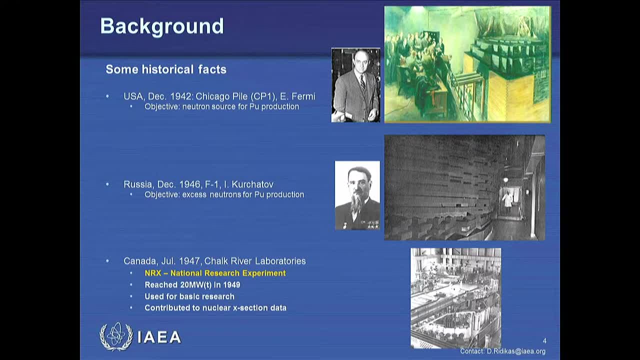 So the historic first steps of research reactor are not very bright in that respect. The first research reactor which you really can call research reactor was built in Canada with the main purpose for basic research as a source of neutrons and measures some neutron-induced cross-sections. 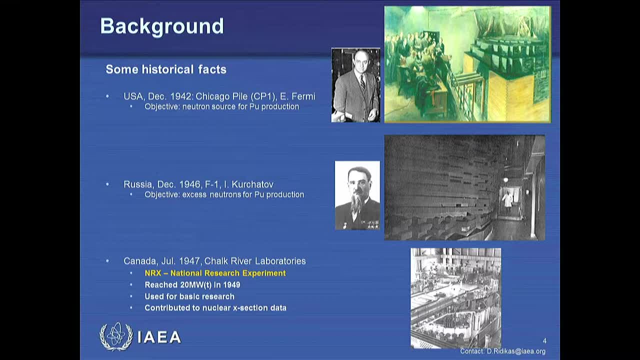 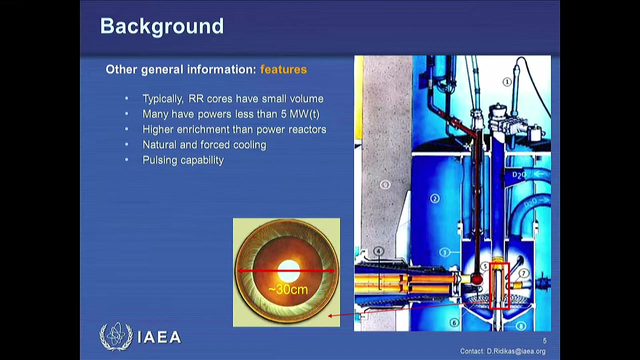 And that happened in 1947 in Chalk River Laboratories. I know you have a friend from Canada here, so maybe he can explain to you a little bit more about what has happened there. This is the slide which you have to understand because 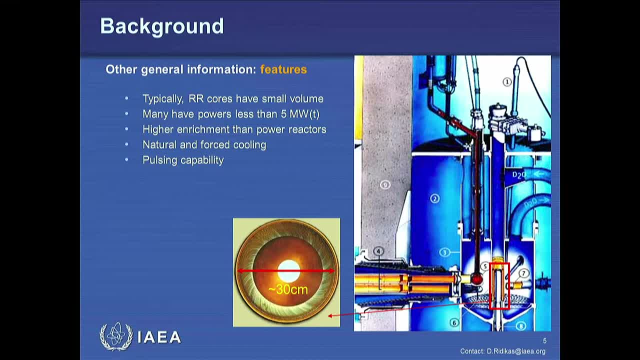 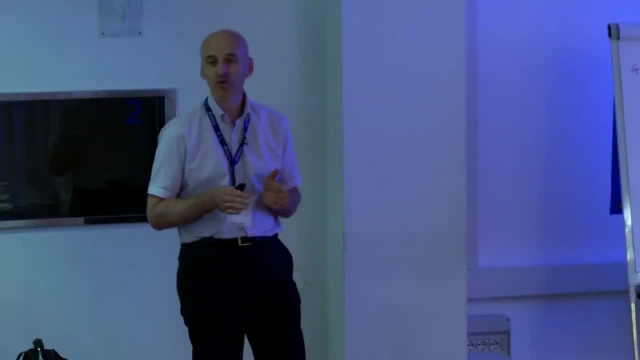 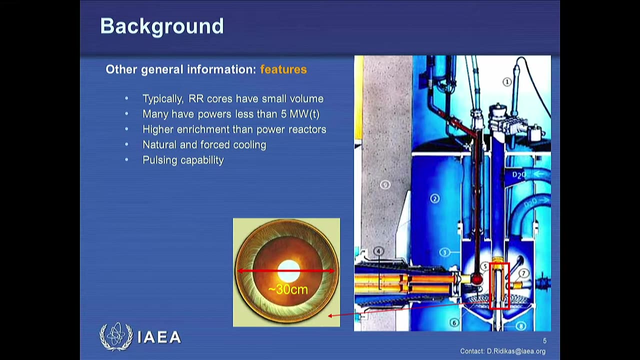 there might be a question in your exam. So if you understand that, you answer one of the questions already. So what are the main features, or what actually distinguishes research reactor from the nuclear power plant? The first is that typically, research reactor cores are very 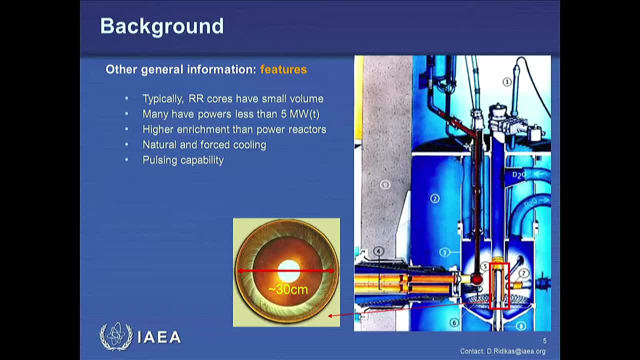 small And you see this is very powerful research reactor running in France, south of France, in Grenoble. The core diameter is only 30 centimeters wide, So these are very small machines in that respect. Many of them have powers less than 5 megawatts. 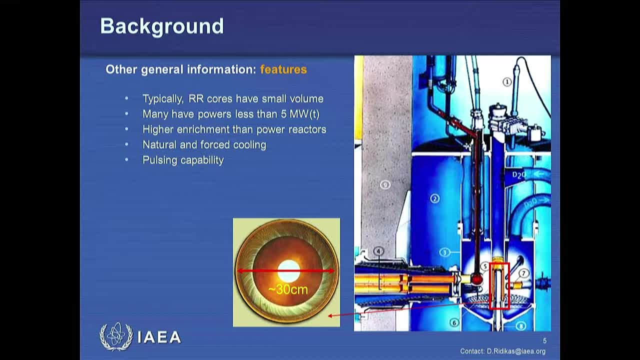 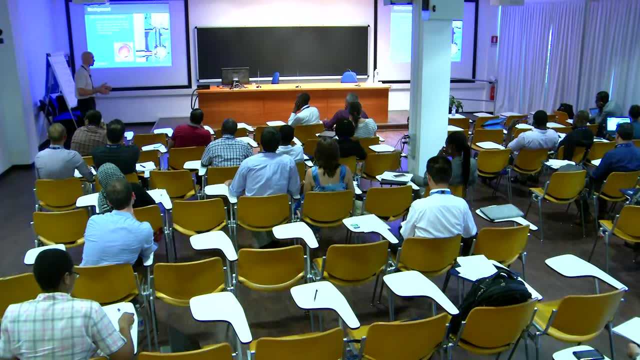 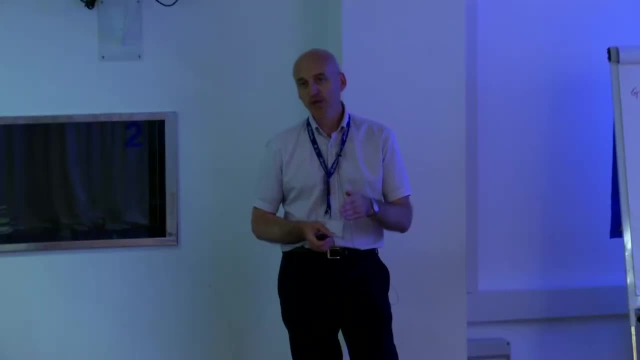 What is the power of a nuclear power plant? Yeah, we have orders of magnitude. So this is another important feature to distinguish research reactor from power plants. We touched a little bit today in the morning enrichment level of the fuel, And research reactors would run typically high enrichment fuel. compared to nuclear power plants. Nuclear power plants today operate up to 30.. They operate up to 3.5, maybe 5% maximum enriched in terms of uranium-235.. Research reactors still LEU. low enriched uranium would operate below 20%. 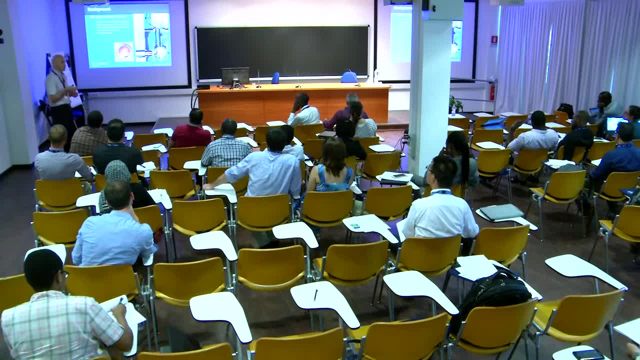 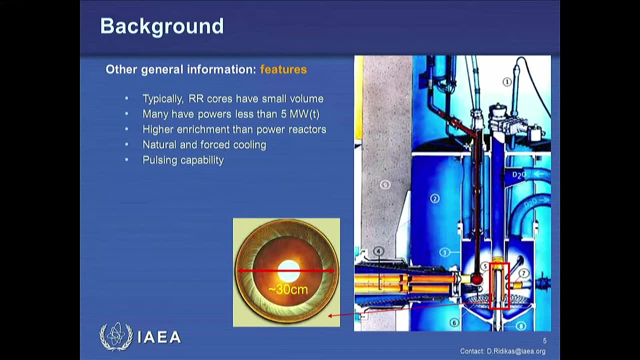 And there was a big program still ongoing to convert highly enriched uranium reactor cores to low enriched uranium reactor cores. Research reactor can run on natural or forced cooling, depending on power. So there are no way NPP can run on the natural cooling. 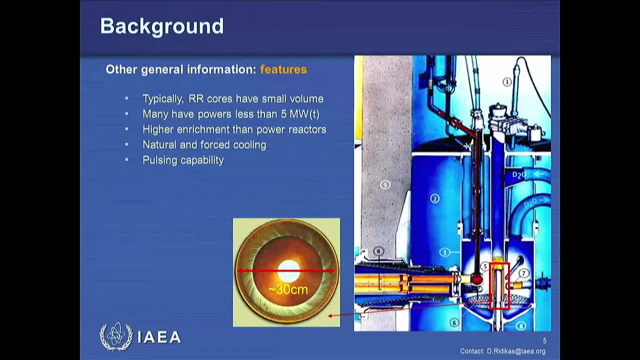 because there is a much bigger power generator And research reactor, depending on the design and purpose it was built, can operate in the pulsing capability. That means you enlighten the reactor, get a tremendous pulse of neutrons and then it shuts it down immediately. 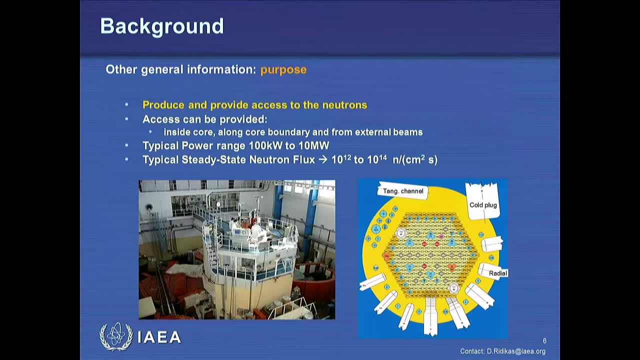 So it goes promptly to critical and then shuts it down Again. what is the purpose? It's a source of neutrons, And these neutrons can be provided inside the core where the fuel zone is located, along the core boundary or from. 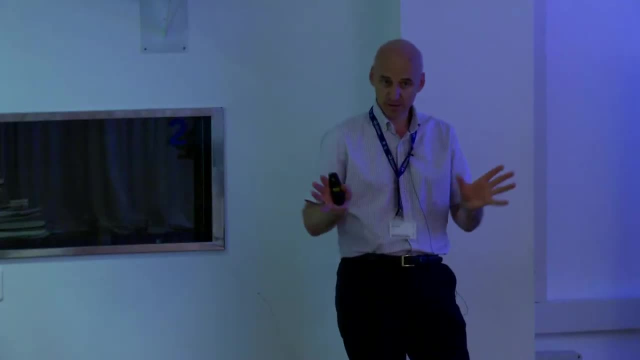 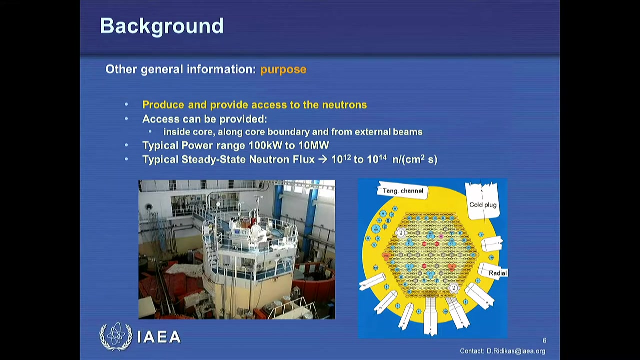 external beams. That means going through the shielding, typically concrete, and getting outside of the reactor shielding itself where you perform different kinds of experiments. I repeat: Reactor shielding. Reactor power can go from zero power to tenths of megawatts. 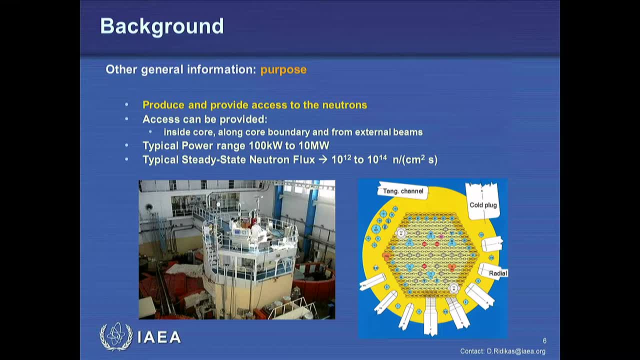 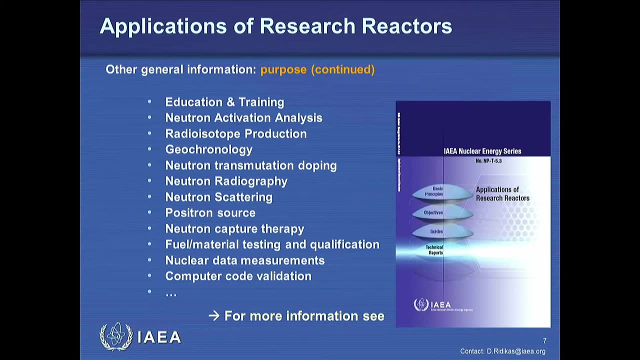 for research reactors, And that's the same for the neutron flux, going from very low fluxes up to 10 to the 14th, 10 to the 15th. Research reactors as a source of neutrons are used for many different applications. 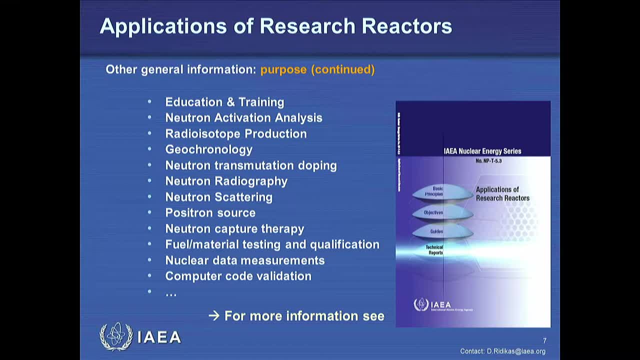 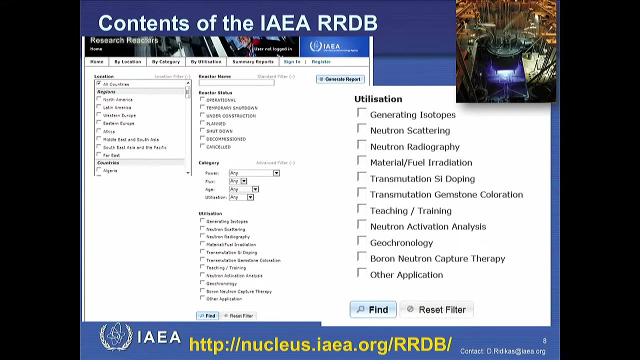 And I will go in more detail to explaining all that, From education and training, from analytical analysis, production, neutrons, Neutron scattering, neutron, radiography, imaging, nuclear data measurements, computer code validation, et cetera. More about research reactors you can learn from IEA research. 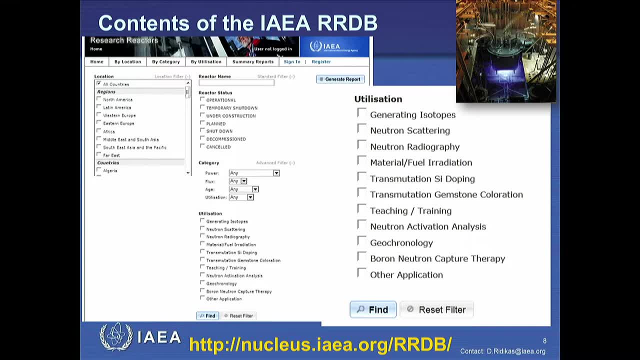 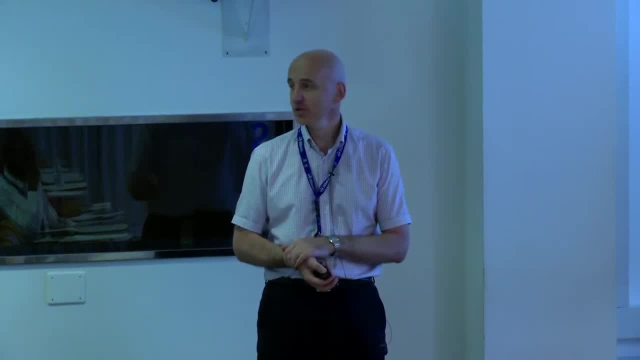 reactor database. So typical exercise, what we give after the lecture or maybe during the lecture. you go there using your laptop and find if you have a research reactor running in your country or in a neighboring country, And what kind of reactor is this? 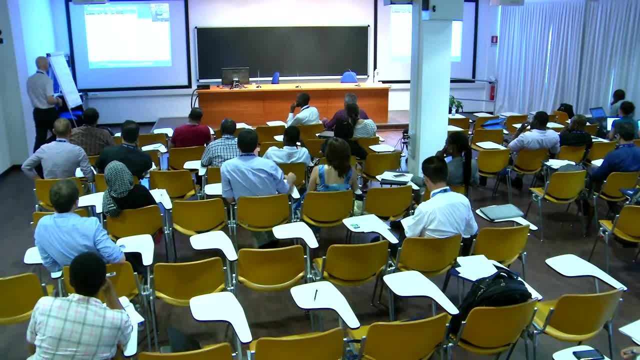 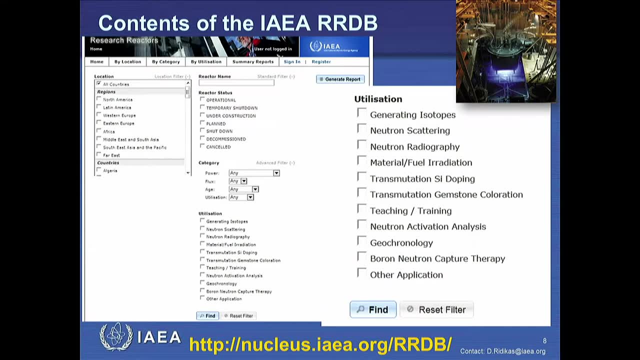 What is it built for, et cetera. So this is interesting, So you can look for research reactors in different countries, regions, If this is operational or shut down, and what kind of power level, flux, age And, last but not the least, for which purpose it's operating. 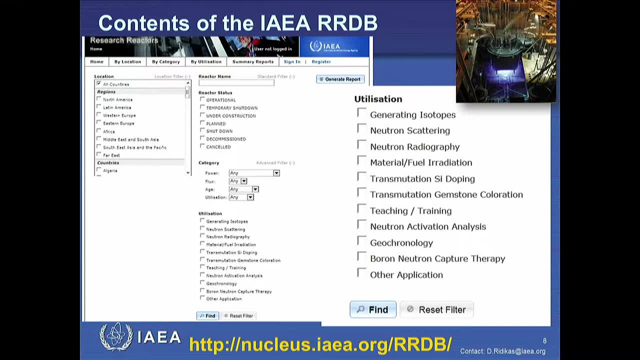 Is it mainly for neutron scattering teaching, training? Maybe it does some geochronology studies et cetera. So all that can be found in this database, A bit about history, History we count. today at least. this database has more. 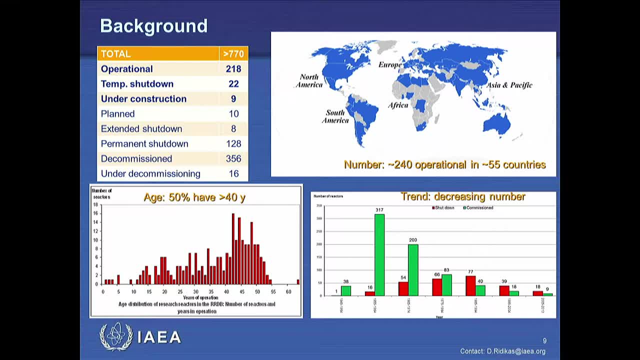 than 770 research reactors registered in the database. That means these facilities have been built historically. We count today 218 operational, 22 on temporary shutdown in 55 countries. You see, research reactors are in all continents, as is shown on the map. 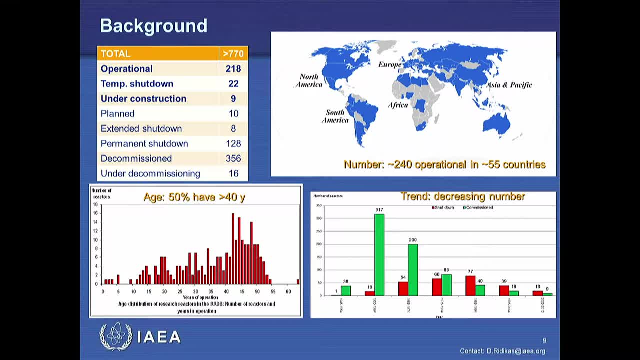 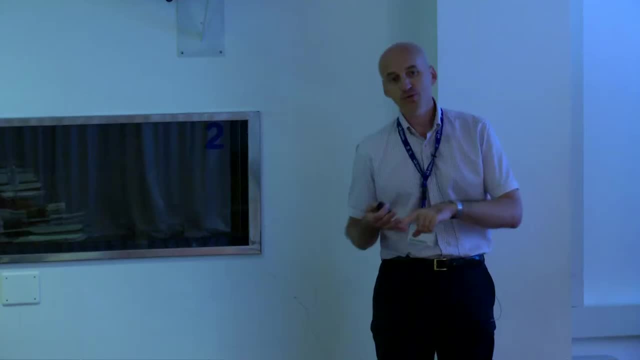 These are very old facilities. Most of them were built as part of the research reactor Atoms for Peace program in the 60s and 70s. That means that 50% of operating research reactors are older than 40 years. That means that also there is aging management issues. 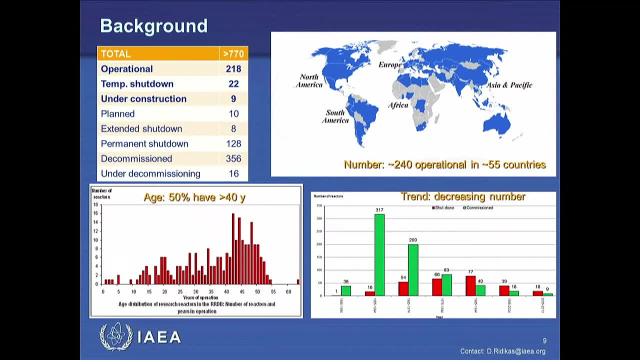 and challenges for these facilities And it also defines the future trend of operating research reactors. You can see on this slide the number of research reactors shutting down compared to those you know Newly licensed From the 70s- 80s, there are two times more shutting down than 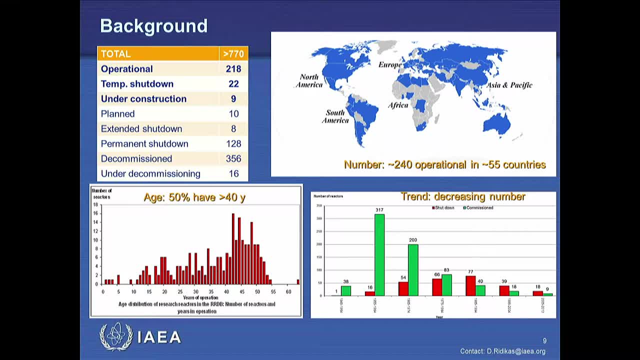 new reactors coming. That means that this number will continue to decrease as the time goes. One of the reasons that these are old facilities and if country doesn't have a need, country does not have a need or the country has no budget to replace old reactor by new. 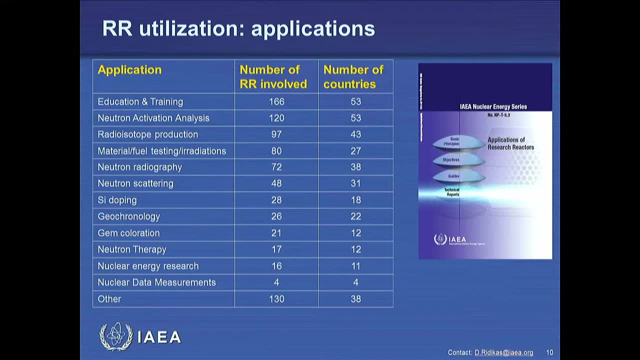 meaning country will not have a need. They will have a research reactor. This is a statistical distribution of number of research reactors providing particular application. So out of 230, 40 research reactors, more than 50% provide support to education and training programs. 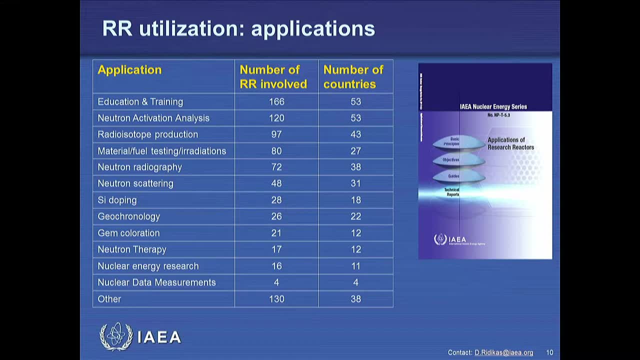 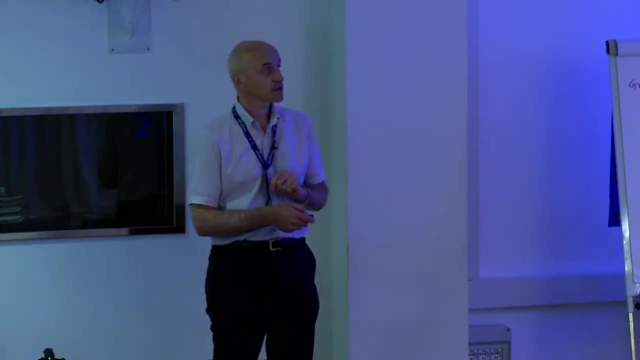 120 reactors do some neutron activation analysis. And the third biggest application is the production material: fuel testing and radiations nuclear. I will go and explain what these applications mean for those of you who are not familiar with that. A good reference to learn about these applications is the. 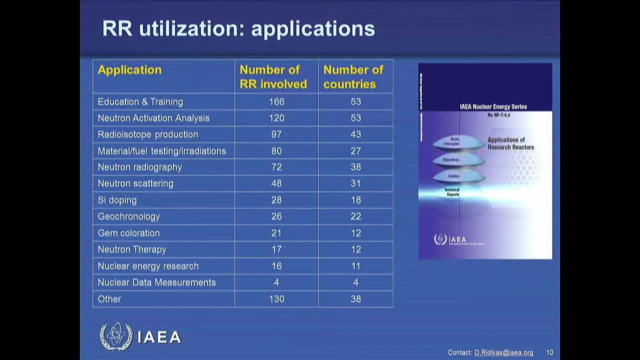 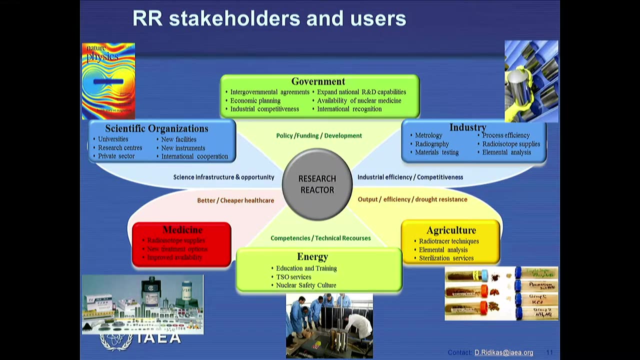 recent nuclear energy series application on applications of research reactors. Now, this is an advantage and a challenge for research reactor, As long as nuclear power plant generates electricity. nuclear power plant generates electricity. to the nuclear power plant electricity, everybody is happy. so you have typically one client or one user. 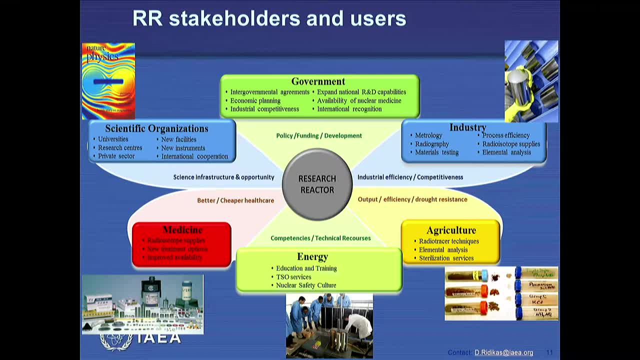 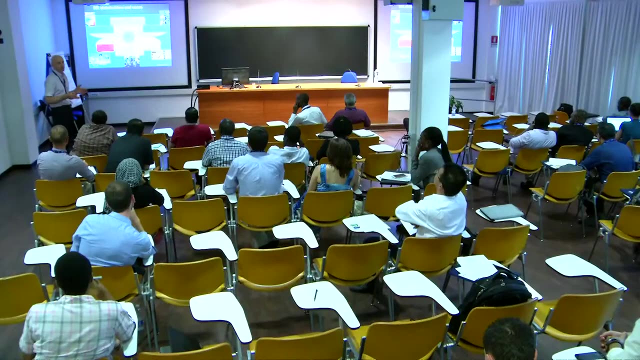 this is consumer of electricity. so in that respect, on commercial basis, NTP provides a service very broad client is a public generating electricity. research reactor is not money generating machine. it will require funds from the state all the time. yeah, so if you believe that you can build a research reactor and make a 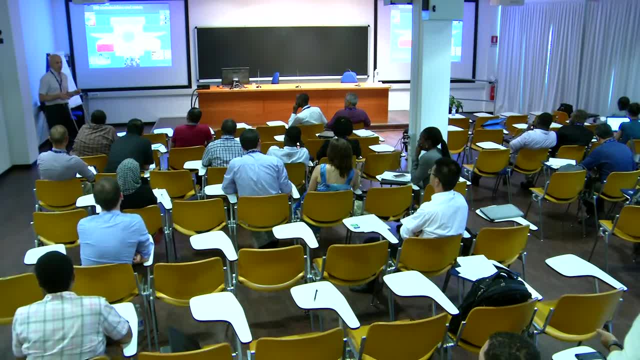 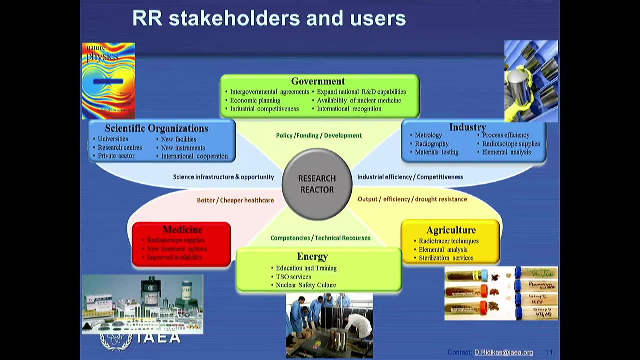 business out of it. I would say no, there are some exceptions, but in general that will not happen. so that means policy funding and development will be defined by the government in most of the cases. research reactor would be a single national facility supporting the very broad area of 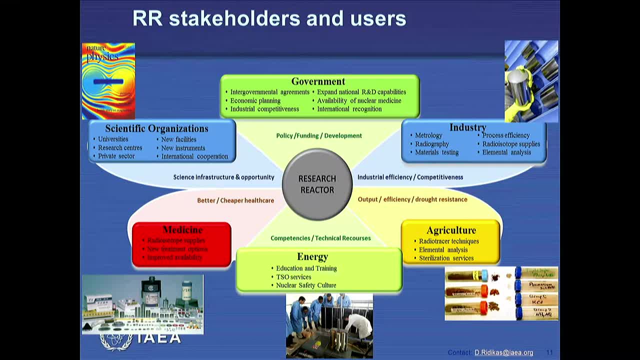 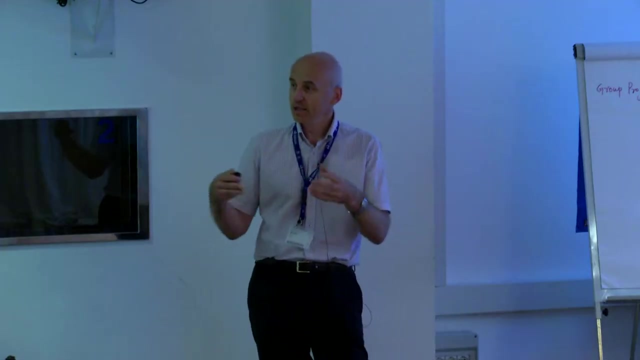 application. nevertheless, there are many opportunities where neutrons can and are used today in different applications. these can be found in sectors of industry, agriculture, energy, medicine and not forgetting research institutions, including universities. so there is a great opportunity but the same time, there is a challenge, because research reactor as an organization. 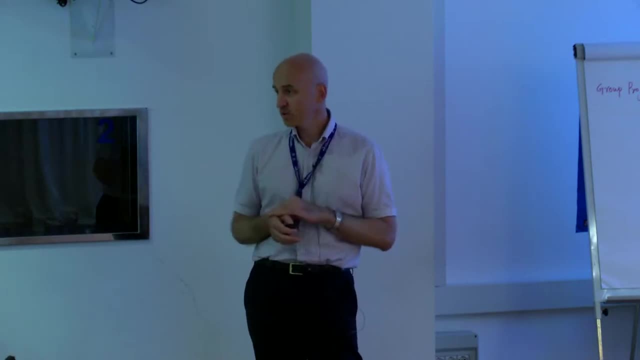 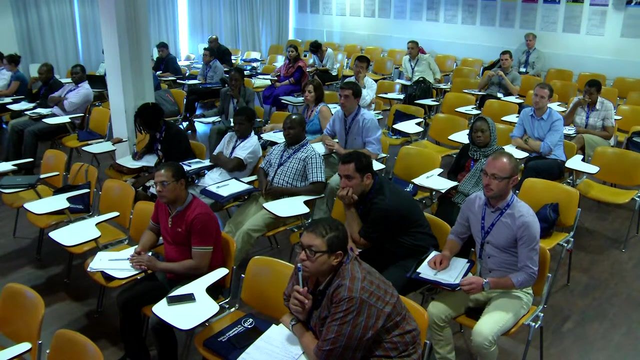 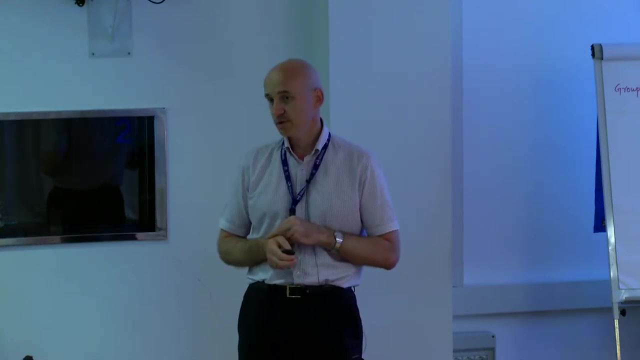 the deals with very broad range of stakeholders. So, being a reactor manager, maybe you're a very good operator of reactor, but you might be very bad or unknowledgeable to manage different stakeholders. This is one of the challenge today for research reactors, because you need to communicate with 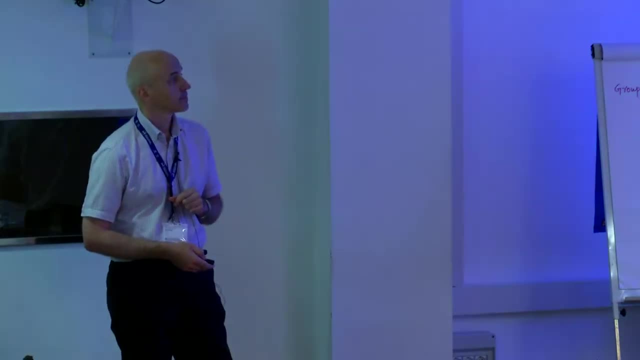 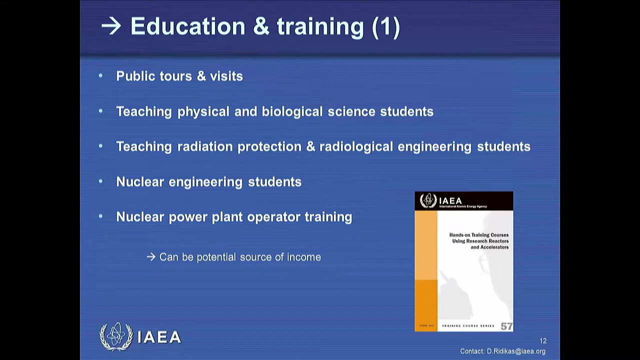 many different people in understandable language. I will go now, one by one, to explain you in more detail. applications of research reactors, and all of the applications will have two slides. The first one, what do we mean, And the second, how it is done. okay, 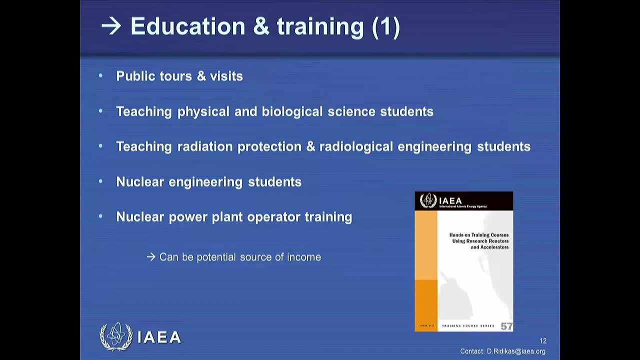 So research reactor: you learn about reactor physics. So you start learning by visiting the facility and you will visit NTP, maybe, research reactor- I don't know if this is in the program, But you will know about it. So you start learning by visiting the facility and you will visit NTP, maybe, research reactor- I don't know if this is in the program, but you will know about it. 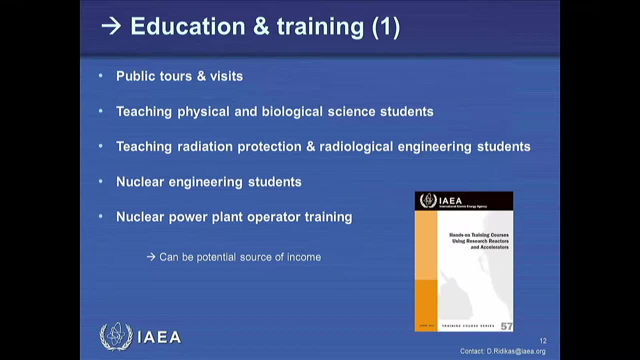 So you start learning by visiting the facility and you will notice that this is nuclear installation. So research reactor can be used for teaching physical biological science students, more adequate for teaching radiation protection, radiological engineering students, nuclear engineering students in particular, and in some countries nuclear power plant-operated. 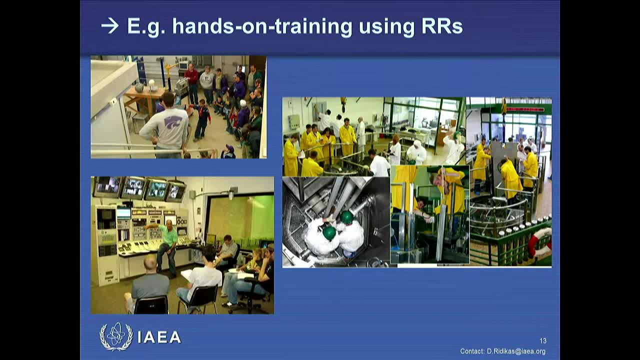 training. Okay, So how it is done depends on the level of education and training activity. actually, You will go walk through just introducing. You can go visit, you leave. you are still alive, right? this is what it's all about, yeah. 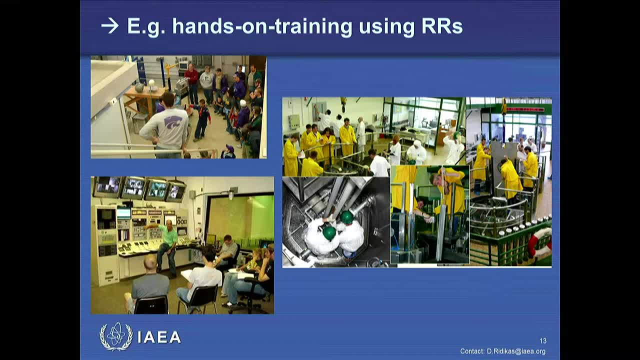 Now you can go and be more serious really: hands-on training touching different components, performing experiments, loading and unloading fuel- All that is possible with the research reactor as part of your education curriculum. You can go even more further In operating room. you will be allowed. 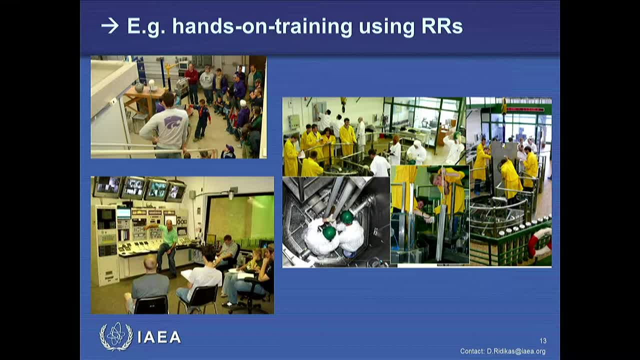 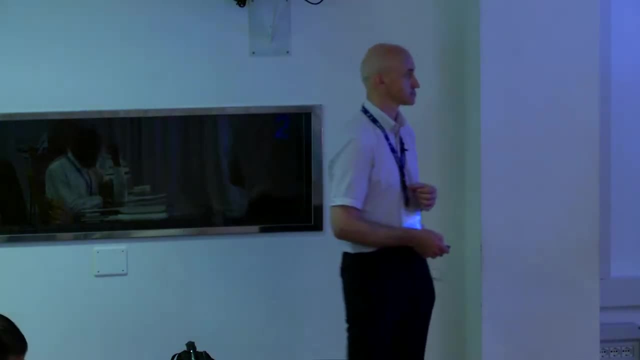 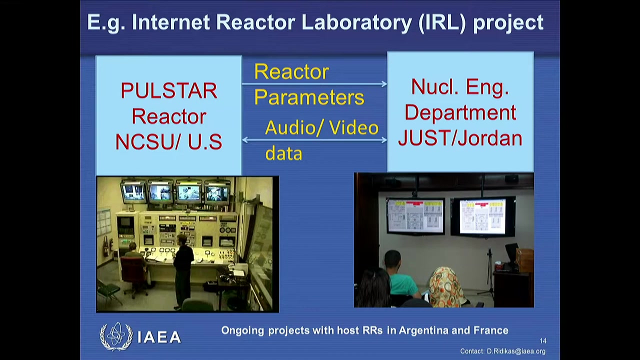 Even some research reactors. to start and stop a reactor, You as a trainer, of course, with your supervisor behind you, but this is a great experience. This is real feeling that you start and stop a chain reaction. You can do that remotely by connecting operating research reactor with the outside university. 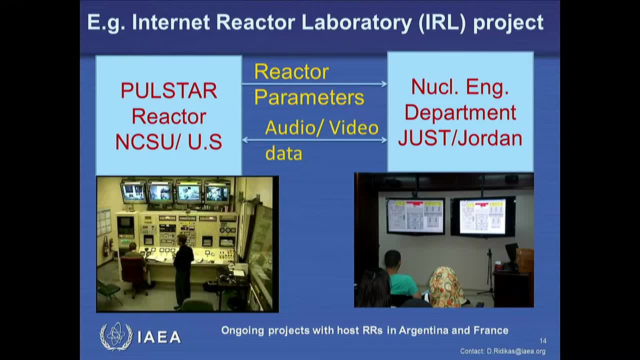 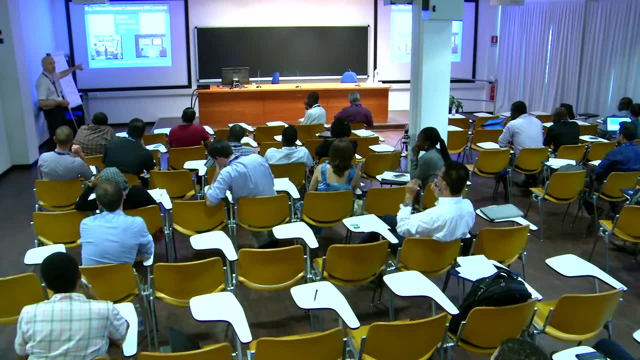 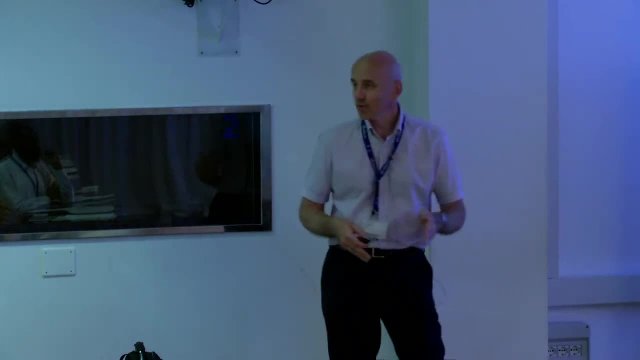 or organization in another country, for example. Without having such a facility, You would perform online experiment. You will transmit through video conferencing the images, what has been done physically, but also reactor parameters, So you can do your lab course not going to reactor. 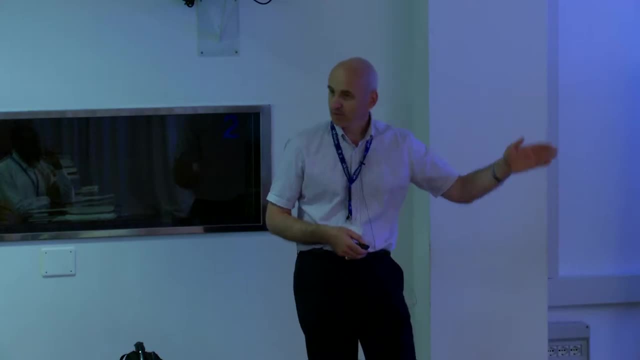 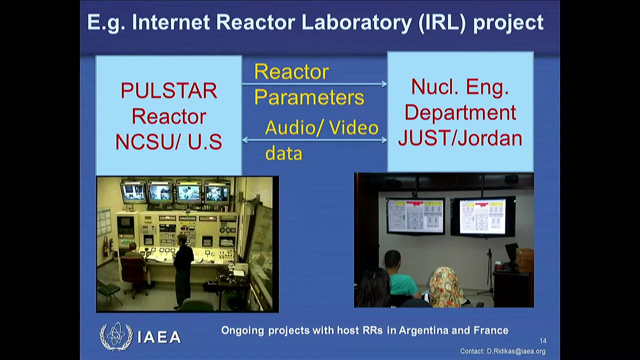 You can communicate and ask operator. I want to start now. I want to withdraw control rod and he or she will do the job for you, and I think this is efficient way to introduce reactor physics and nuclear engineering for the countries and organizations who do not. 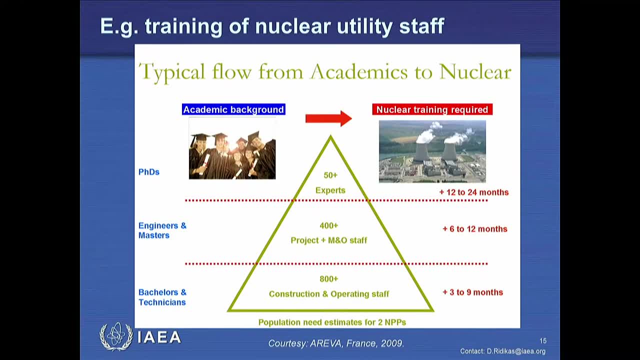 have direct access to such facilities. We also think that research reactor has an important role to participate in overall human capacity building for nuclear power, Because nuclear power personnel requires different areas of technical expertise at different levels. This is an example of two NPP blocks in one nuclear power plant where you would need 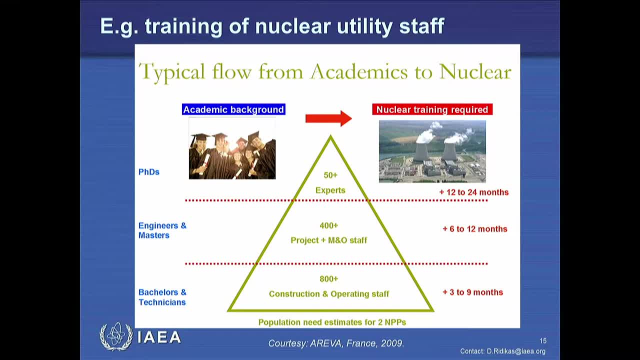 to train about 1,000, 1,200 people, And this training includes two stages. You need people with the right academic background, meaning graduates of the universities or high schools. Some of them might be required as a bachelor technician level, some of them master in engineering. 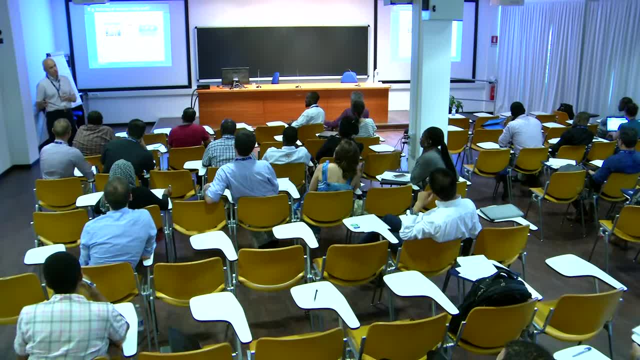 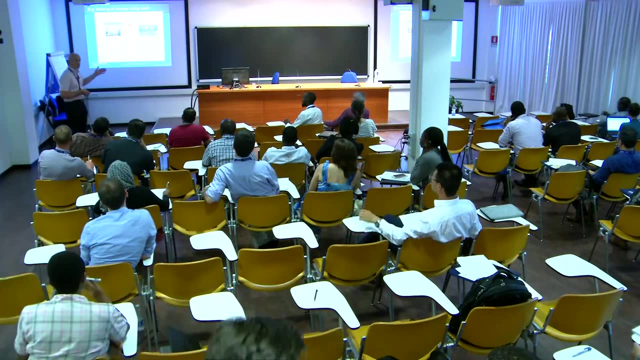 and some of them PhDs, typically managing the nuclear power plants or projects related to nuclear power plant. This is the area where directly research reactor can contribute as part of the university curriculum. Now, after graduating, even if you had some training on the research reactor, you will 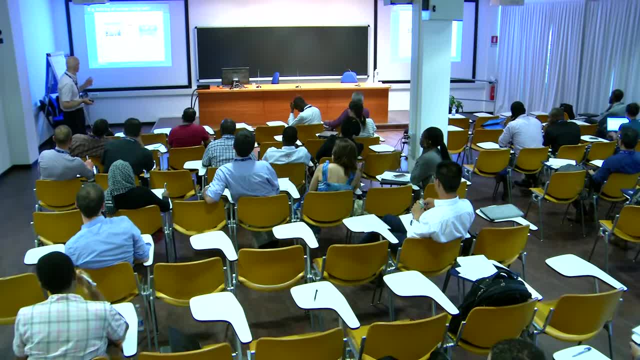 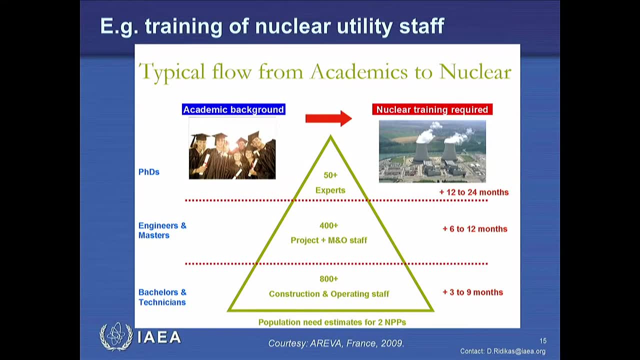 not be able to work at nuclear power plant. You need a special nuclear training And, again, depending on the position you occupy, You will need additional from three months to two years to be able really to step in and have a job as a utility staff. 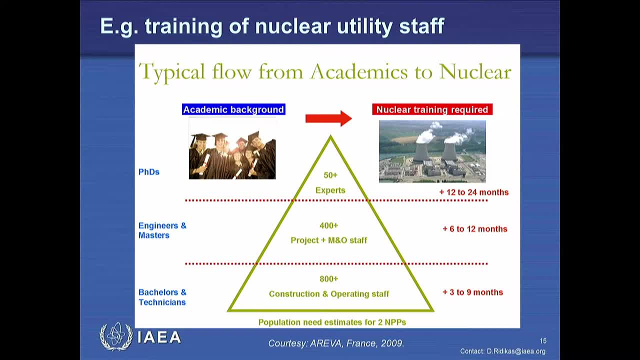 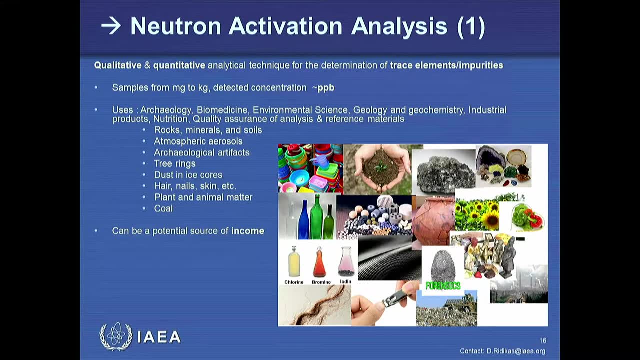 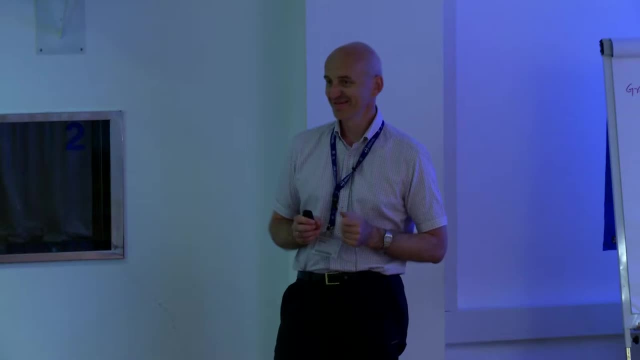 So again, in this special nuclear training, in some areas research reactor can help you to prepare these people. Next application: You're doing very well. Only a couple of you have closed eyes, so it's not so bad. So second application: 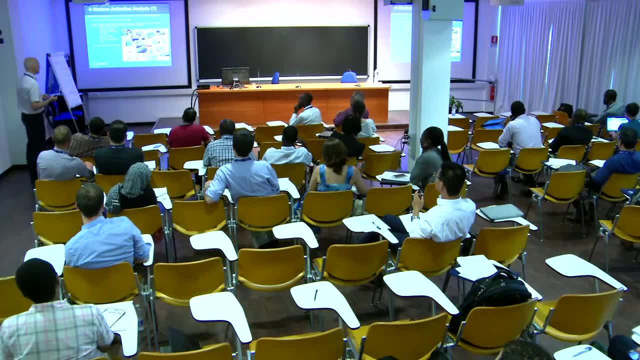 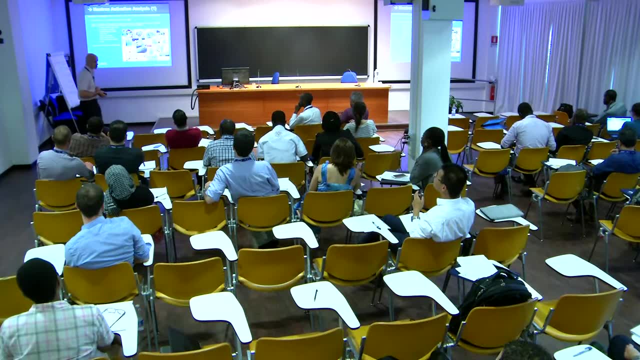 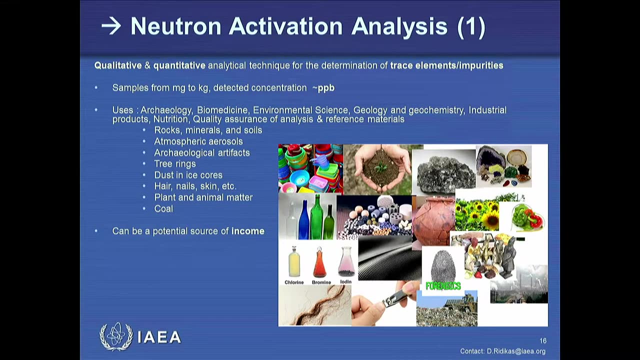 That's neutron activation analysis, As the definition tells. activation analysis: you put a sample, you irradiate and you measure something. And that's the qualitative and quantitative analytical technique to determine trace elements in various samples. These samples can come from different sectors: archeological, atmospheric dust, hair nails. 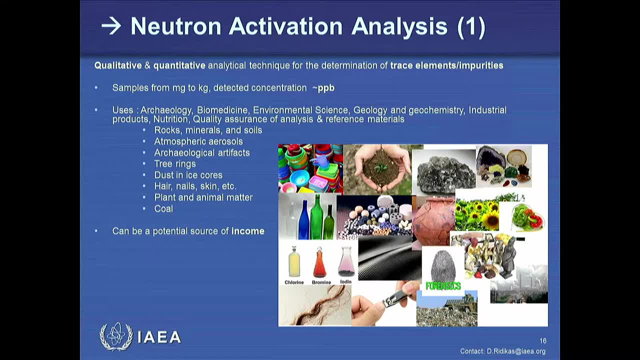 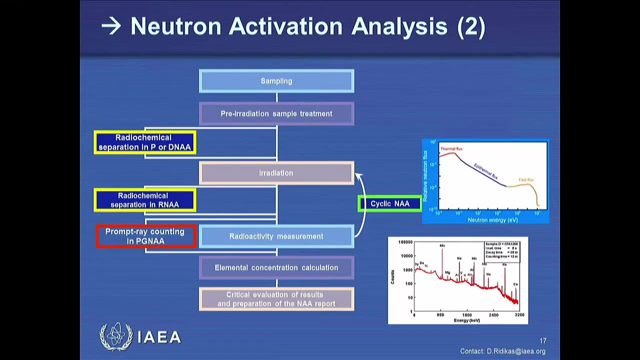 skin, plant, animal, You list it. It's all kind of samples where sometimes you need to know at impurity level if this matrix has a certain element or isotope, And the research reactor can do that. You start with the sampling. 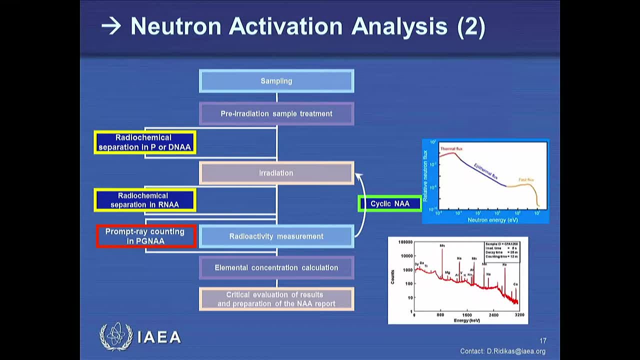 You do irradiation, You create radioactive elements. by putting some gamma spectroscopy, you're actually able to determine at which extent gold is irradiated, And you can do this. You can do this. You can, of course, test thePMC mode with the US下次 region. 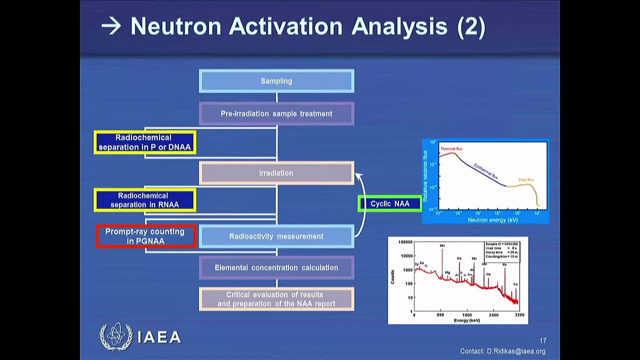 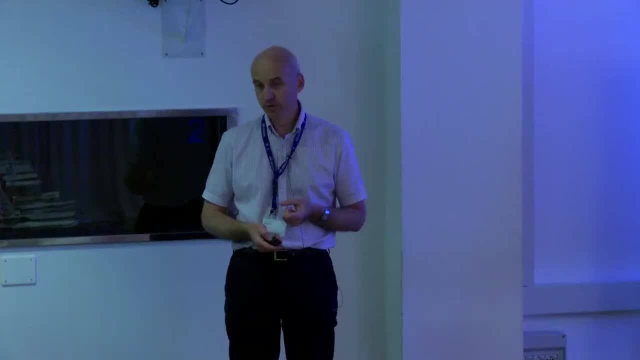 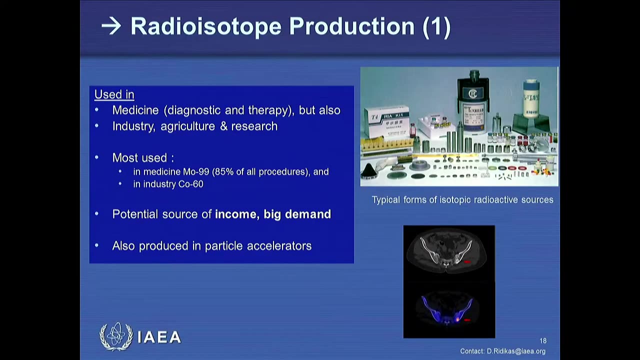 And the most common mattes are then grade 6 to 92, up until gallium and the duodenal levels, And maybe we decided to test the same thing at number of different universities for data. we cannot run modern medicine without being able to perform diagnostics and therapy, and these rely 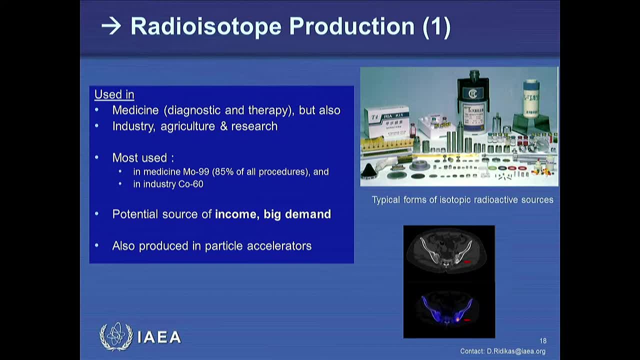 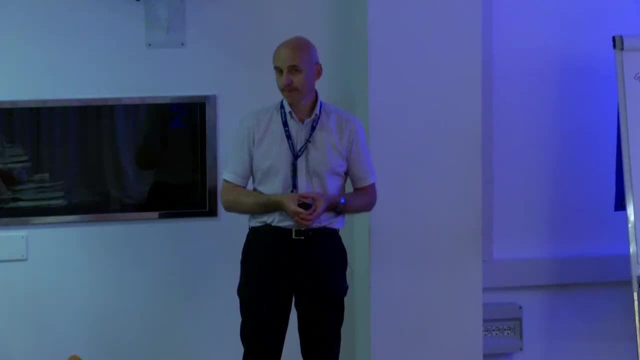 a lot on radioactive elements, but also radioactives are used in industry, agriculture and research. so if you come from the national research institution, you need to calibrate your detector and without radioactive source you will not be able to do that if you go and explore oil and gas. 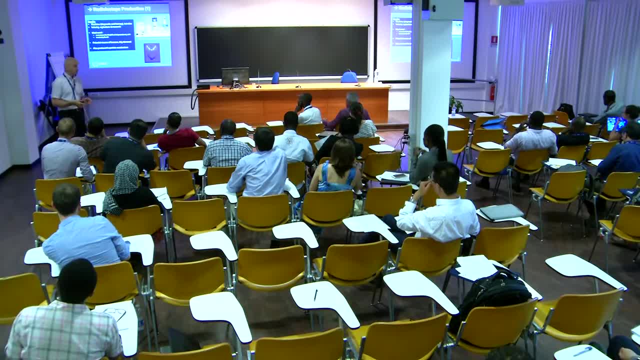 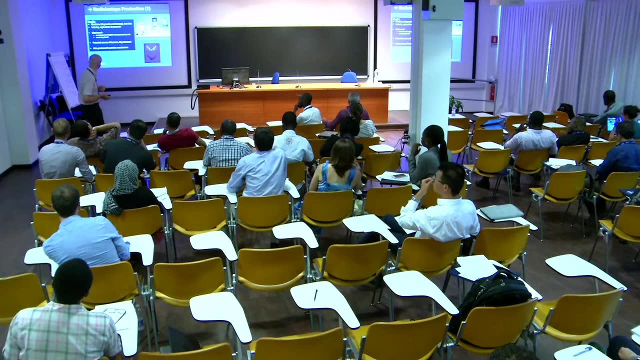 and to see if there is a leak in a pipe. one of the ways is to inject radioactive material and to see through as a tracer to see where this leak comes. so there are no most economical savings using, in some cases, such techniques. there are two most important. 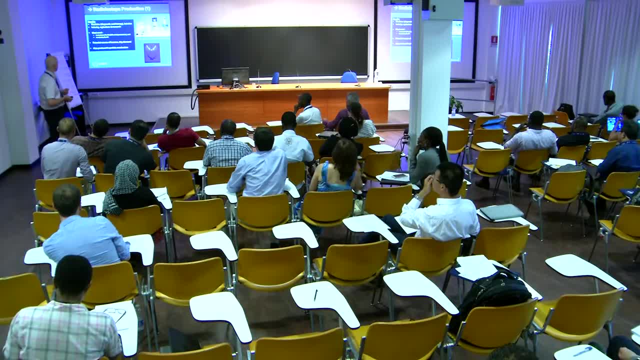 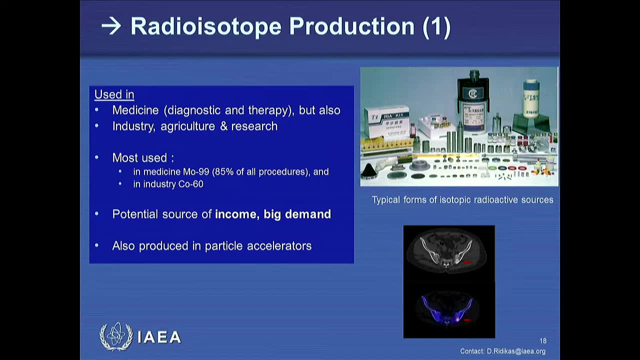 radioized. i think most famous and most known in industry. it's a cobalt 60 which also used as irradiator. you can irradiate food, wood, sterilize medical equipment, etc. because that kills bacteria. in general language speaking in medicine: molybdenum 99- 85 percent of diagnostic procedures. 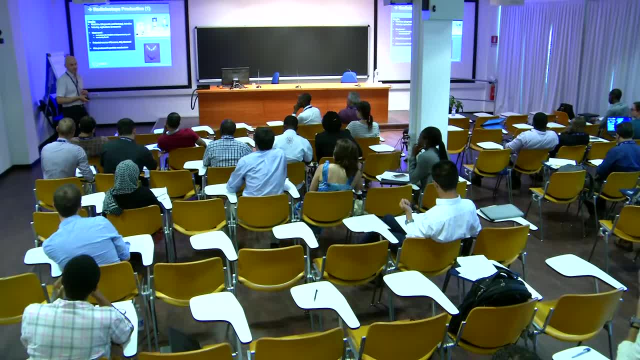 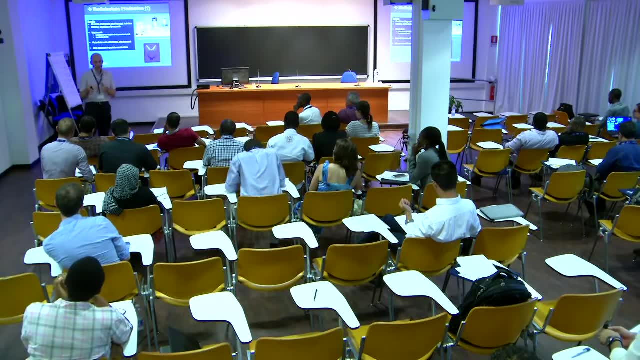 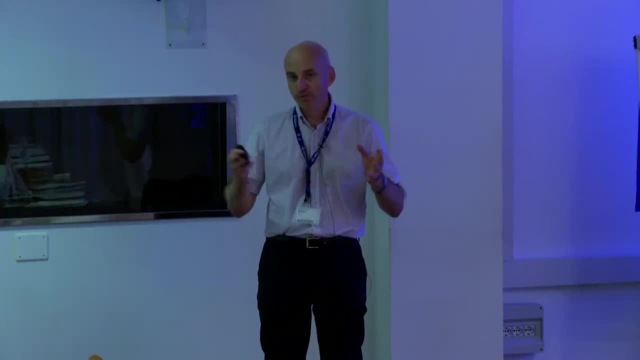 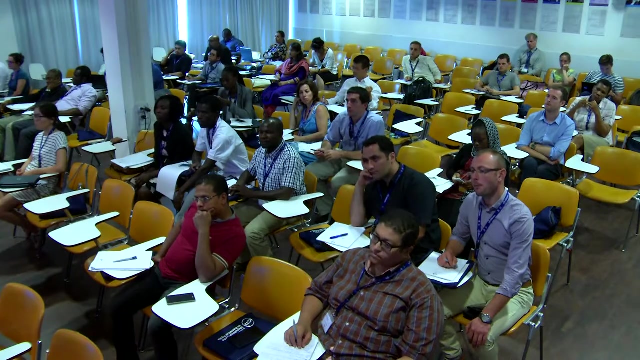 worldwide finding if you have a cancer or tumor somewhere in your body is thanks to this particular adjective, because it's a perfect characteristic for imaging purposes. so without this isotope you would not be able to predict and most probably prevent cancer development. how this is produced at research reactors: you start with the target material you radiate by. 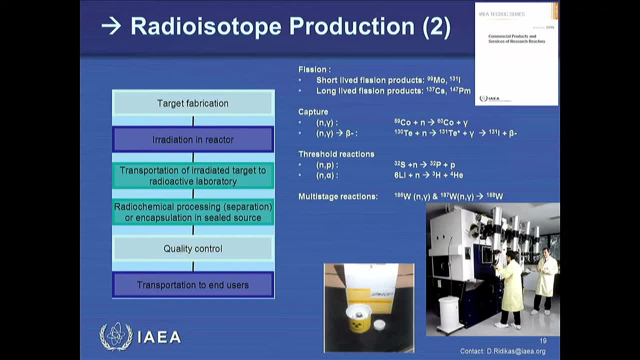 neutrons and you create a cobalt 60 phi in your body. and then, if they are working, in Moses, and you create a radioactive element. and this is an example of reactions. how, from cobalt 59, by adding one neutron, you end up with cobalt 60. how, in case of sulfur? 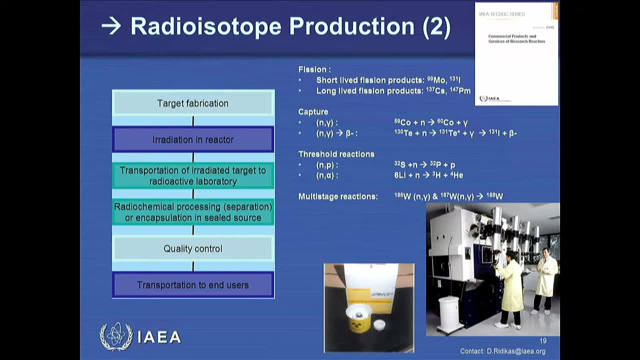 you get a phosphorus, for example. yeah, so these are number of examples. you start with target fabrication with certain quality assurance, quality control program. you continue at irradiating at reactor. you perform transportation of ready target to the hot cells, extract what is needed for your purposes radiation element, perform quality control- very important step because you 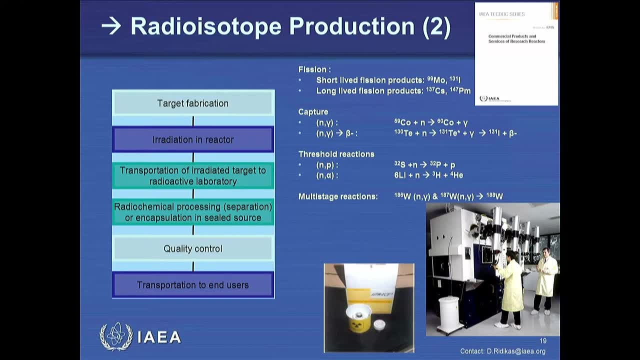 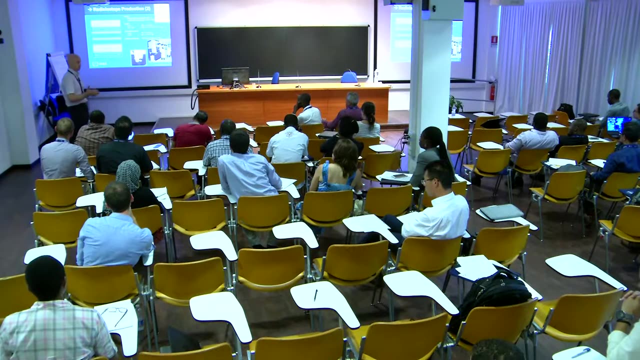 are bringing some of it to the medical hospital. transportation logistics is equally important, because if you're late, there is nothing to transport. it has decayed and that's it, and you need to restart from the beginning. so that's another important item, in particular for the short term. 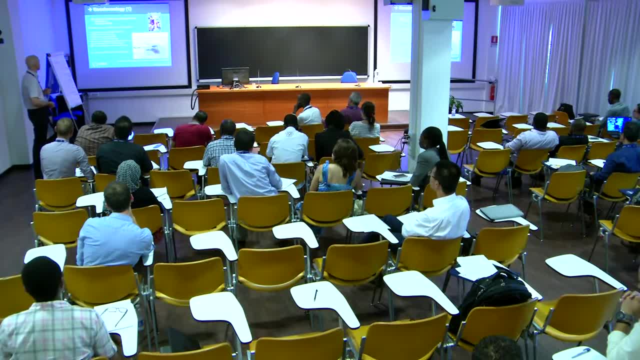 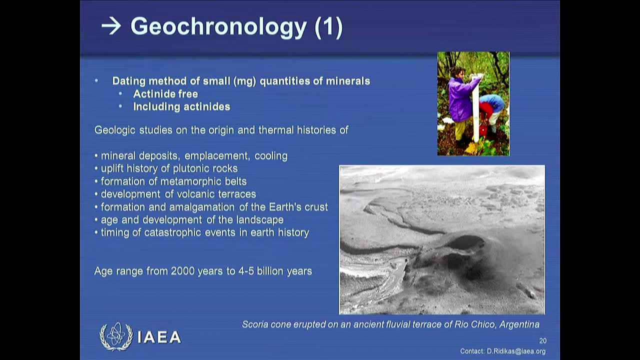 you can date objects. you can date rock and soil using a research reactor and depends if your sample has actinide or it's actinide free. you have two possible techniques to date back to the a few billion years, so here you rely on some elements which are 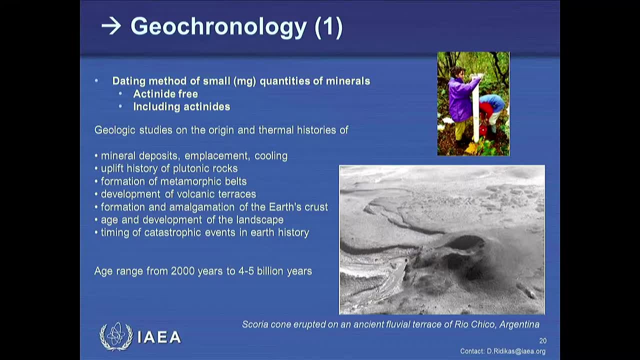 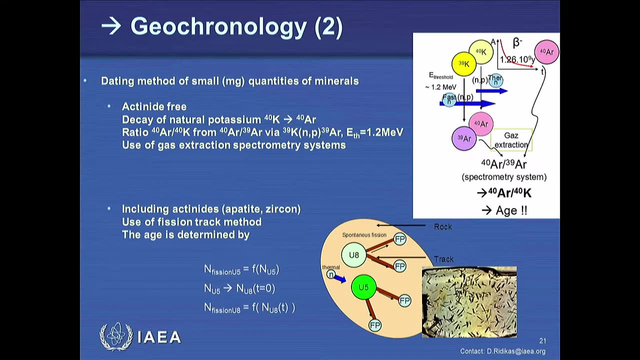 natural, naturally decaying with very long period of time and by looking at different proportions between potassium and argon or between uranium isotopes. actually you can date back the materials to very long periods in the past. again, you need to radiate, measure different ratios, and you're able to do that. this is very 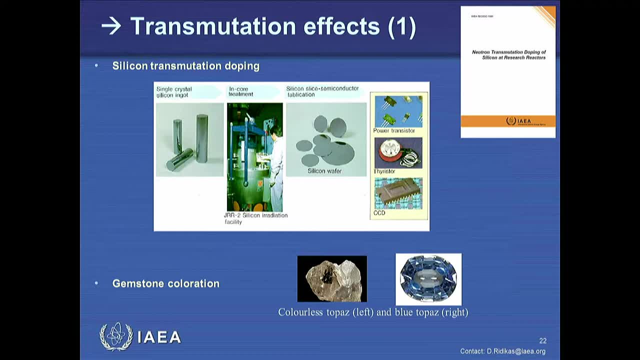 important. now on the data to record those based on the seasoning and톱 and its different 糥 amounts. results: it is up first irradiate some stones to add value to them, and you call the process gemstone coloration, when the stone without major value becomes a jewelry, as long as it's not too much radioactive. 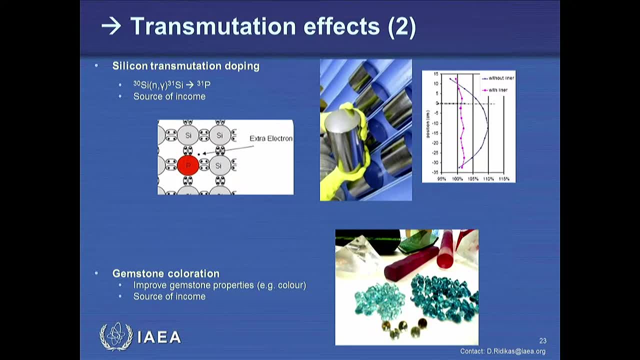 right. so how it is done, you start with the pure silicon ingots. you see the size, typical size. today, industry requires different size of ingots to be radiated from six, eight to ten inches, and this is irradiated in the reactor core in a homogeneous way. and what is happening actually? 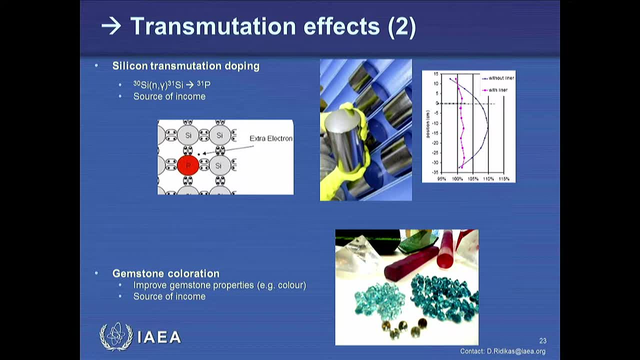 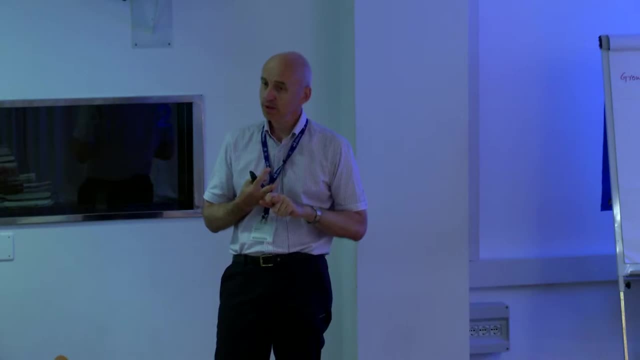 that silicon captures neutron and you create a phosphorous impurity which certainly adds value to the semiconductor material. that's the same you need for the gem coloration. you need to calculate exactly what are the neutron gamma fields required to make a defect in a lattice of the gemstone. 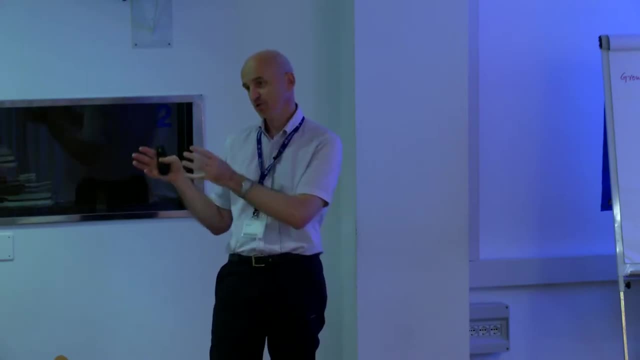 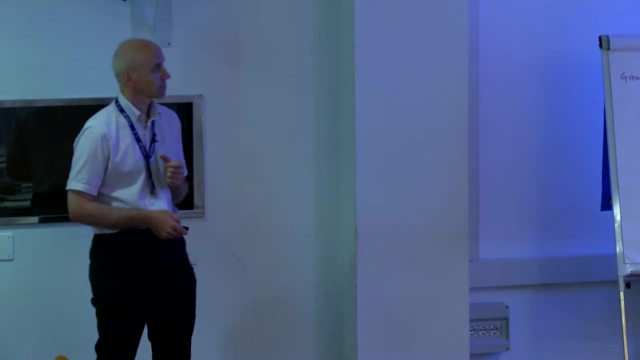 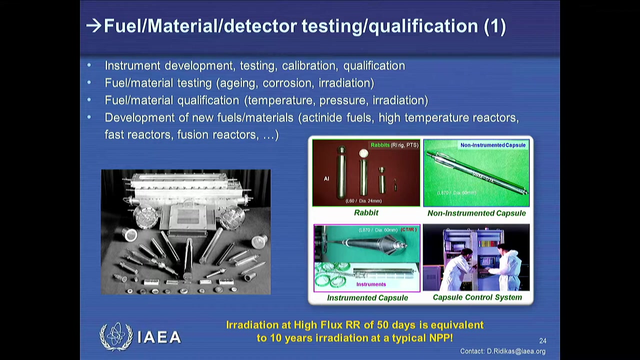 to make colorless. so that's the first application, which brings you back to the nuclear power research reactors is a source of neutrons. nuclear power has many neutrons in the core and outside the core, so to see how these neutrons are behaving you need a lot of nuclear instrumentation. 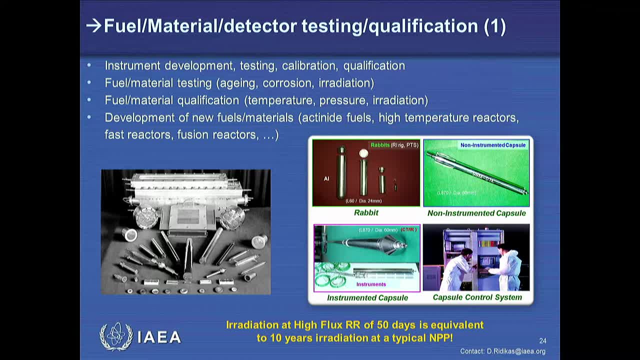 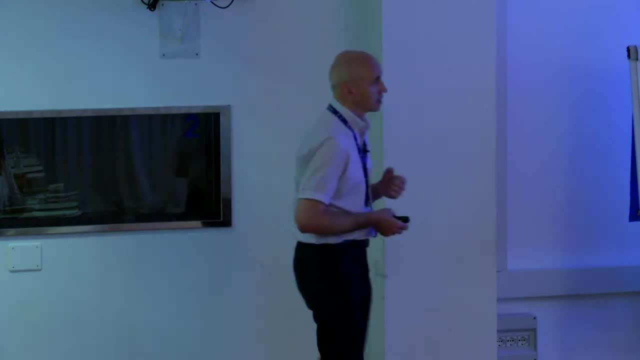 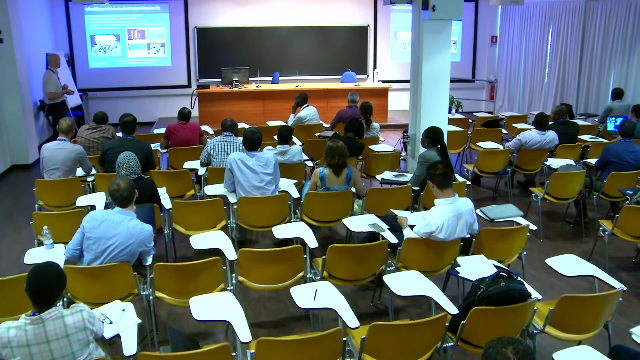 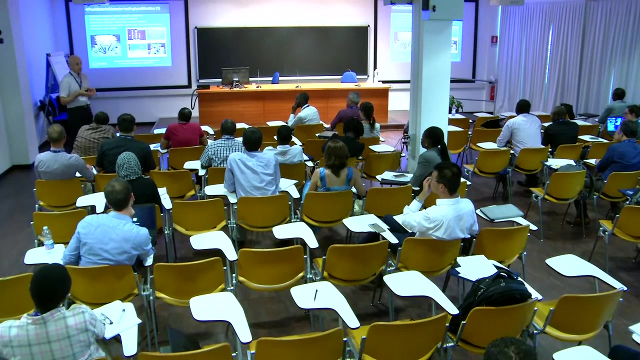 so research. reactors are a source of neutrons, so you can make a defect in a lattice of the gemstone. you can make a defect in a lattice of the gemstone. now let's talk about if you have a pure silicon by ever using akur city. power is actually a very substantial energy, energy resource. because of its sound quality. it's a deeply toxic process. this nuclear power reactor comes in key, though in nuclear power 저희가 often deal with persons also with uranium energy or nuclear power reactor. however, to use nuclear power reactor as a well defined source of neutrons can serve, develop and improve nuclear instrumentation thousands, countless hours a 씨가 for nuclear power plant. it can test and qualify various materials for nuclear power plans for one important reason that irradiation of nuclear power plants can test and qualify various materials for nuclear power plants. for one important reason that irradiation of nuclear power plants for 10 days because of high flux research reactor. 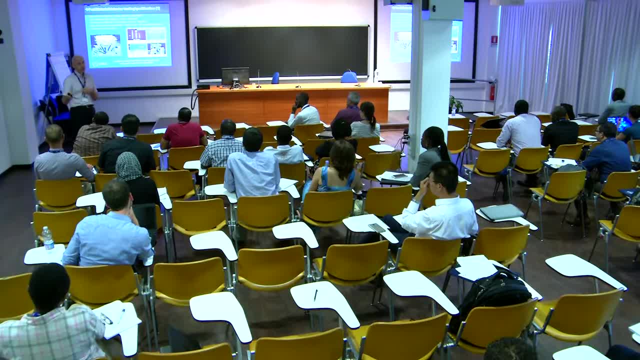 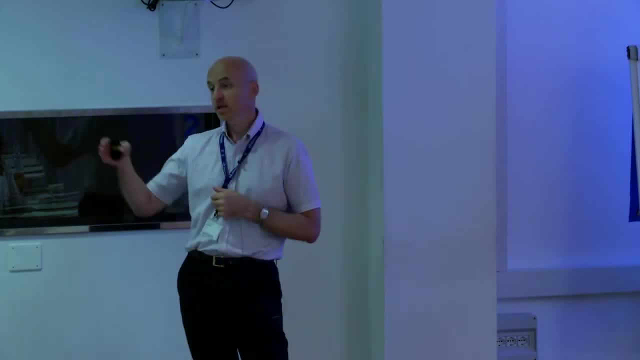 In other words, thanks to research reactor, you can predict experimentally what will happen with the structure, material or a fuel in a nuclear power plant for tens of years to come. So there is a great support in particular for the existing nuclear power plants in terms 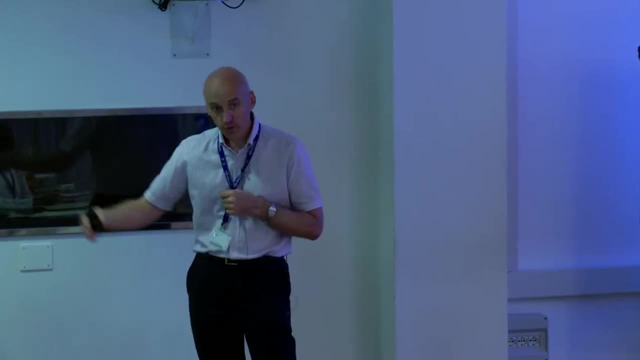 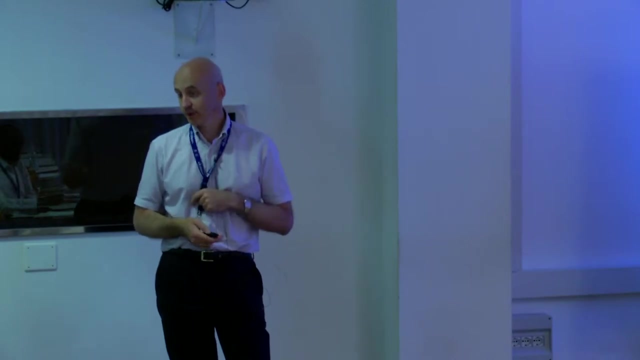 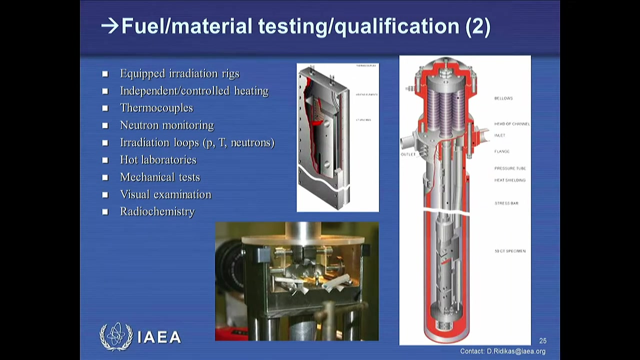 of extension life operation, but also- I will come back to that- in particular for the new generation power plant designs, because you need to test them experimentally. This is what is happening. You have dedicated what we call irradiation rigs, where you create experimentally one-to-one 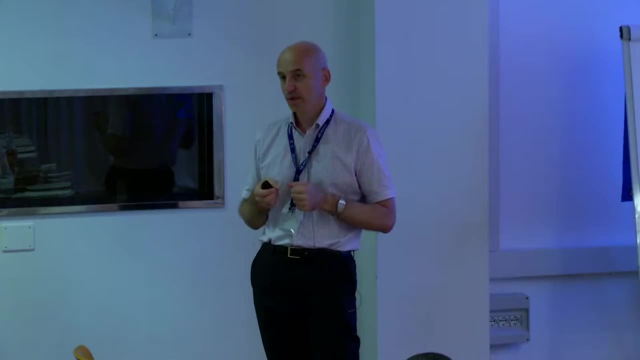 conditions occurring in a nuclear power plant in terms of coolant, in terms of pressure, in terms of temperature. So you radiate sample, It will come to you. You radiate sample In the release of the nuclear power plant. you radiate sample. 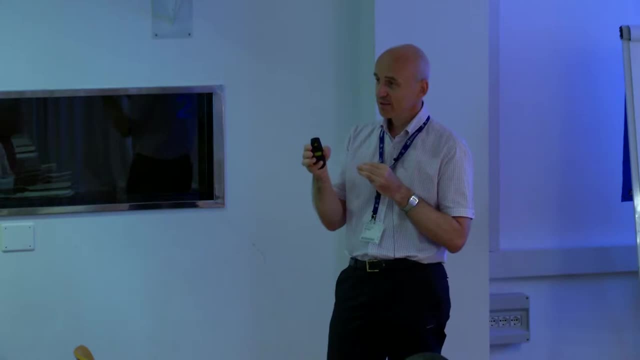 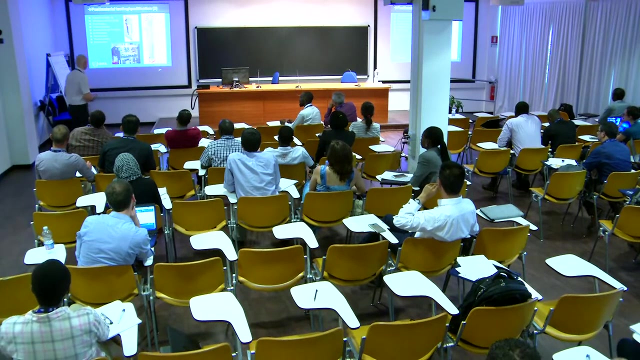 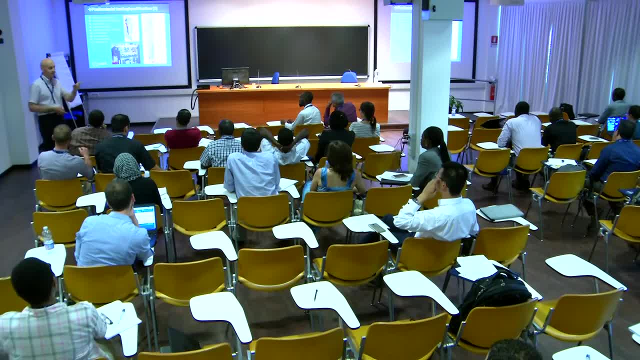 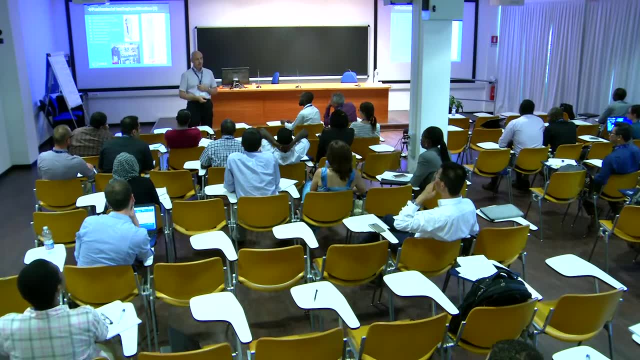 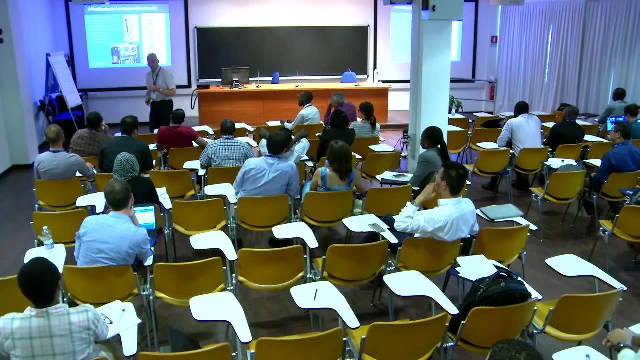 in the conditions you want it to apply? Yes, What is the time between the test and the irradiation You just said by the two words: One is for research, Another is for testing. There's no major difference. The test reactor actually comes from MTR material test reactor. 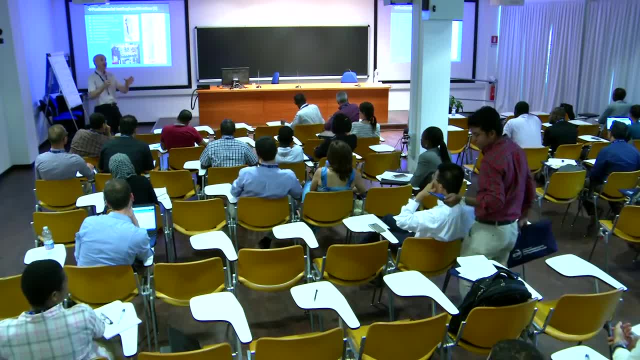 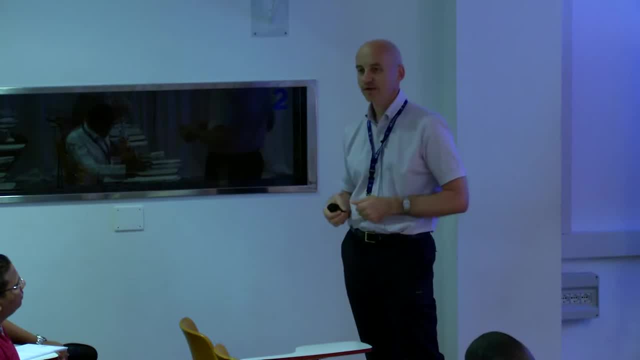 So these reactors have dedicated purpose And, design-wise, these are high-flux machines, sufficiently high to make a difference once you radiate the material. But these are also research, because you're researching about materials, So there is no main difference, Okay. 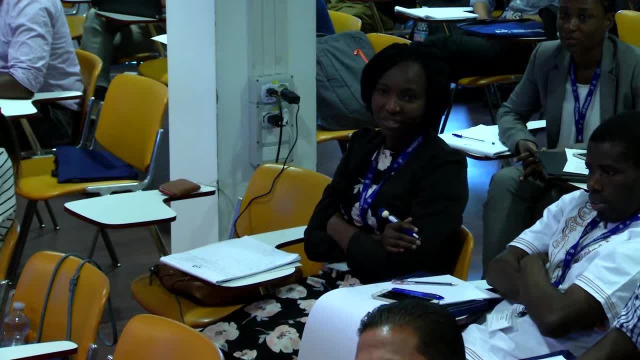 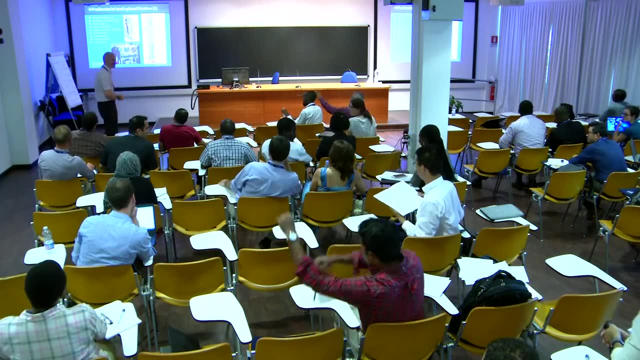 Just different definitions. Okay, That was the question. No, There were two questions. Yes, You know the pressure is a very important parameter. Yes, Yes, How you can deal with that Here in research, it's very important. 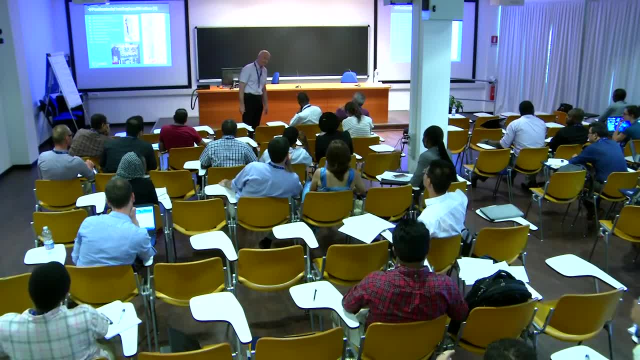 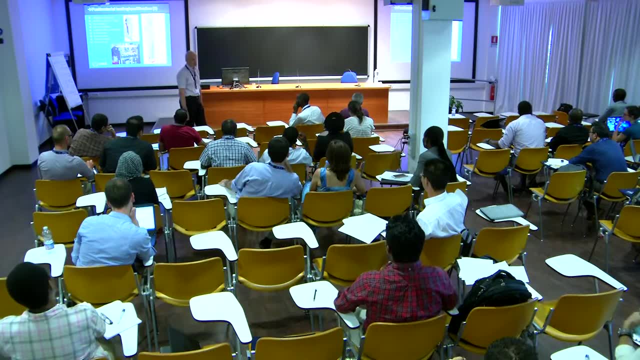 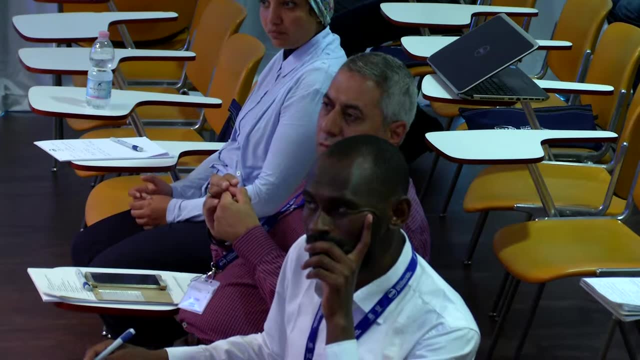 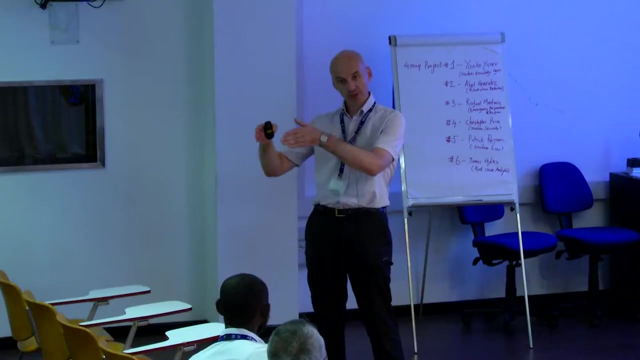 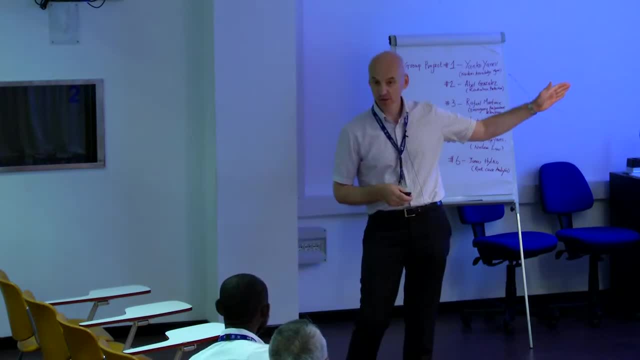 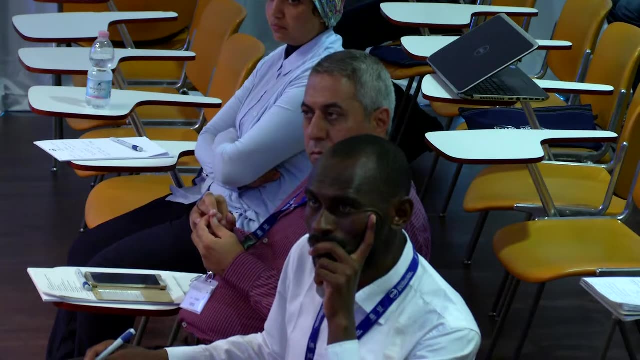 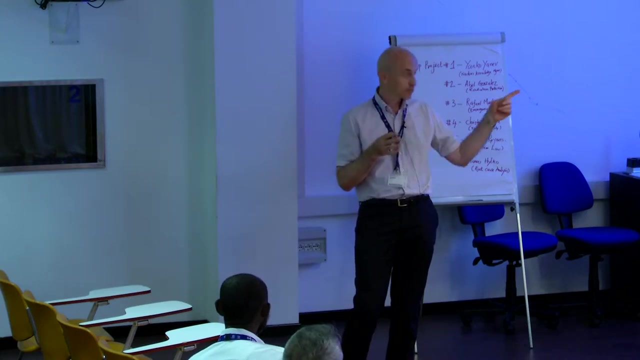 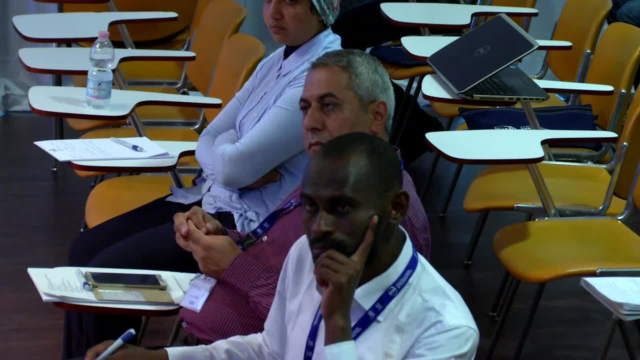 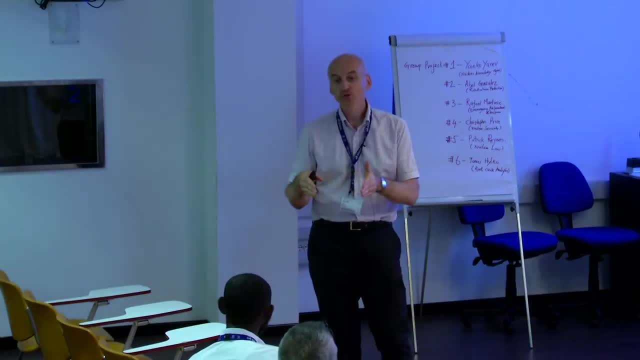 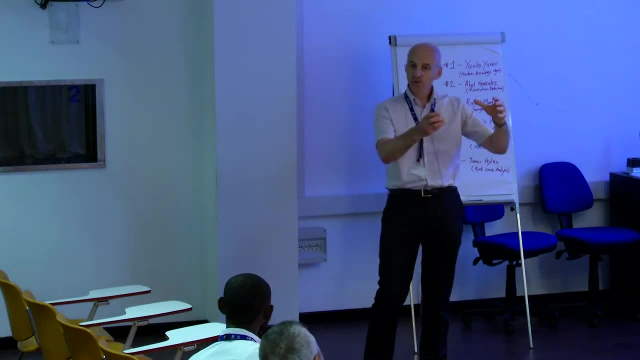 future generations. And in this way I create exactly the conditions, monitoring pressure online and temperature online to make sure that during the radiation process it corresponds to the realistic environment. So this device comes to the core of a research reactor as close as possible to reach desired flux levels for 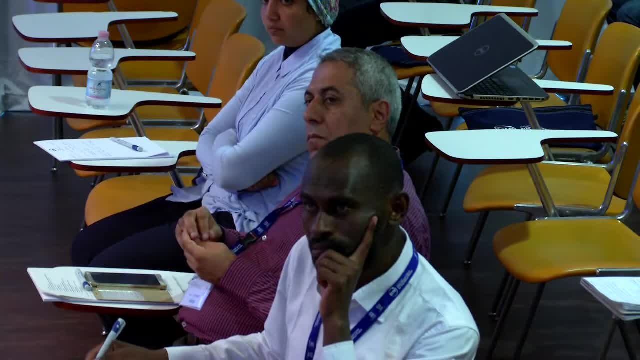 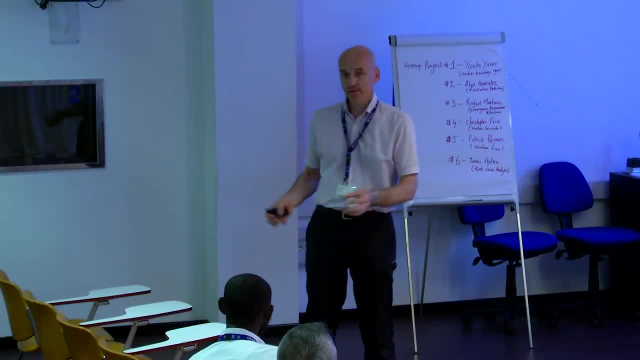 radiation purposes. And then you extract that and do different tests and examination- we call PI, post-irradiation experiments- to see the real material, either using chemistry, mechanics or different approaches or other analytical techniques to see what has happened with the. 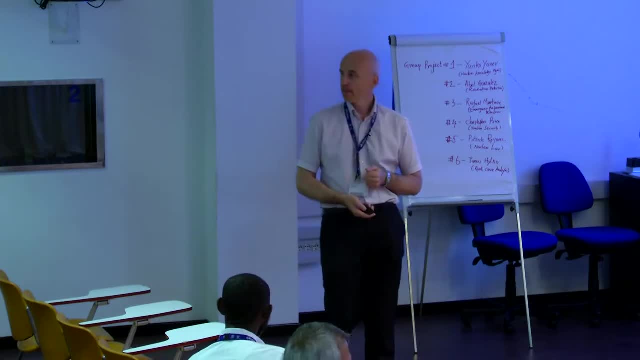 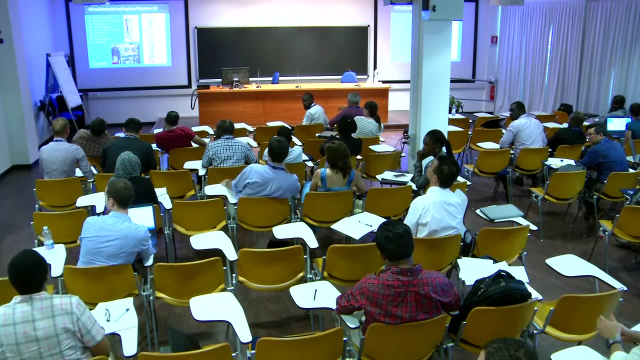 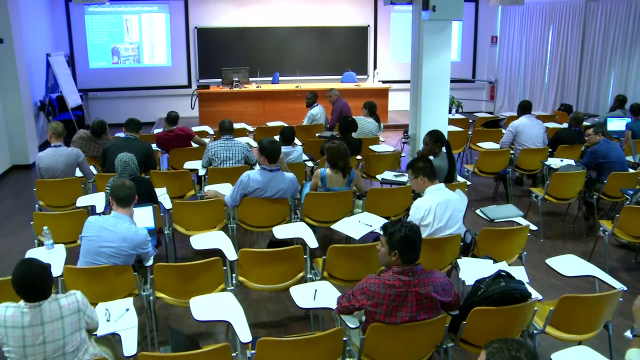 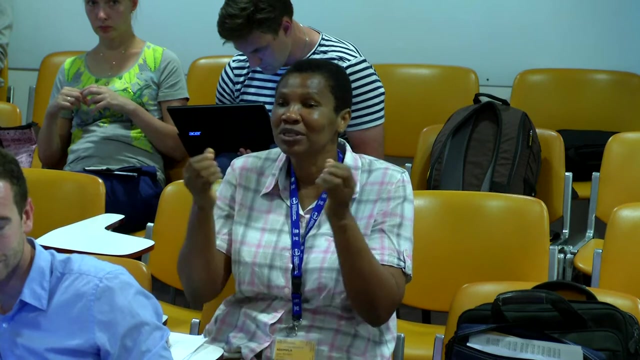 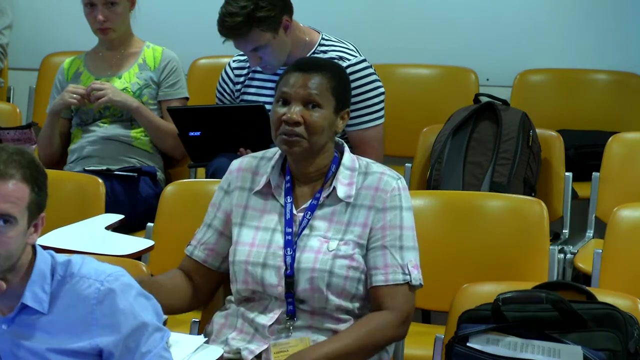 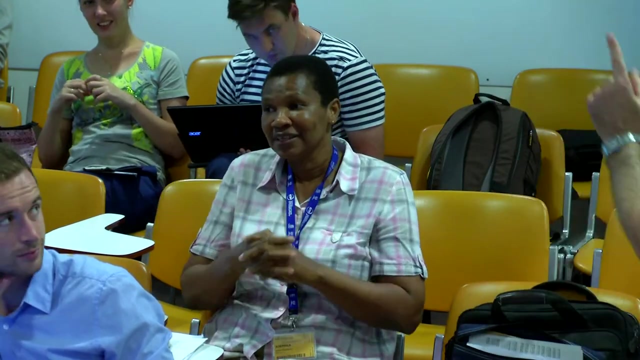 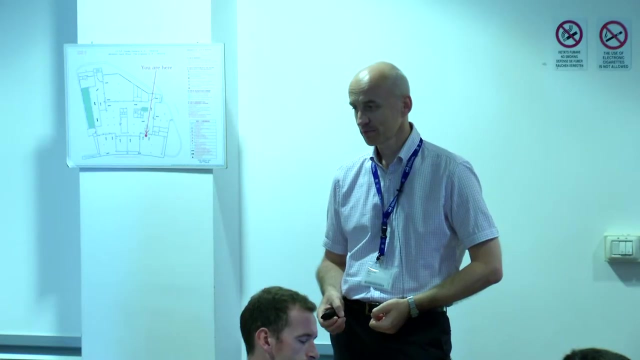 material during radiation. Yes, Yes, as long as you get money. yes, Not my. No. Now there is ethic part of it. right, You're using something natural. you're consuming natural resource- gold- which is always limited. 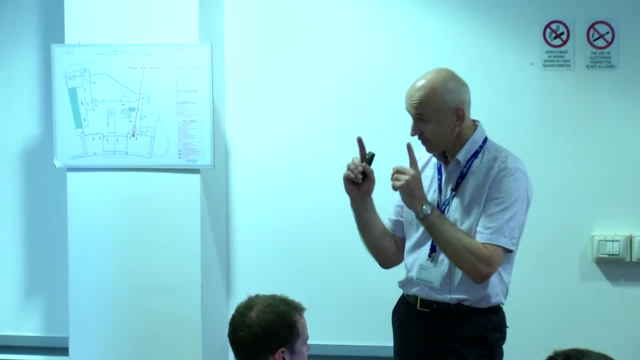 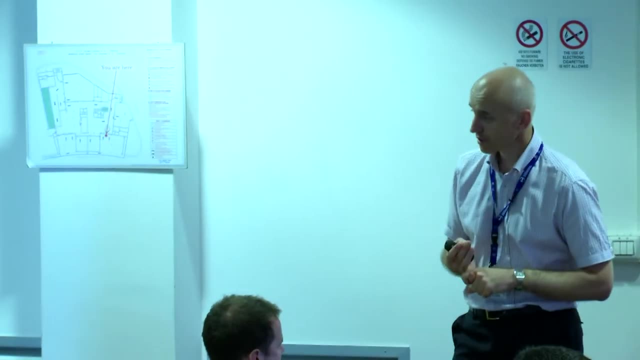 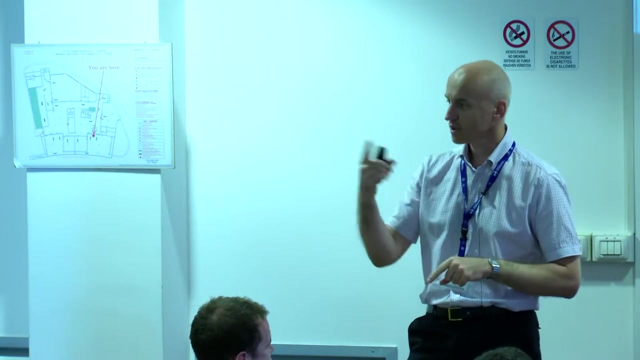 This is the way to create something which is nice, if acceptable, and you replace it And somebody makes a lot of money off that. Now, in European Union, this is forbidden. You can produce, You can commercialize. That's outside of European Union. 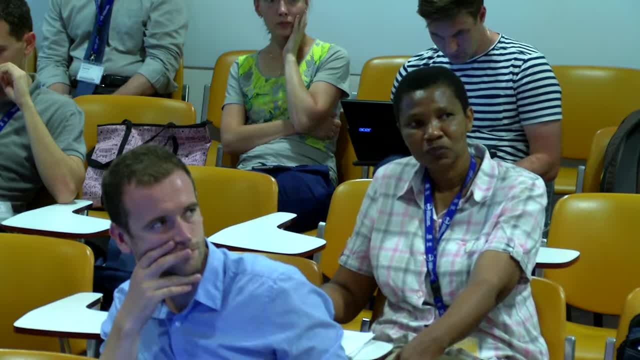 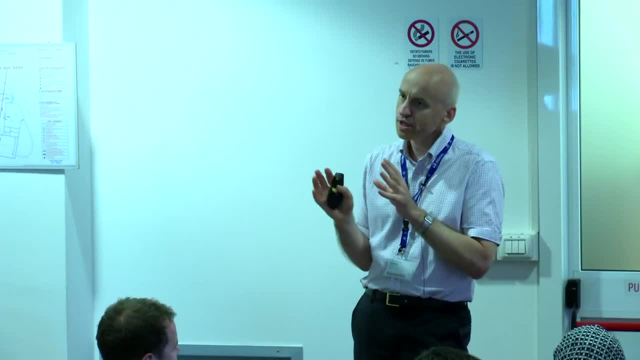 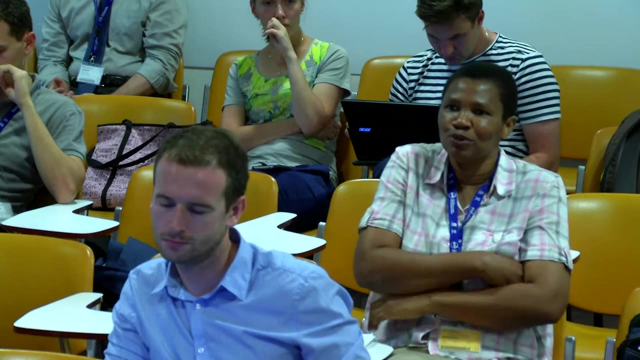 So this is: the politicians decided we're not going to make jewelry through irradiation process and that's it. Yeah, I don't call it justification, I would call it acceptance and policy. Yeah, I call it justification because you must. 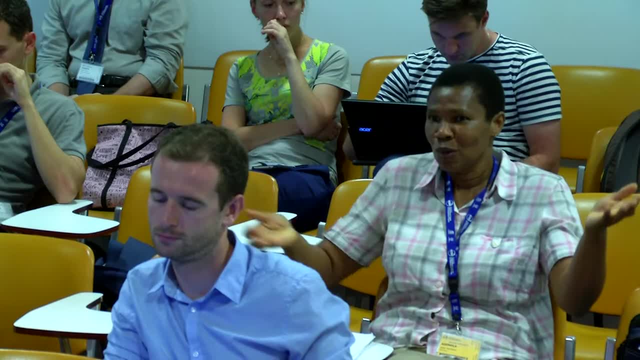 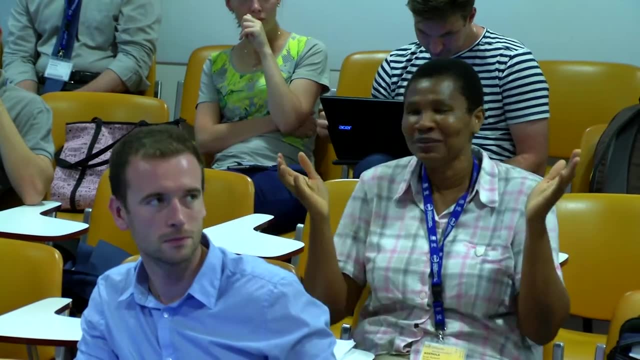 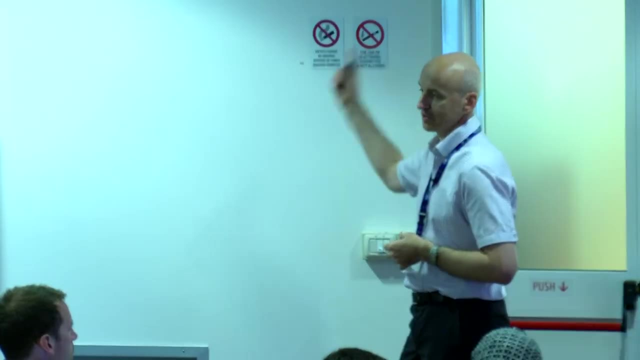 risk the benefits You must benefit just to put a necklace on your neck and you don't want to lose it. Let me put it differently. When you build a house, build a house, do you keep natural colors or you paint something on the top? 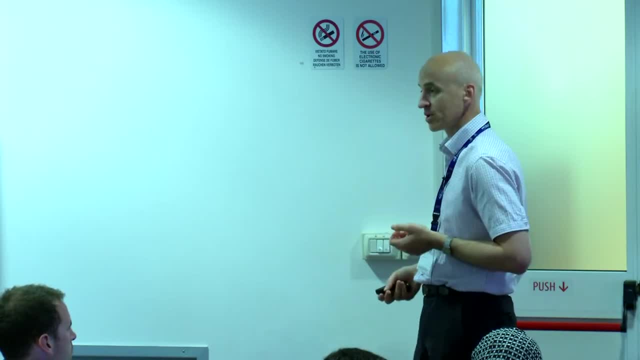 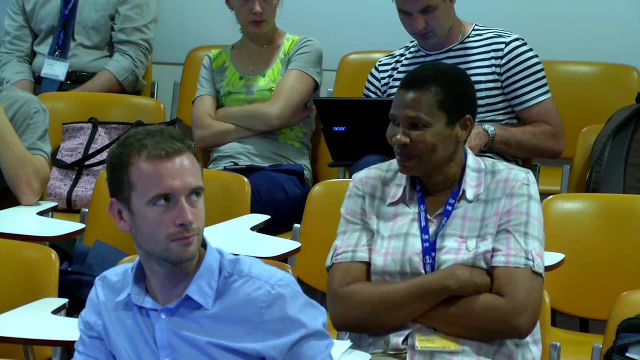 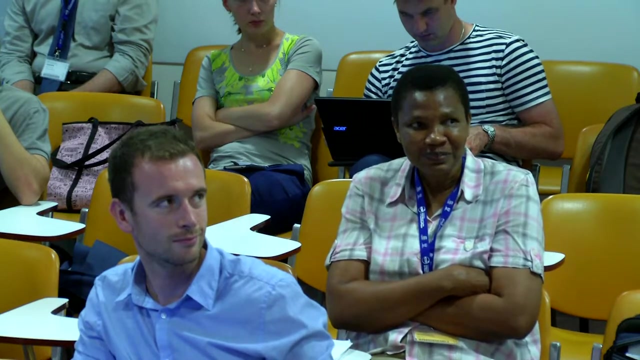 What's different? Because I like yellow, So I'll put something. Is it justified for my taste Or is that harming you? No, it's not harming you. this one, The irradiation paint, is not harming you. All chemistry behind and accidents in the chemistry. 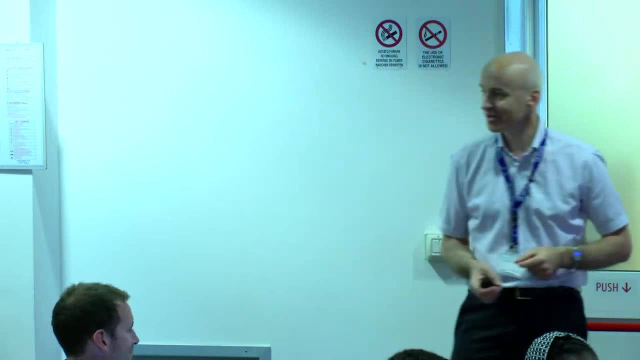 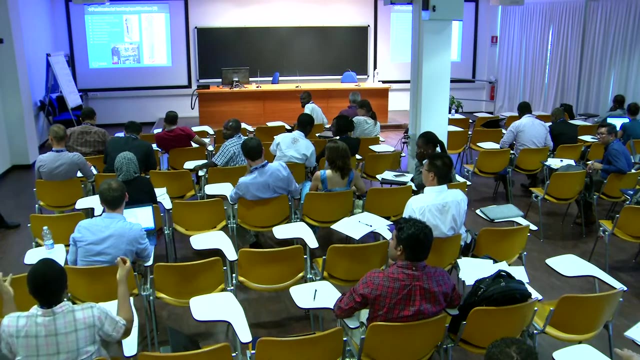 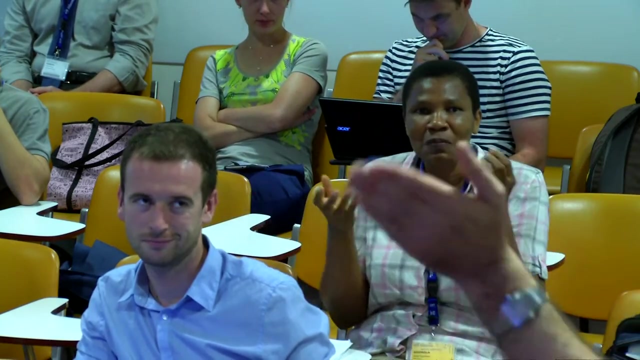 plant are not harming you. We can have long discussion, But this is well monitored, Because if you can use other methods to make it to shine- and You can use- Why then use irradiation For this stone? you cannot use another method. 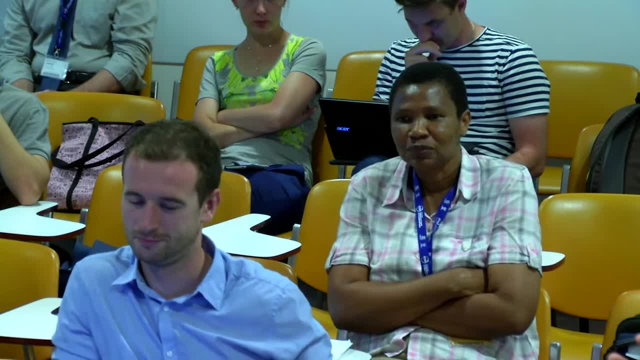 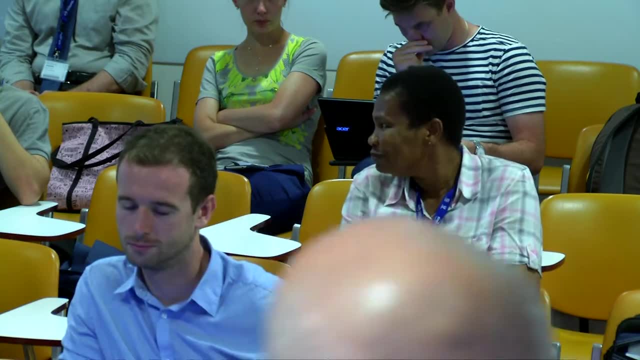 There is no another method, either neutron irradiation or gamma irradiation, for this stone which has no value, but after irradiation has a value. So this is what we call add value. Add value by irradiation. Yes, Of course. 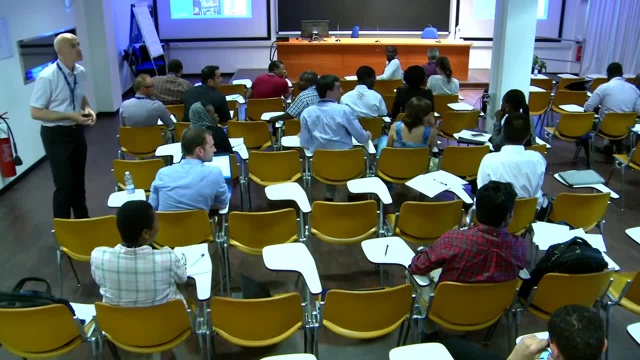 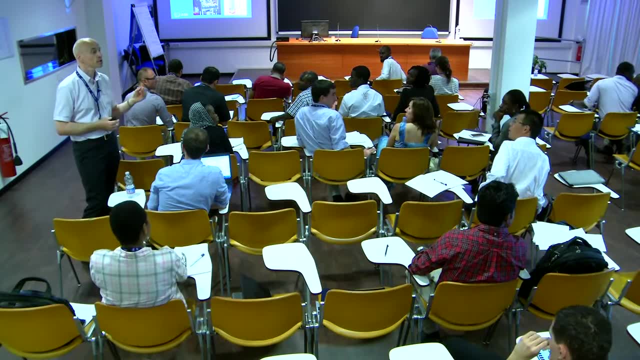 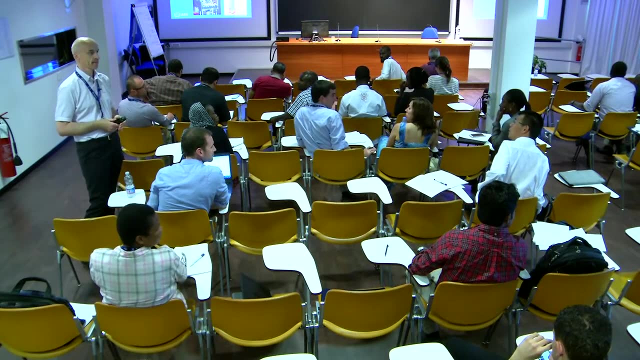 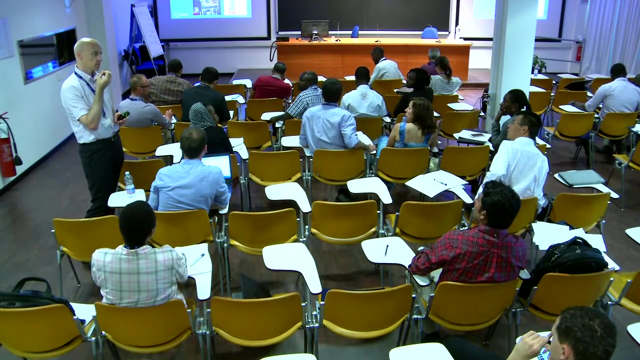 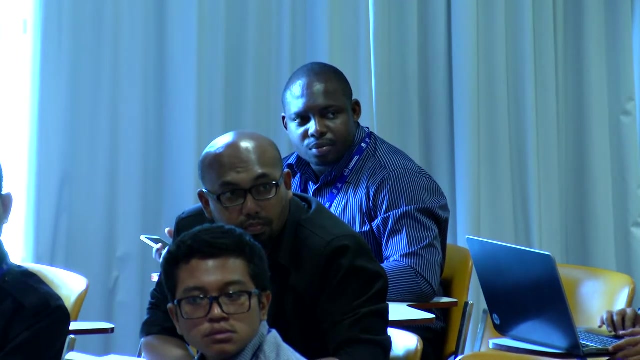 Even before coloring. it's radioactive, It's radioactive, Everything is radioactive. Yes, Yes, There is very strong. 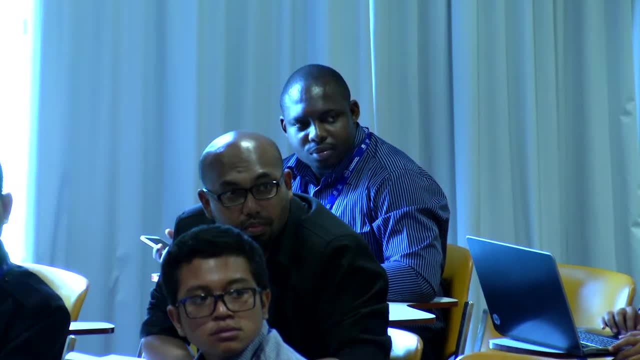 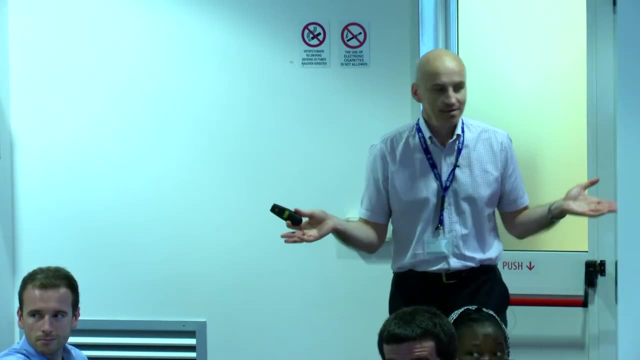 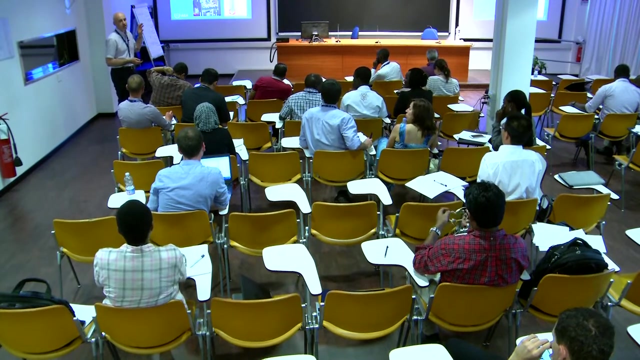 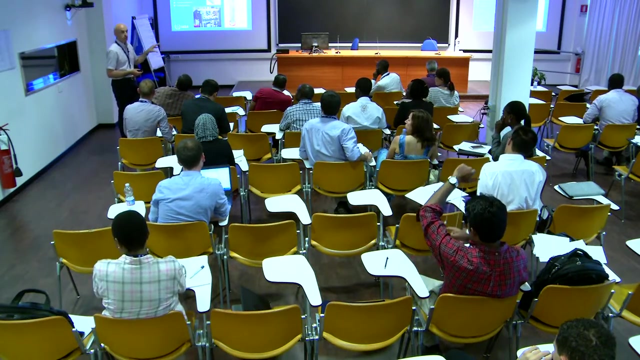 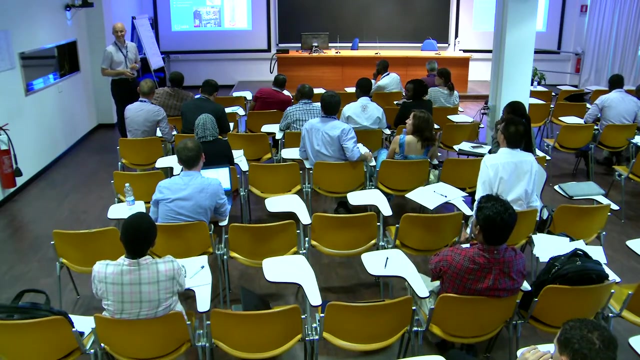 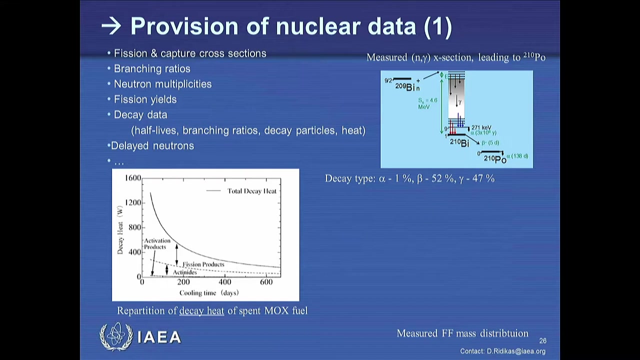 And it's very important that no long-lived radioisotopes are created. so everything decays and you keep only nice color. I share your opinion, but I have to be neutral. 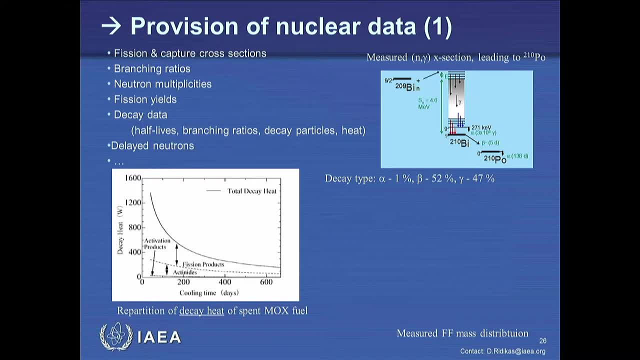 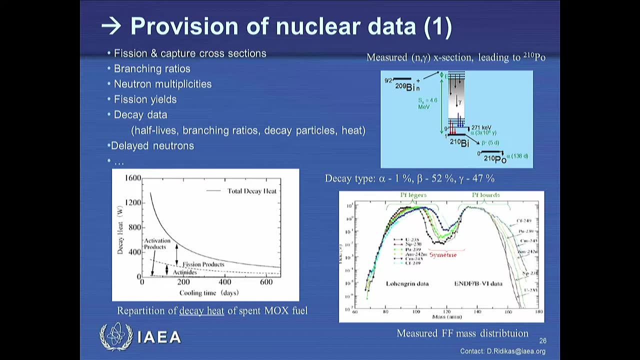 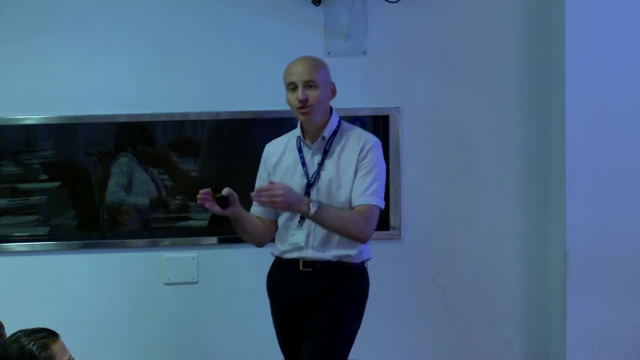 Oh, you share your opinion. Okay, Right, To understand reactor physics, you need to learn about basic interaction, And nuclear data is extremely important when you go through the optimization process, because your calculation is as good as experiments were good in supporting your prediction. yeah, 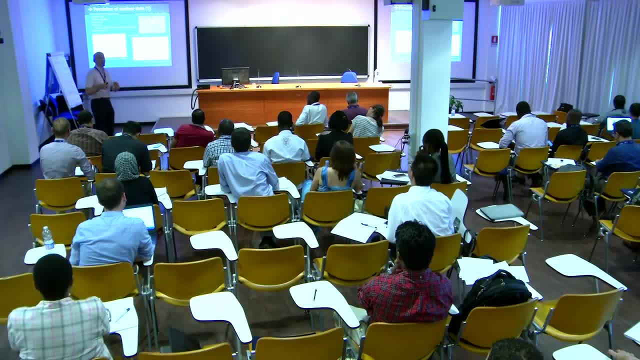 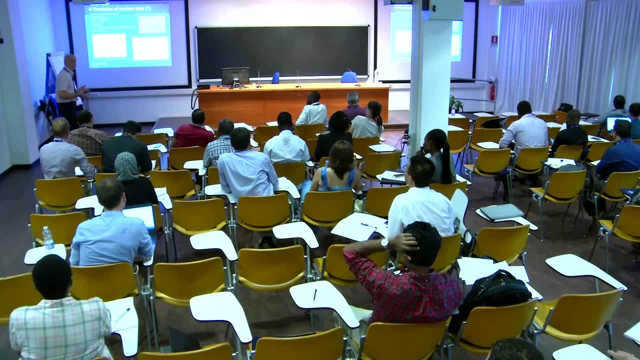 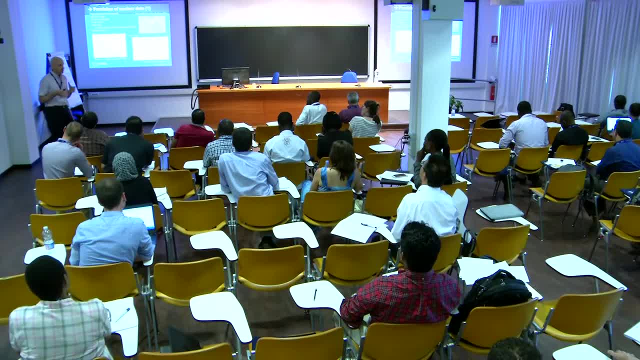 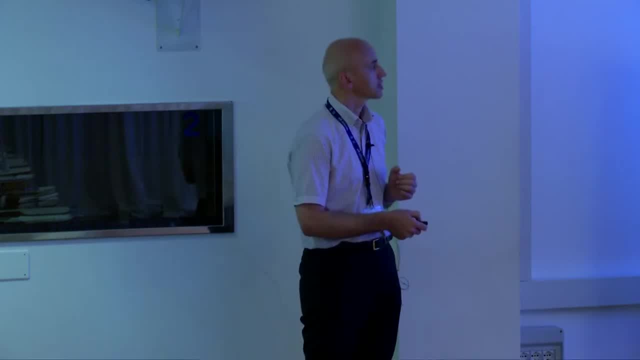 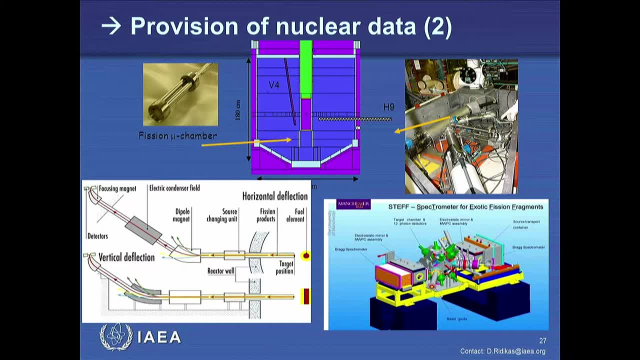 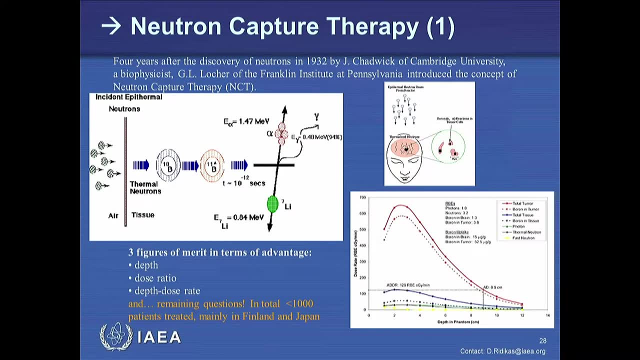 gamma, beta or alpha spectrometry and you can actually measure these important fundamental quantities as part of your research project. The neutrons have been tried to treat the patient And the process is simple. This is called neutron capture therapy, So actually you do not treat the patient directly with neutrons. 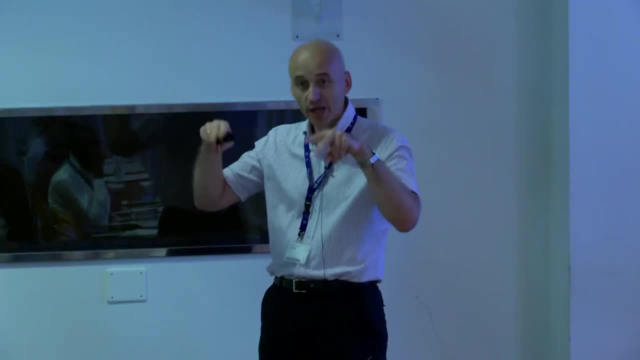 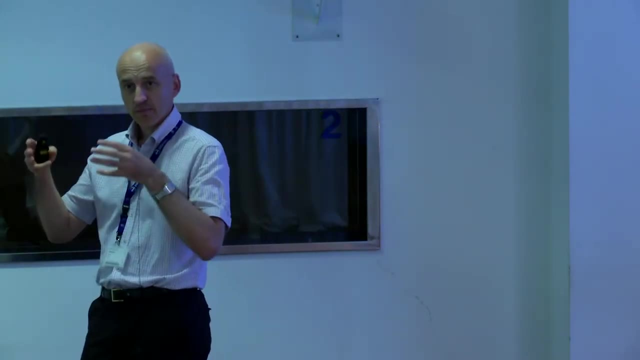 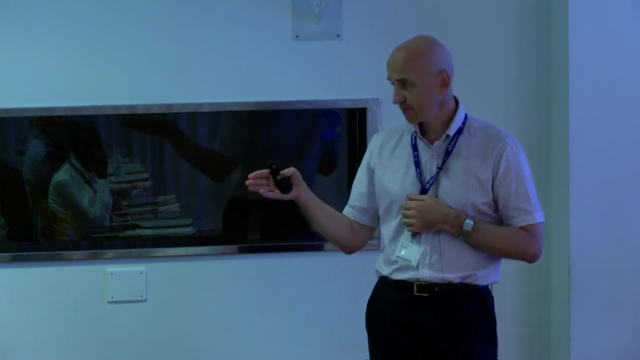 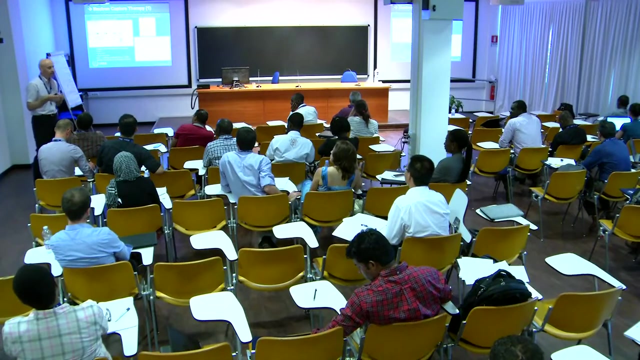 As long as the tumor has been identified- and this is a right tumor for this particular treatment- you inject boron concentrated material into your tumor cell. Now, when the neutron goes through the body, this is also not a good approach, right, When the neutron goes through the body, in most of the instances it will not interact. 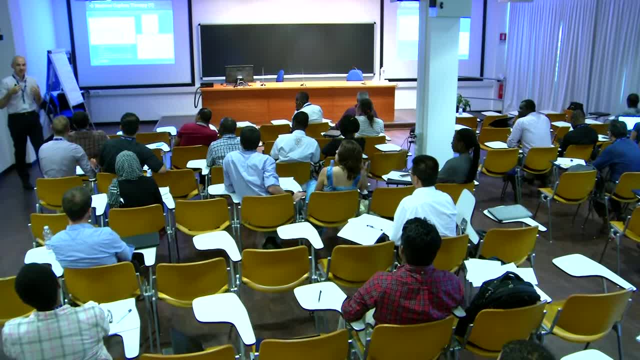 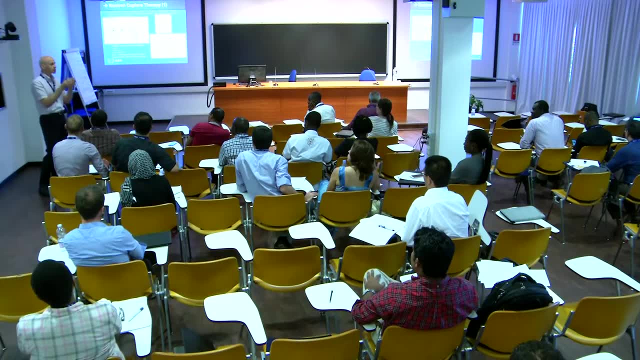 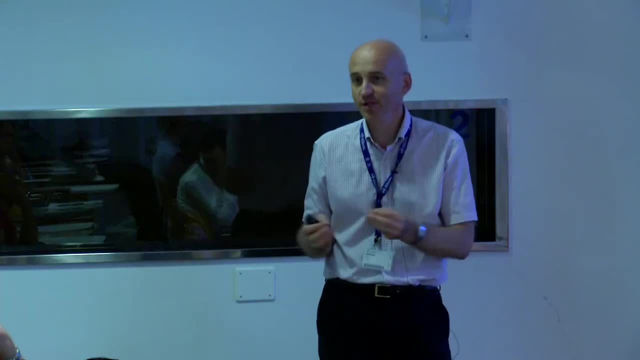 or not sufficiently interact with the normal tissue, But as long as it meets the boron, it makes a reaction and alpha particle is emitted which burns locally the cancerous cell. So the physics is a bit I don't know. for some of you very simple. 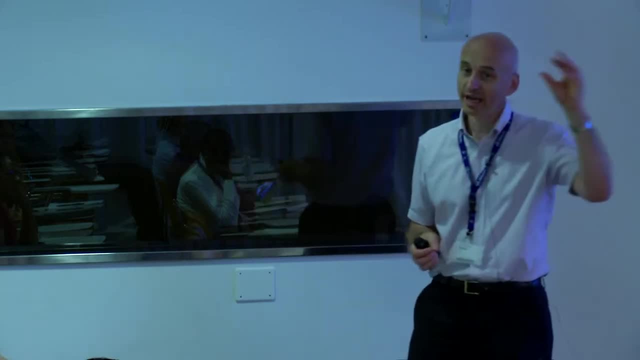 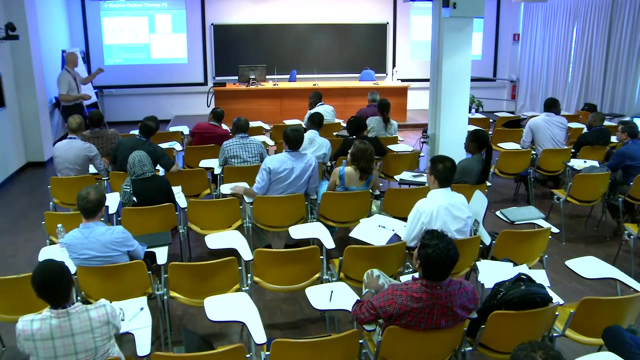 For some of you it might be complicated, But the point is it's not neutron directly interacting with the cancer cell, But it goes through the transfer of one particle to another. Now how it is done, you see, you localize, and this is typically. 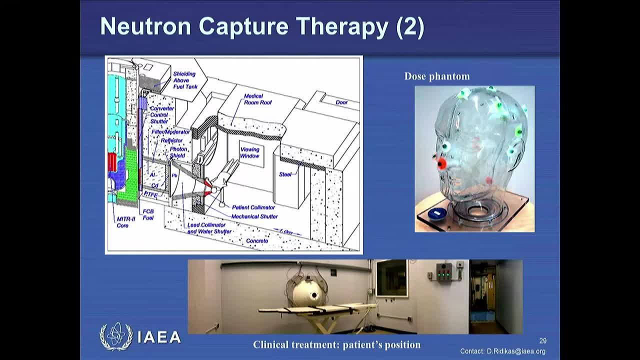 A lot of work needs to be done before by irradiating those phantoms, because you need to calculate the neutron energy and dose the patient would receive during the irradiation process. Then you define the time intensity position your patient at the reactor through the collimated 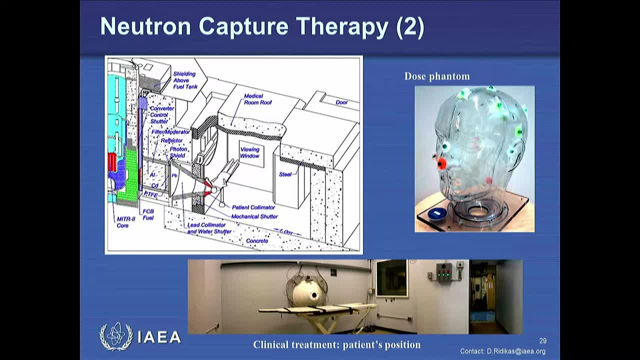 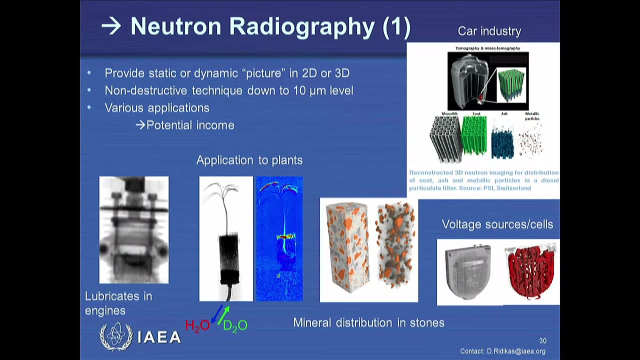 beam And you do the irradiation with the presence of a medical doctor. okay, Some pictures. yeah, Less words and some pictures. Radiography is one of ways to attract many different users to research reactors, because it can provide 2D and 3D picture in non-destructive way. 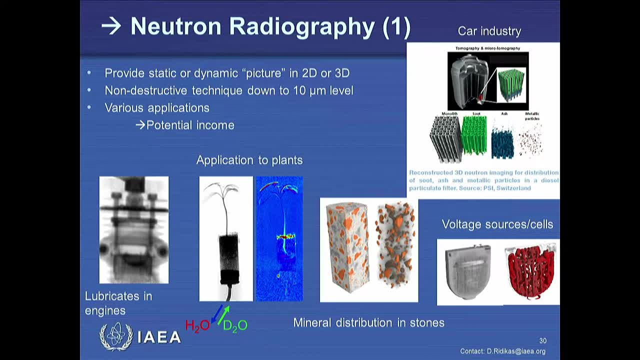 And you can go down to the micro level in terms of resolution. So you cannot see atoms- Not yet with this technology- But you can see very fine structure, what is inside. This is typical image. 3D reconstruction image of diesel motor filter in the car industry. 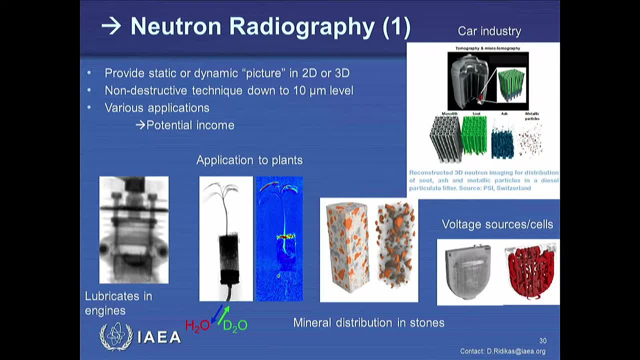 where you clearly see how metallic particles are distributed within the filter. It's very important for car industry in terms of efficiency to see how filter works and how it captures metallic particles. You can study source cells In the material construction. you can see how the stones are distributed inside with. 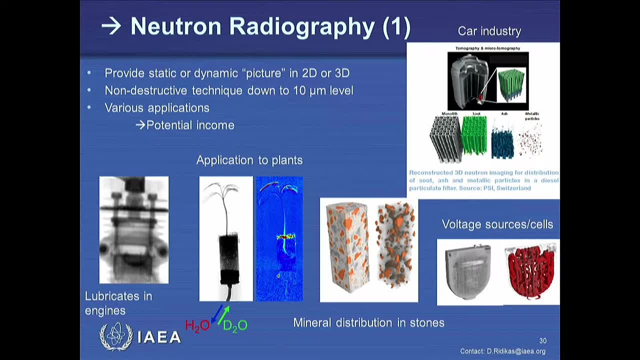 very powerful technique for anybody who is involved in the construction and cement in particular. You can study plants. You can study how plant takes the water, And this is- you see the image how the water is distributed as the time goes. as long as 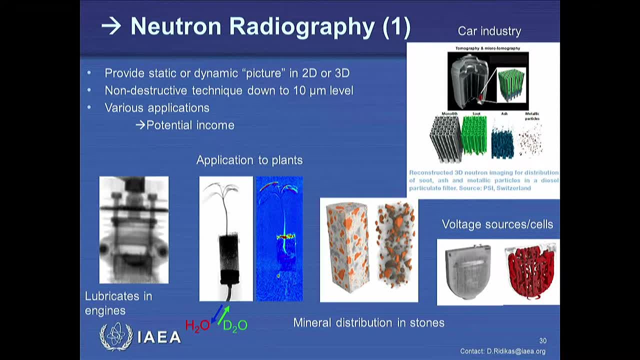 the flower was watered Through dynamic. Through dynamic imaging, you can see how the engine works and how different parts of engine receive the oil from the source, because it needs all the time to move smoothly. And that also can be done by neutron imaging. 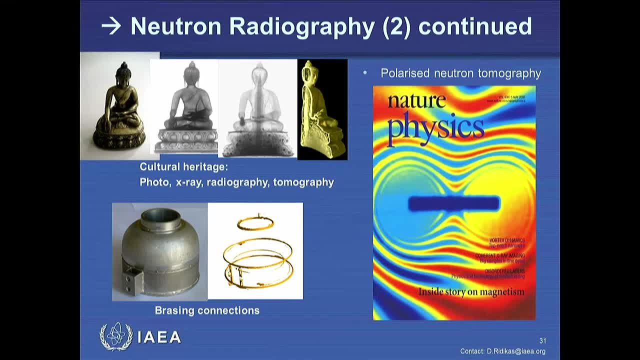 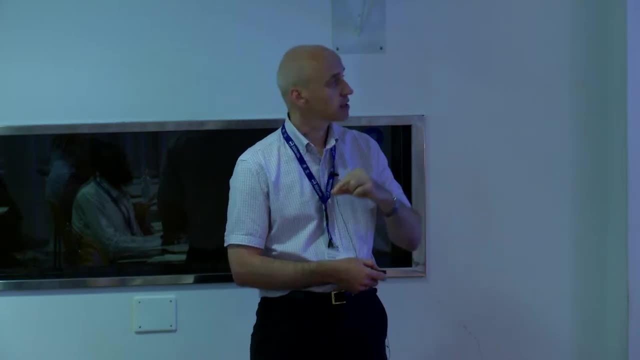 You can apply that to cultural heritage. This is an example to see how neutron tomography gives more information compared to typical X-ray tomography, For example an X-ray image. Because of the thickness of the material, The neutron can penetrate deep. 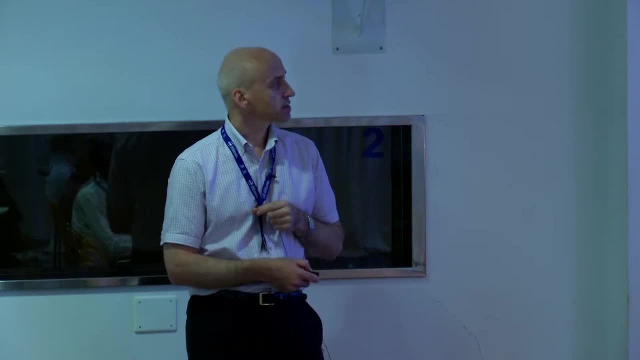 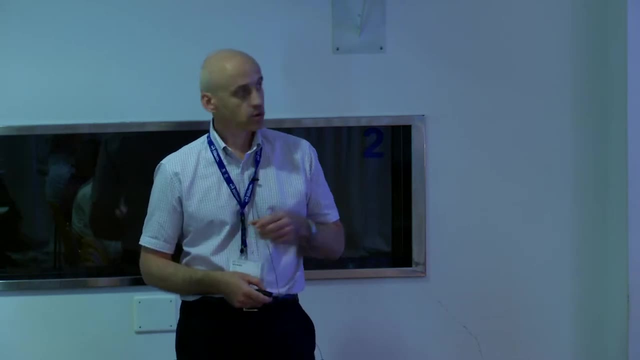 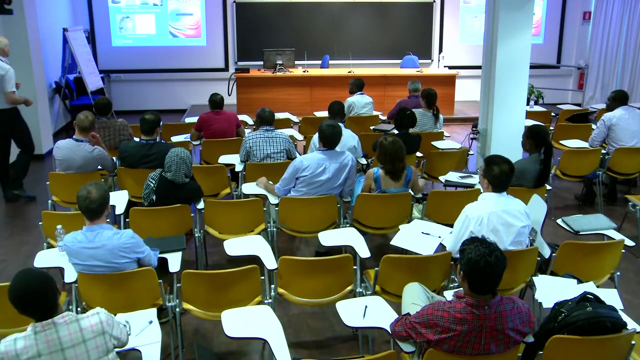 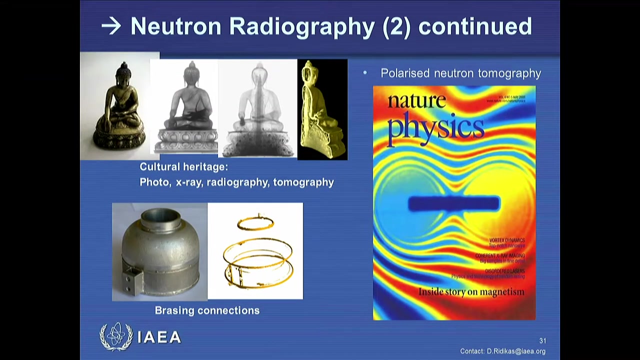 This central part was not visible, Neither these interesting structures inside of the Buddha statue. So you would never learn it unless you break it. But who allows you to break cultural heritage object? You can use that also for quality control, quality assurance, And this is typical example where you see that the brazing connections 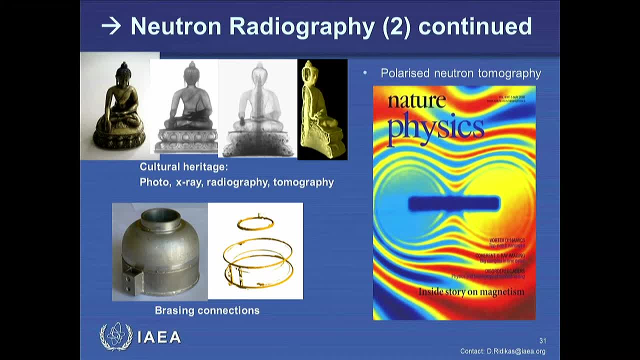 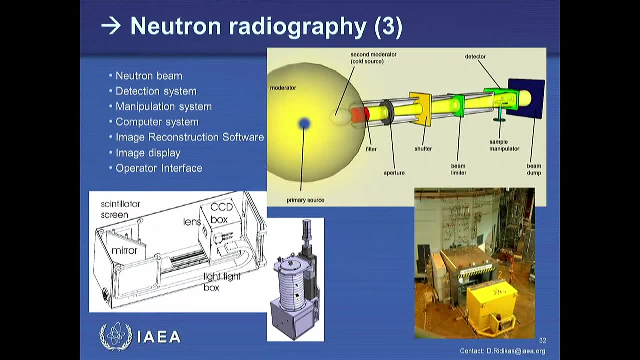 For some of it, Some of it were not done properly, You would not see it with the eye at some point How it is done. This is your research reactor. You have beam going through the shielding, You have a shutter, You place your different detectors and you perform neutron imaging of your object. 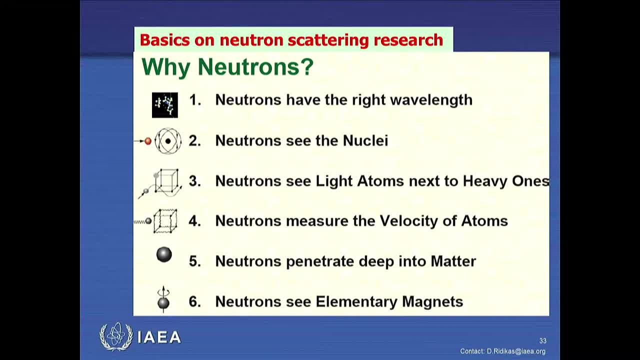 I will take another two, three questions, So that gives you a bit of waking up atmosphere Before we go on. I have a question. I have a question Because I will. being a nuclear physicist, I would like to go a bit more deeper in physics. 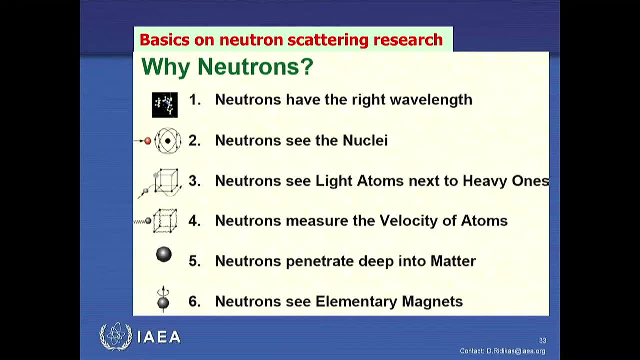 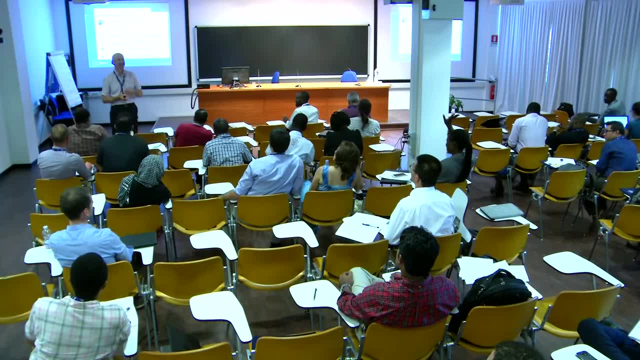 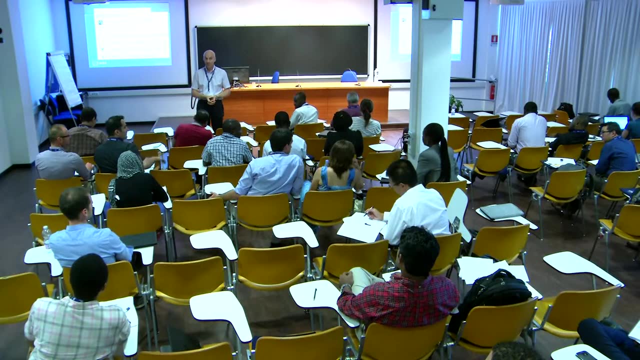 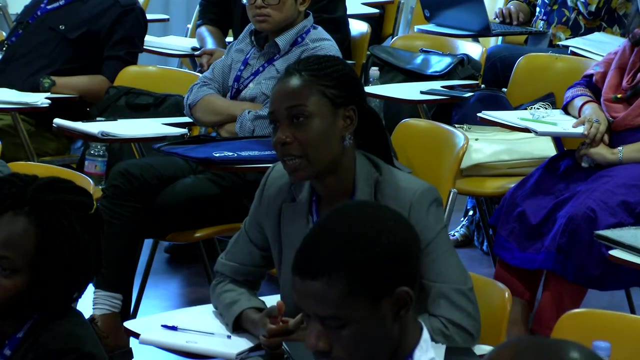 So be prepared. Any question or remark or criticism about research reactors? Yes, Do you feel? I mean, as we answered you mentioned: continue to create nuclear reactors, Correct? Do you feel nuclear reactors? Do you feel nuclear reactors? Yes, 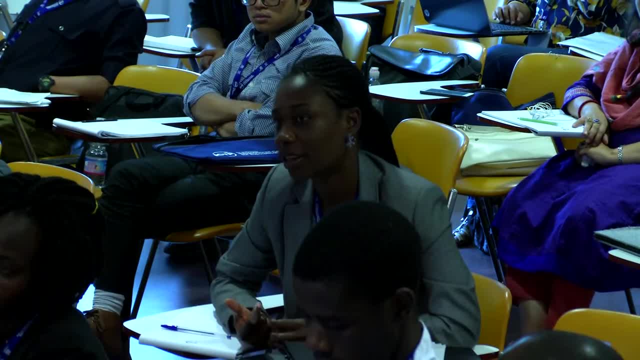 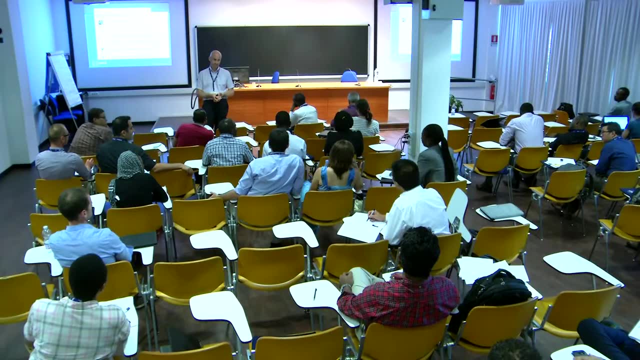 Do you know what they mean? Most of the things you're talking about are useless. You don'trealize them. Yeah, So, like you said, in Aleppo, A nuclear reactor is there, Whether nuclear Poison or jakieak share, Can this flow? 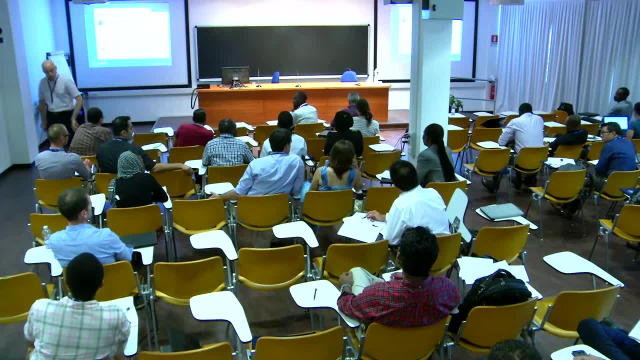 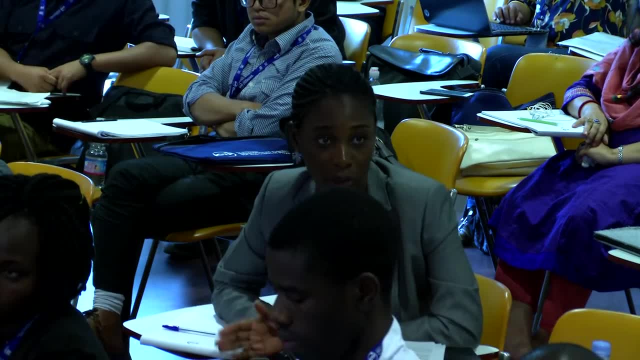 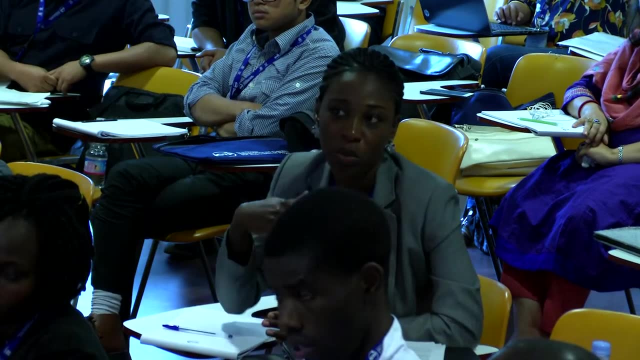 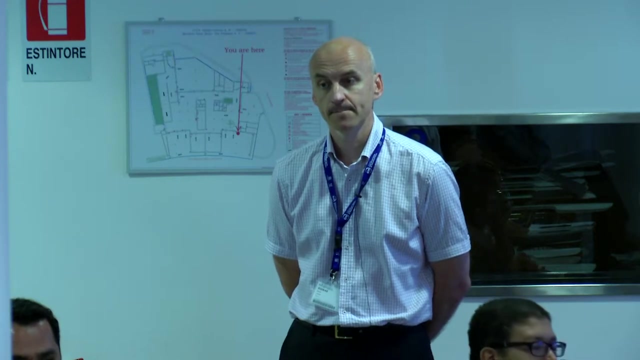 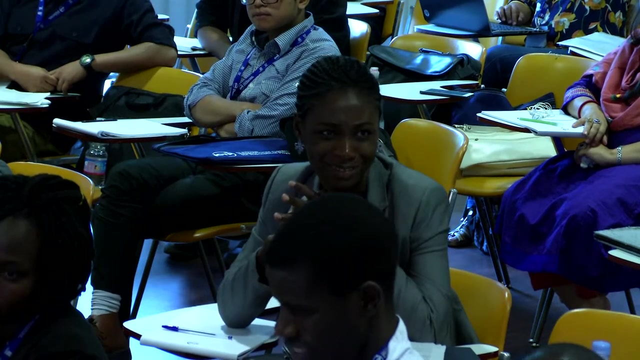 Earth as green, as black, as blue? Yes, Can it flow Or can it impression that there will be more Non-zero atomic reputations? Yes or no Care, Yes, Yeah, Okay. OK, This is here. I was okay with your question. 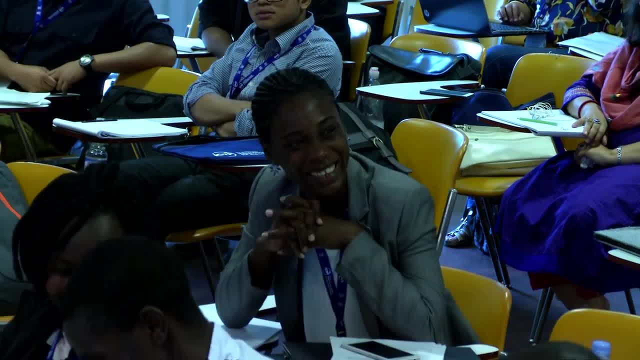 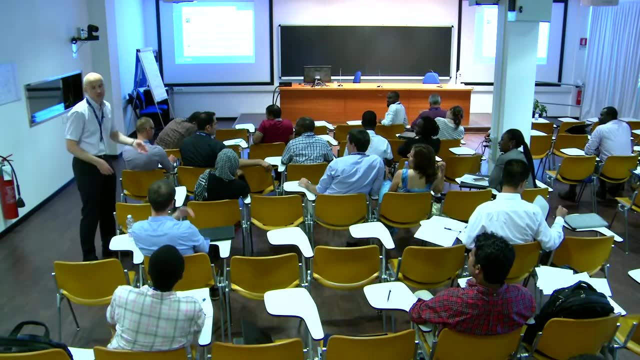 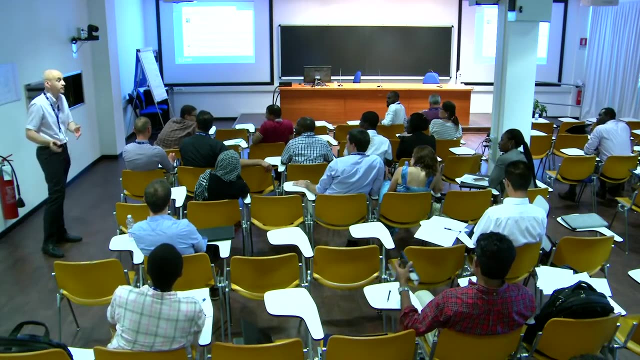 until the last two, I mean yes and no. everything is possible. there is no zero risk scenario. so this person can be trained very well at Research Reactor and later comes to NPP as a future employer and sabotage. this person could do the same without training at Research Reactor. 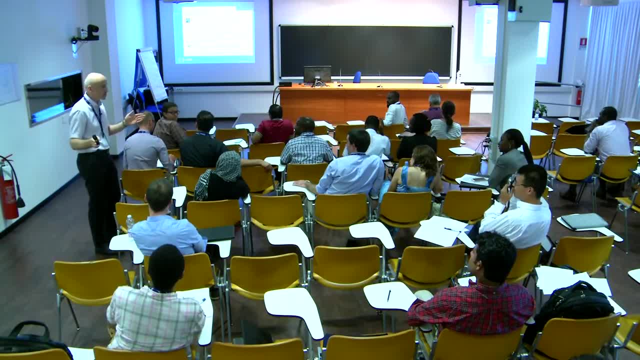 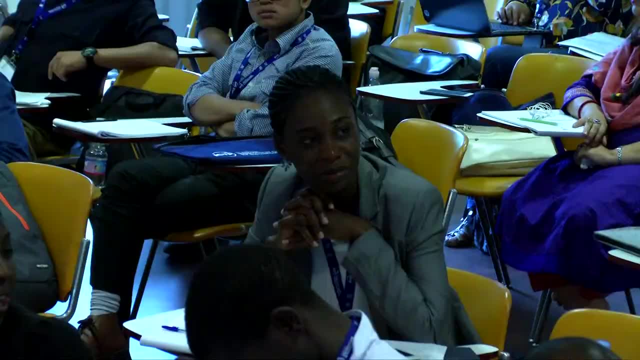 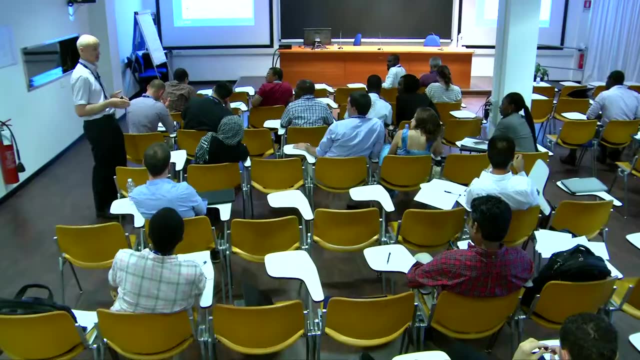 this is, I think, security people and clearances should be in place, that this person, as long as he or she works at Research Reactor, most probably will go even faster through security clearance to work at NPP because he already worked at nuclear installation and it's part of. 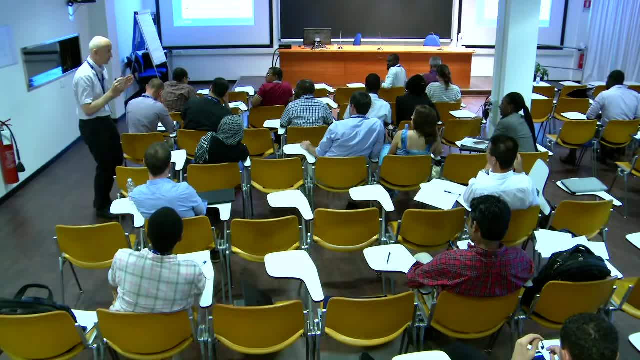 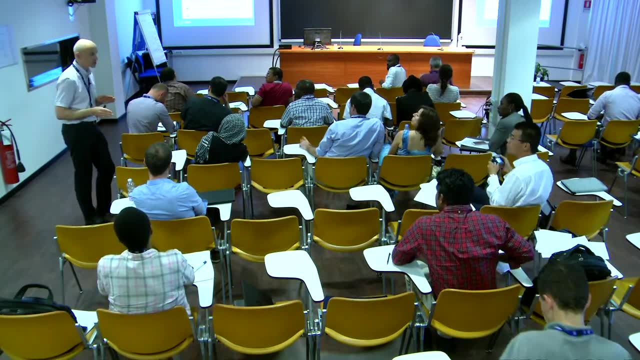 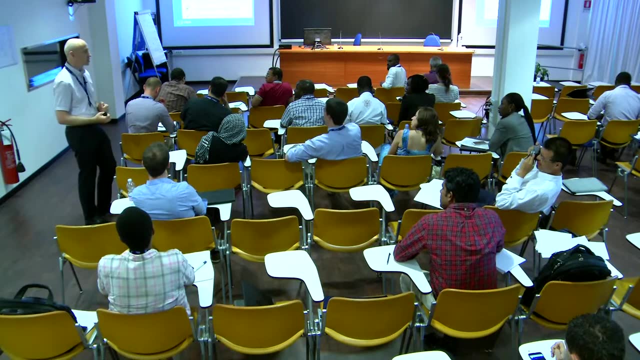 national business. now there are different scenarios. some countries say: going to nuclear power, I don't need a Research Reactor because I'm not developing technology. I'm a newcomer country, I'm bringing technology and all these people are going to be trained by the provider of NPP. 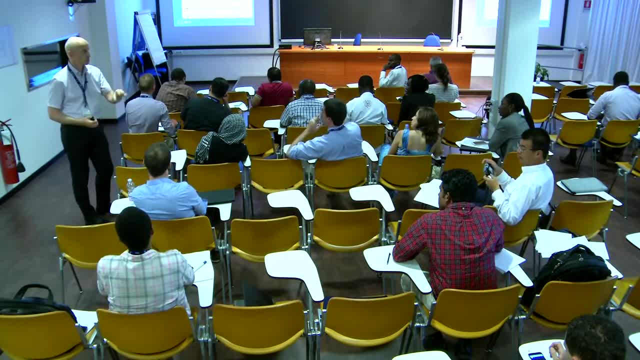 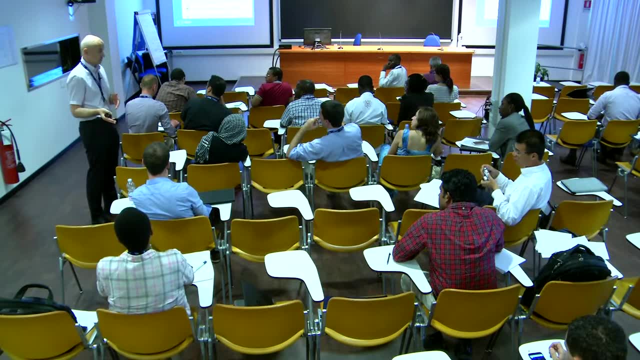 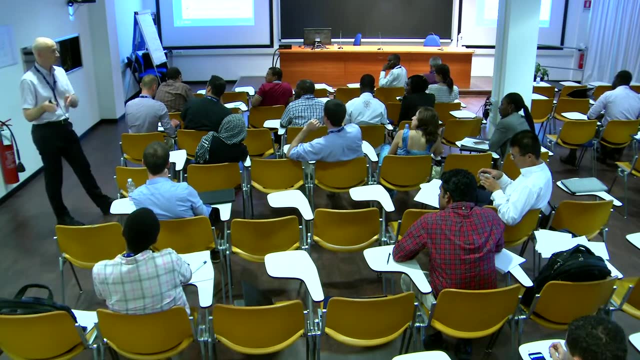 being Russian Federation, France, Korea, US, Japan, whoever provides NPP, and this is one of the scenarios. other countries already have a Research Reactor, so they see which role this Research Reactor is going to contribute to the national nuclear power program. in most of the cases, 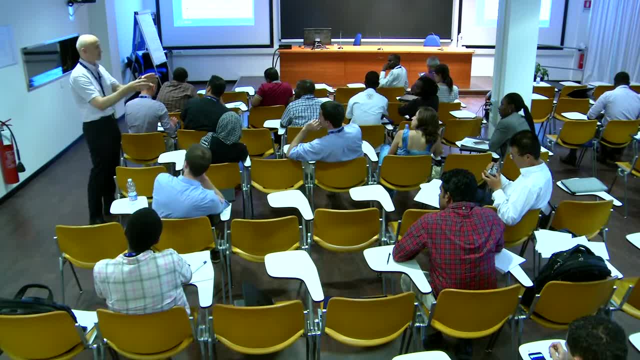 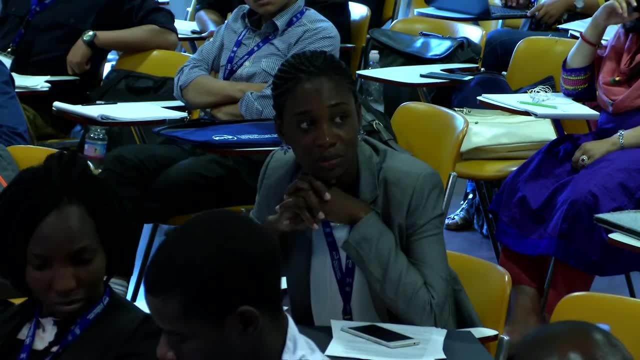 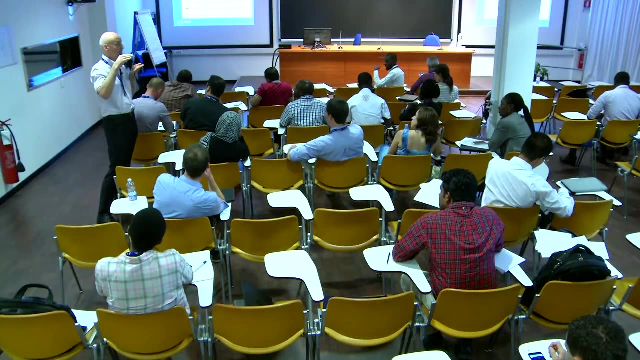 we see Research Reactor organization positioning itself as a technical support organization, because this is the only way the knowledge stays in the country in nuclear field, yeah, but if this role is not given at the desired importance, some of the organizations will be left and this service will be provided. 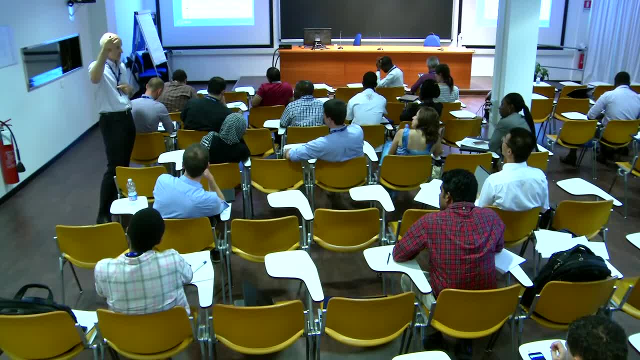 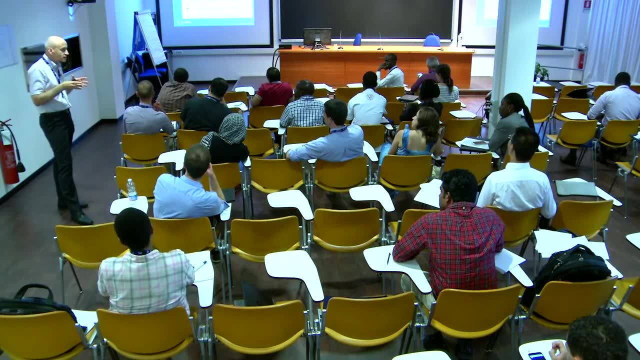 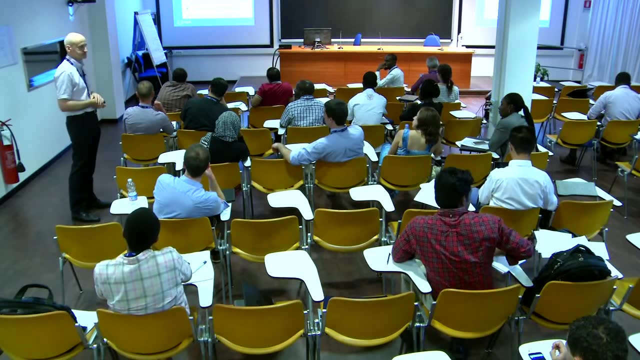 by technology provider or by the third party. so it's very much important that country decides who is doing what and if this is seen as a national asset or I go to NPP. we don't need a Research Reactor and we shut down the Research Reactor. 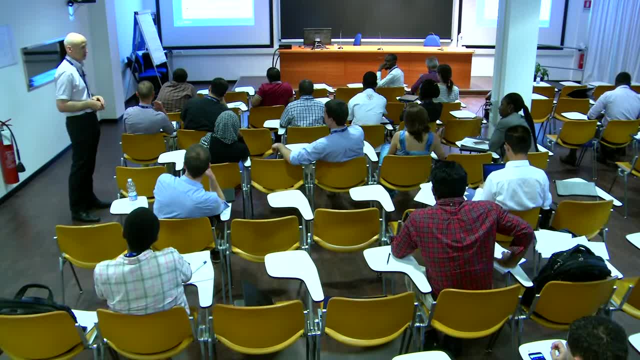 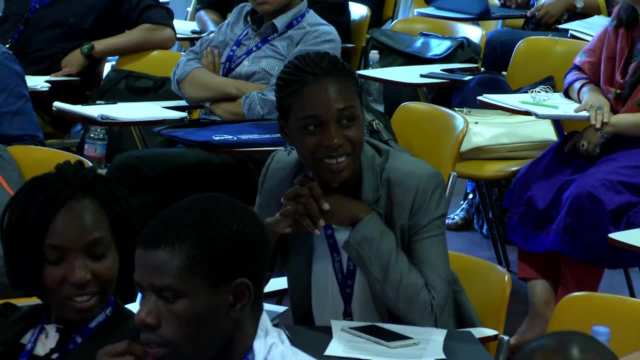 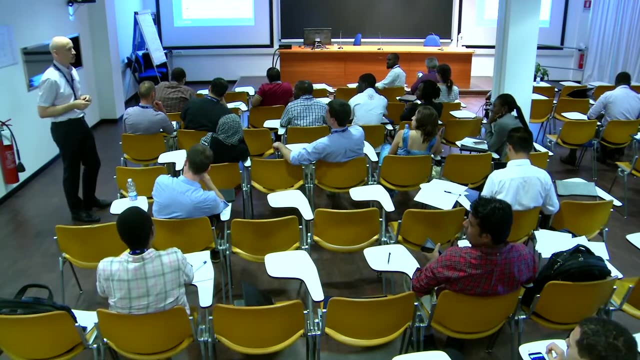 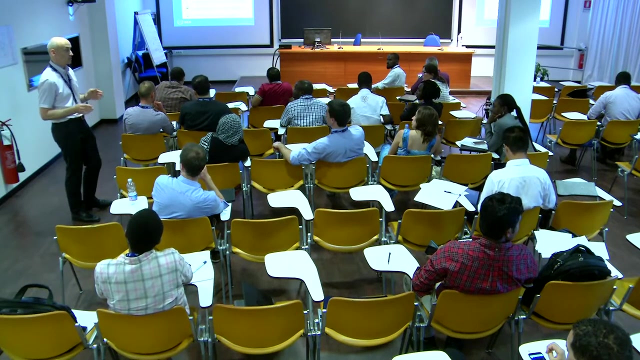 all these scenarios, except sabotage, are valid. so historically, up to now we have not seen a single country going to nuclear power without having a Research Reactor or having access to Research Reactor. right now we have countries who said we do not need the Research Reactor. 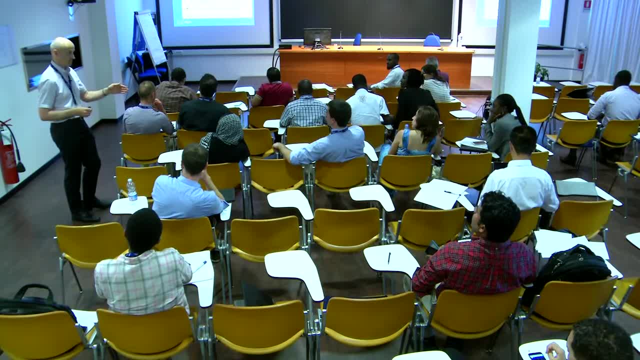 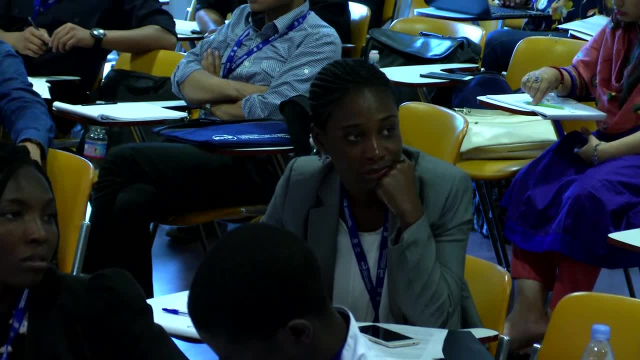 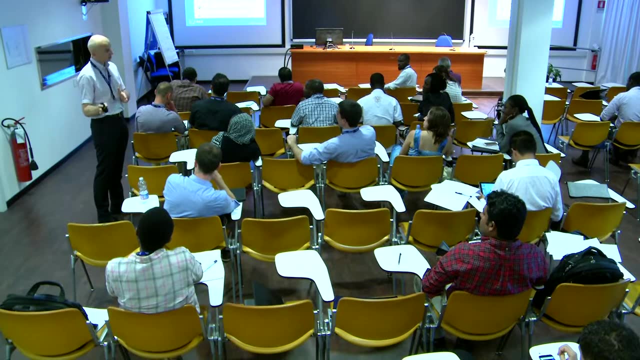 like Sweden, like Finland, like UK, all of them had the Research Reactor while they were building this capacity and capability. and now they say, if I need the Research Reactor, I will go to neighboring country and get myself served. but they say: for our NPP. 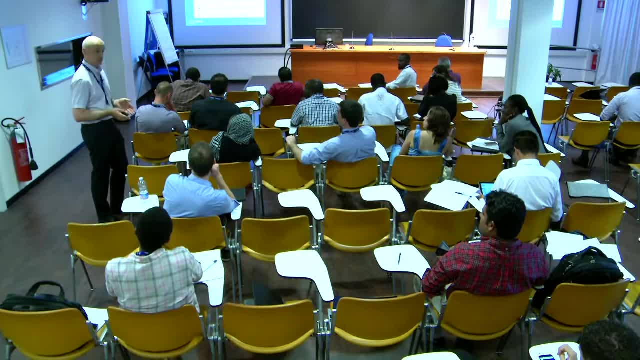 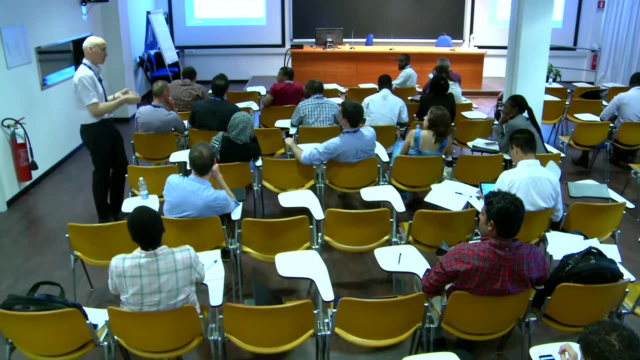 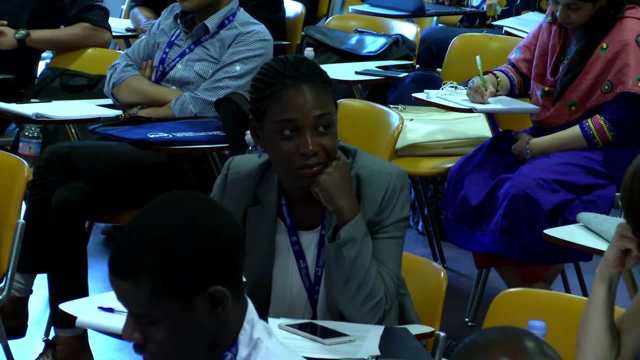 we don't need it, except United Arab Emirates, where they say we go directly NPP without passing through the stage of Research Reactor. but this is my personal opinion- personal, not IAEA opinion is very extreme example: because they have money they can buy Operator, trained Operator. 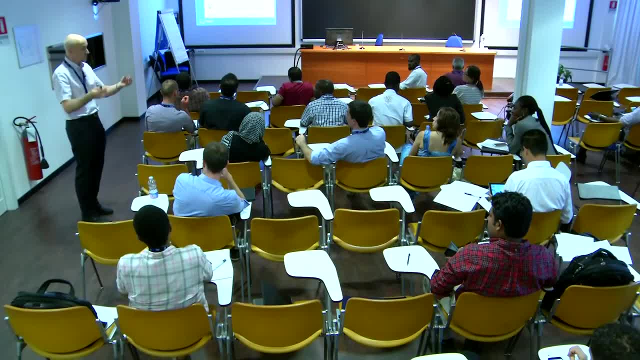 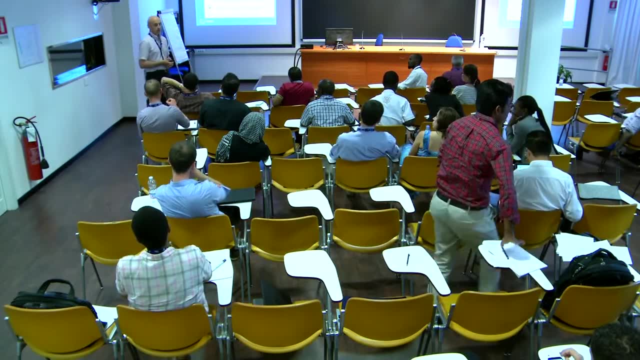 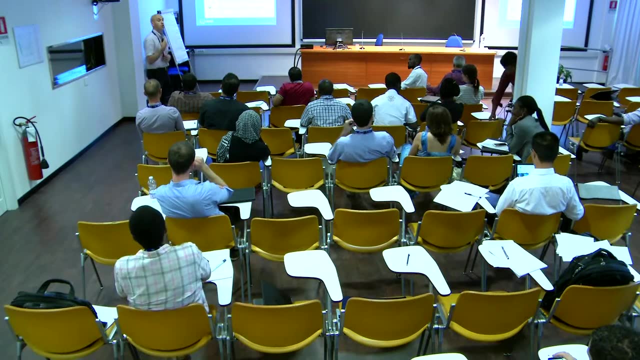 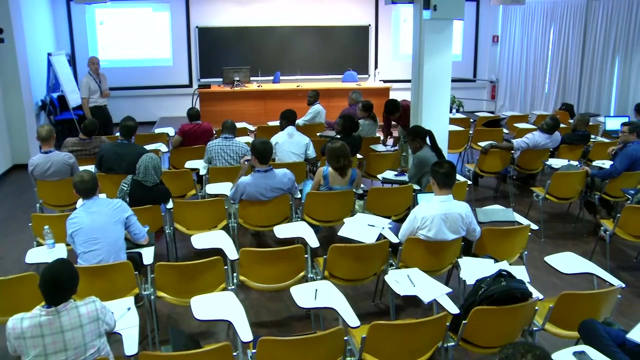 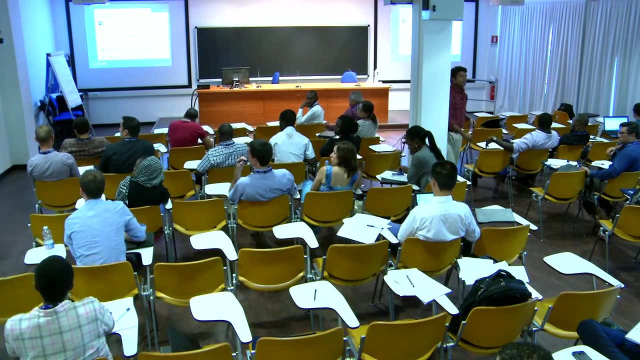 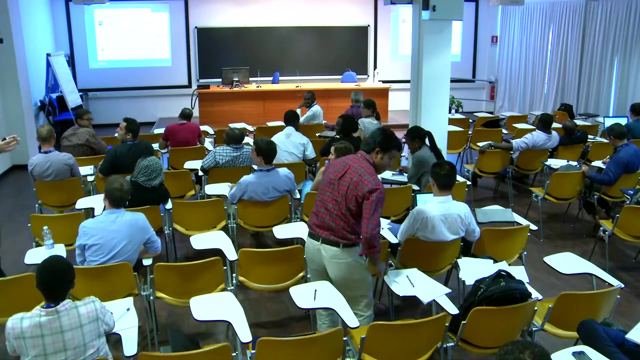 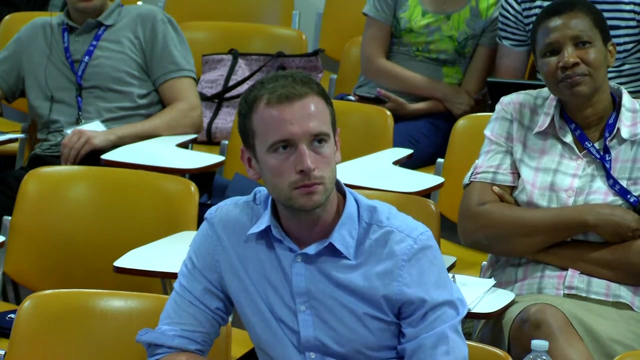 it's not necessarily maybe- will develop on their own all necessary capacity to be completely, you know, be the masters of the NPPs. so that's personal opinion. yes, you can continue listening. the high enrichment of fuel is key, because more enriched fuel you have, more Uranium 5 you have. 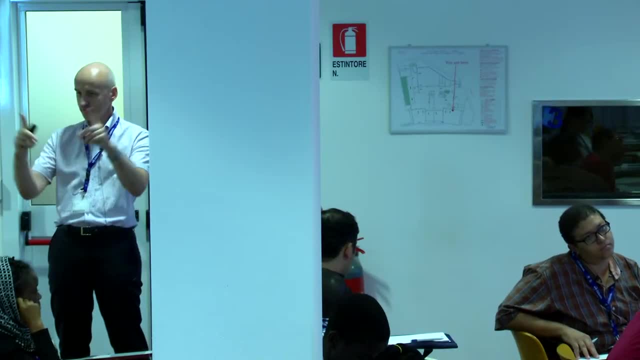 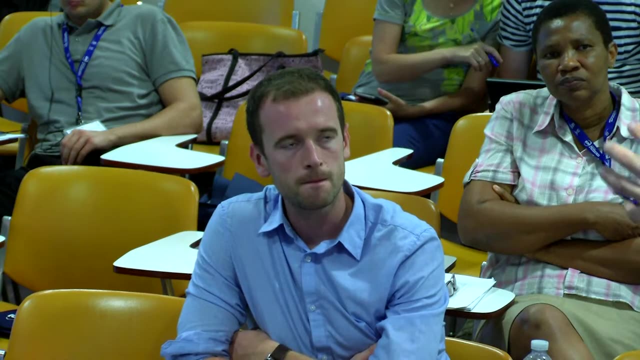 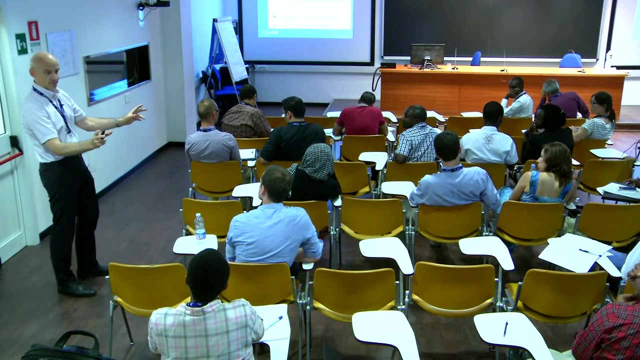 in a small volume. so the flux goes like R square out of the source. so you aim at compact course and very dense Uranium 5 concentration in this small volume right now. you will put a reflector. you will get some neutrons back. that adds another percentage. 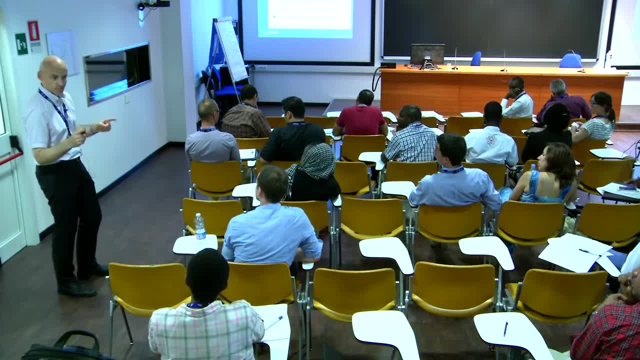 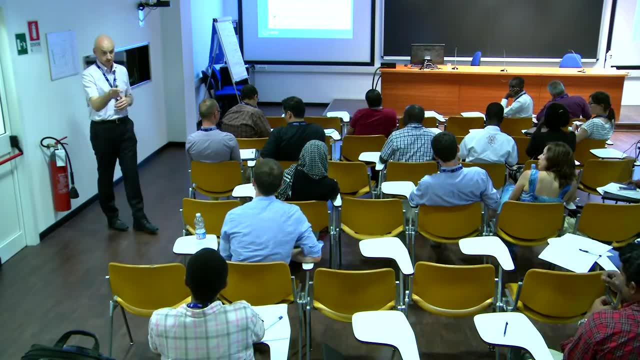 but reflector moderator, you will not have much of fast. so then it depends on the design what kind of neutrons you want to produce, but that's what only allows- I will speak about limitations afterwards- to go to the levels of 10 to the 50 Newton per second. 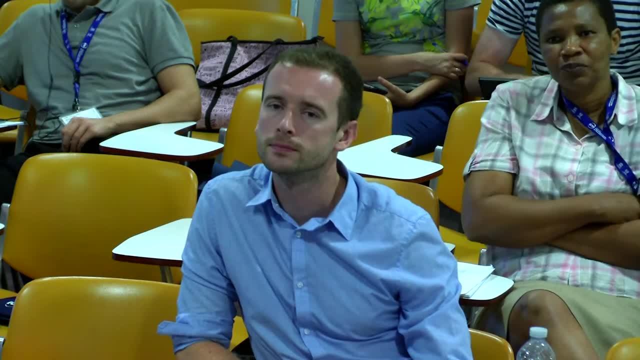 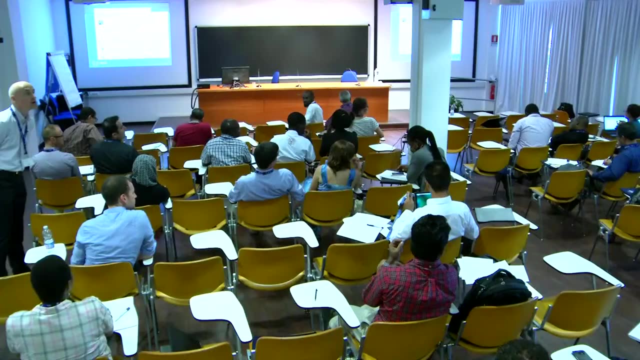 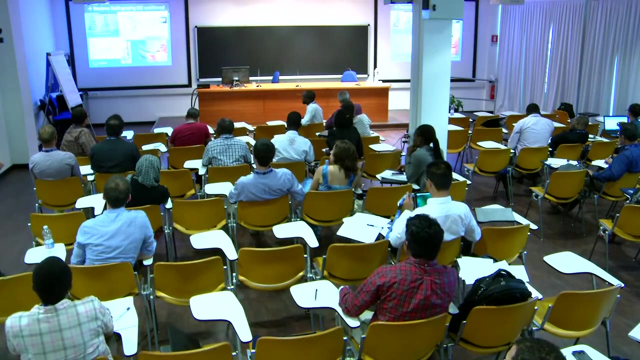 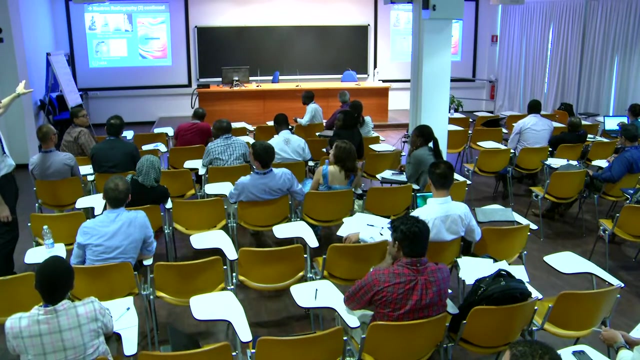 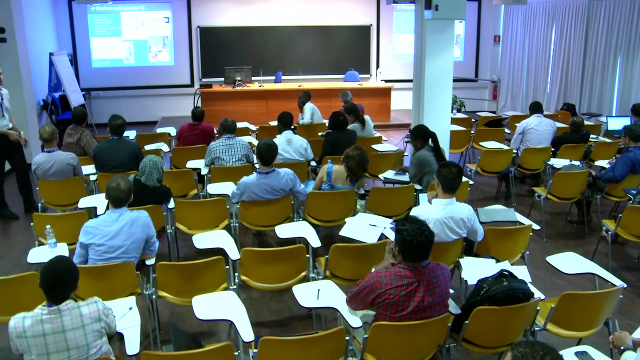 square centimeters. okay, I think I. yes, that's a reactor specialist depends. this again depends. for this one it can be 30 minutes, it can be a few hours, it depends at the flux level, at the sample irradiation position at your trigger. in Malaysia you might need a few hours. 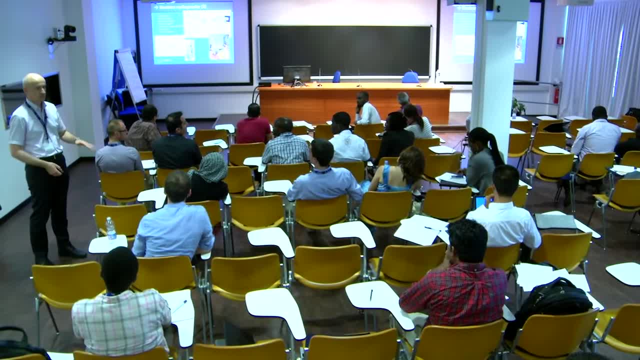 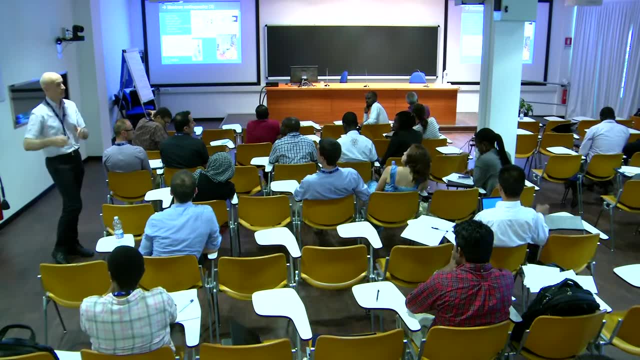 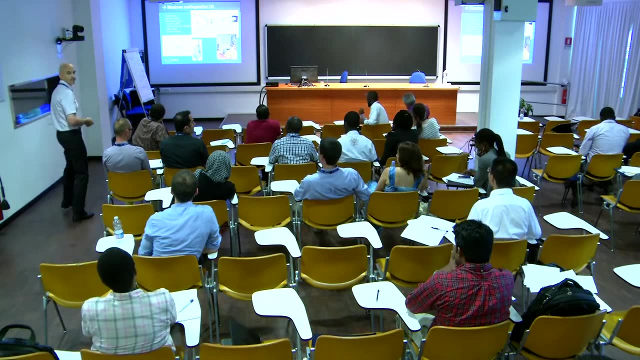 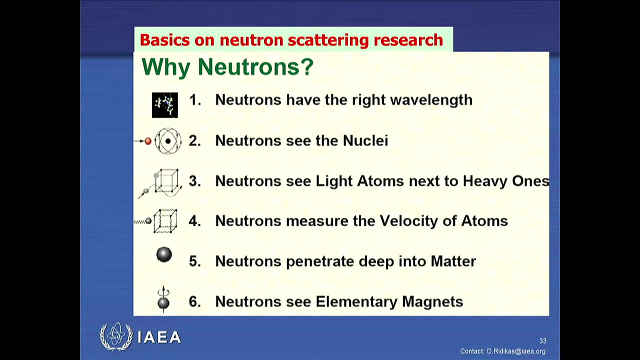 in, say, German reactor which is 20-30 megawatt, it might be tens of minutes, because they have much bigger fluxes and they can do the projections and rotation of the sample much faster. okay, neutrons. so why neutrons are so particular compared to other particles? 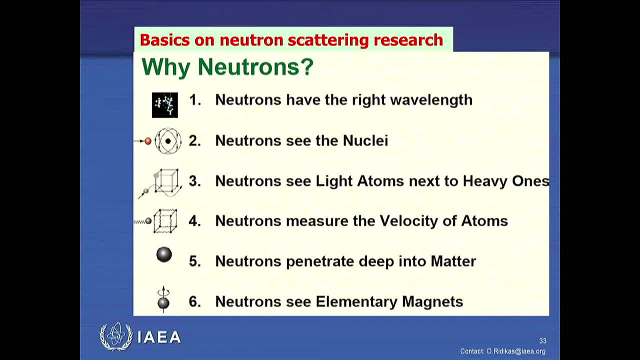 because they can be managed at different velocity, a different energy. we say in quantum mechanics. they have right, wavelength. yeah, somebody took quantum mechanics course. wavelength is relates how fast and how frequent oscillates the wave. if you look at the neutron as a wave package, neutrons can see nuclear. 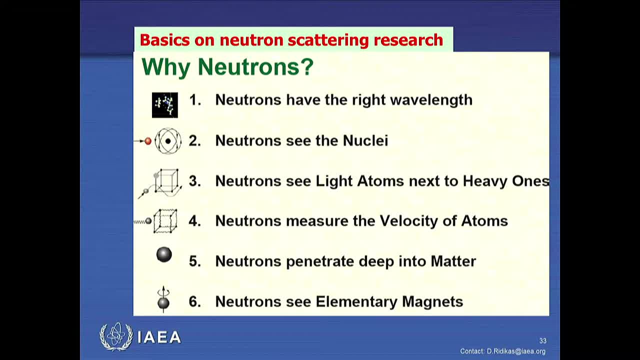 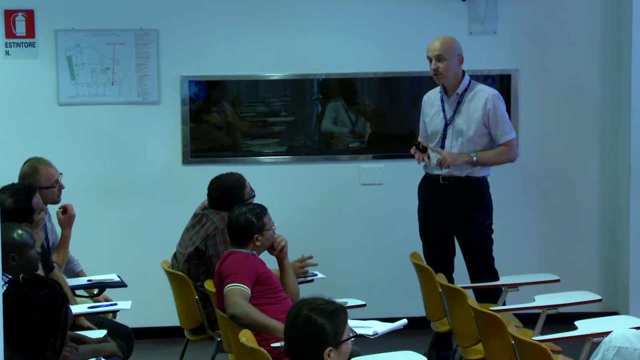 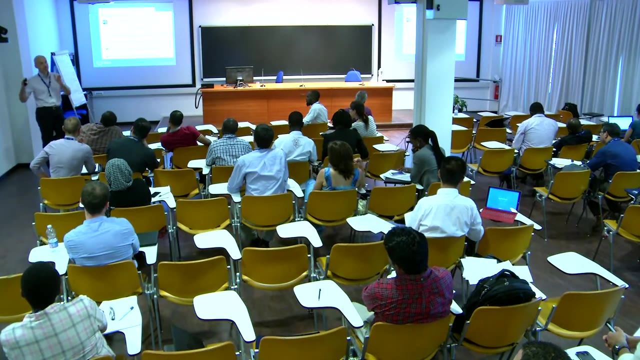 through interaction, typically scattering, capture or making another reaction advantage. another advantage is that neutrons can see light atoms like lithium, hydrogen, boron, together with very heavy ones like uranium, lead, mercury, right yeah, and that's not the same with the x-rays. x-rays would see mainly 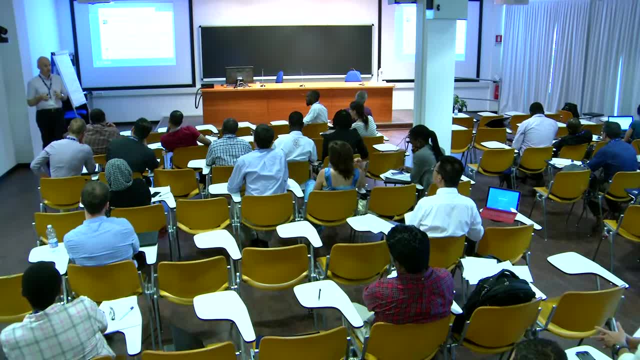 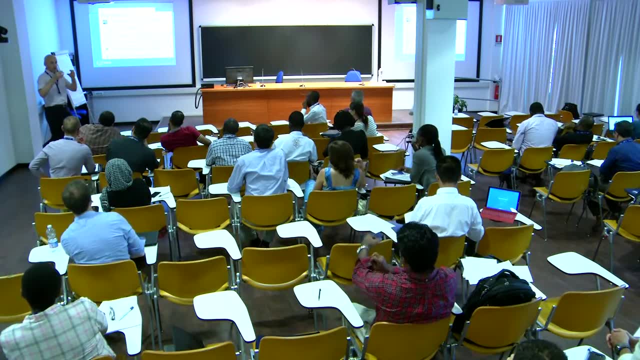 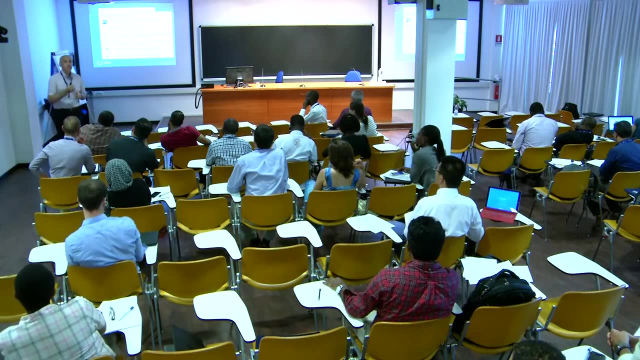 because of atomic interaction. atomic interaction mainly high and heavy elements. neutrons can measure the velocity of atoms, every atom, including our body. they move, and to say how fast they move in which direction. neutrons can help you to do that. because neutrons have no charge. it can penetrate. 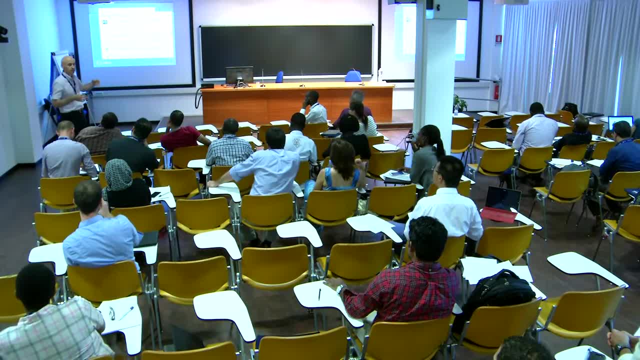 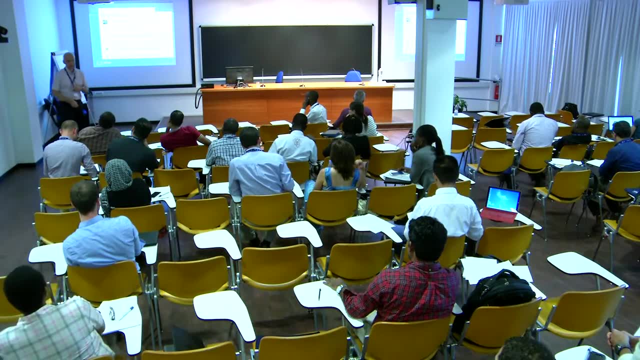 very deeply and this is advantage because it can- you can work with very big samples in non-destructive matter and neutrons have a spin, so it's it's very good probe to work with magnetic materials and magnetic materials in some of the areas is their future. 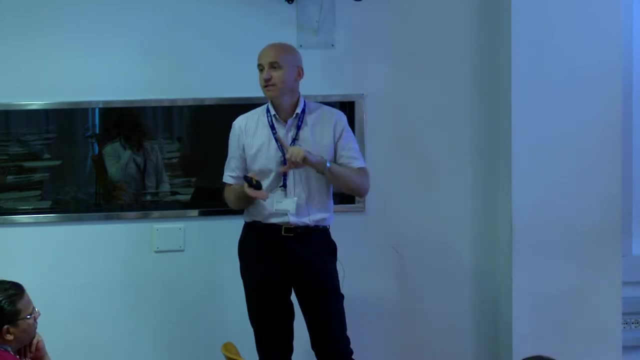 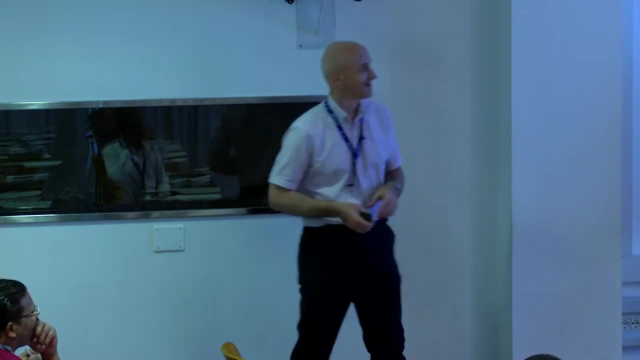 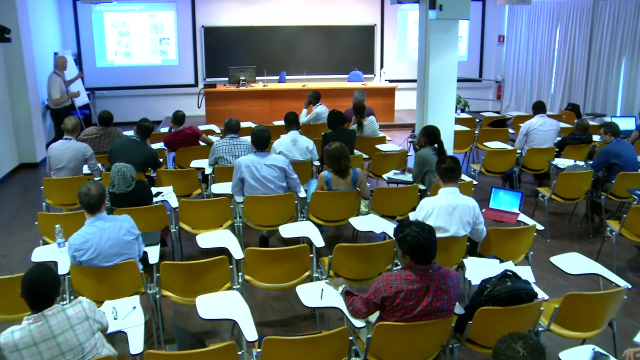 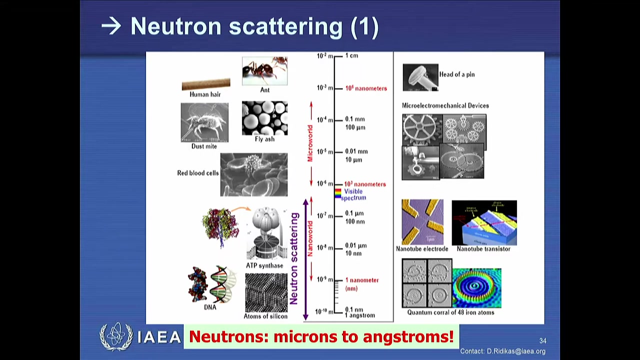 so because of these properties- at least if you understood 50% of what I said, or, I hope, 90- it allows you, with neutrons, to study from tens of centimeters real objects down to nanometers or parts of nanometers and study human hair red blood cells. 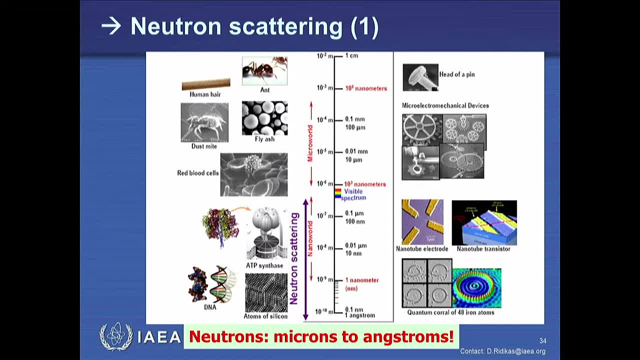 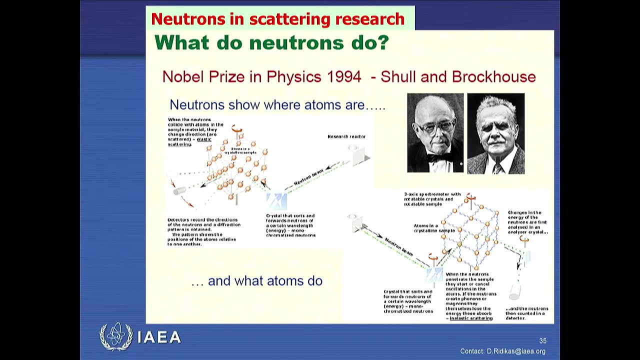 and even down to DNA. yeah, so it's very large dynamic range where neutrons can come. in terms of structure studies and material studies, it's very simple concept that neutrons show where atoms are and then you can do through what you call elastic scattering. it's a 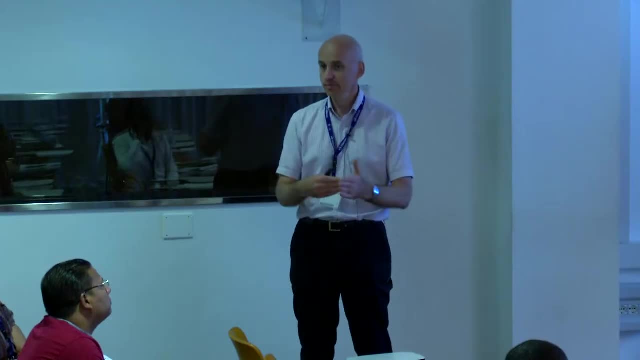 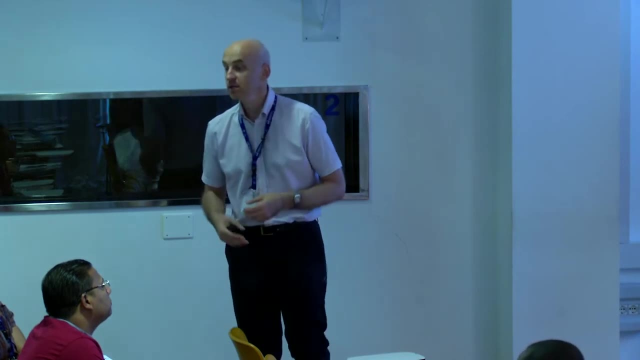 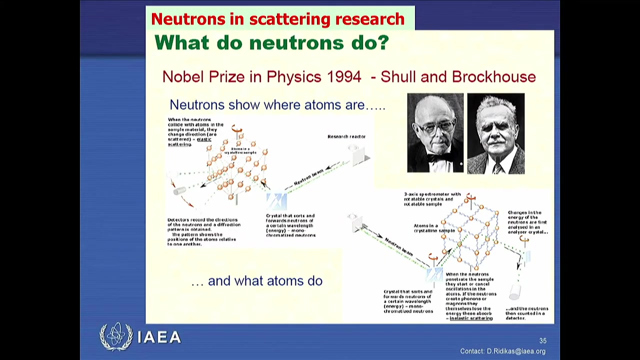 billiard game: right, elastic scattering. yeah, in most of the cases no energy was transmitted, or very negligible, and you see just a different angle at the same velocity coming the ball. that's elastic scattering. if some energy has been taken or given, this is an elastic scattering, yeah. 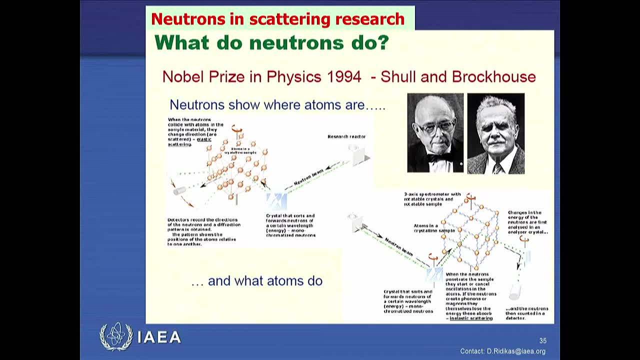 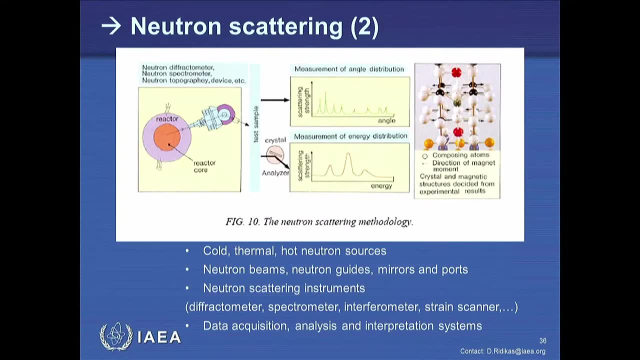 these two simple concepts. these guys got Nobel Prize. so sometimes life is simpler than it is, yeah, so what actually typically you do? you get neutron out, you let it interact with the sample and you measure after interactions, the neutron angle and energy, and that allows you to tell a lot. 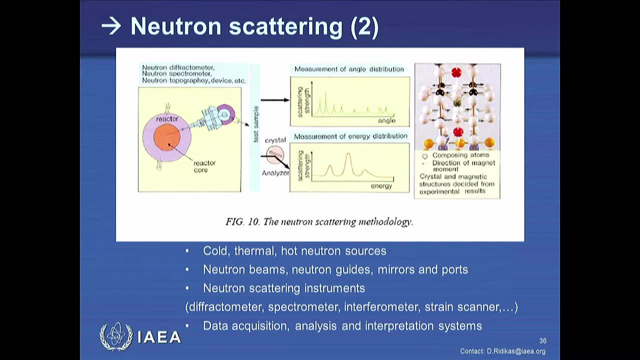 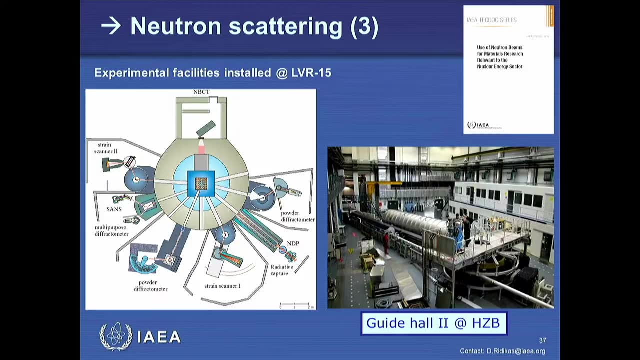 what has happening in that particular sample. this is a basic concept of neutron scattering for materials research. so that's why when you visit research reactor, you don't see only the reactor core with the shielding, but you see many beam cubes- what you call beam ports- going out. 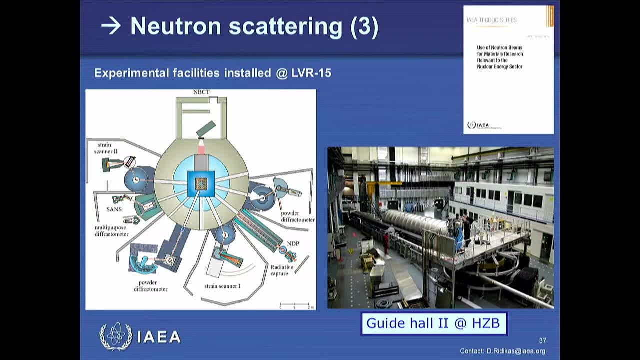 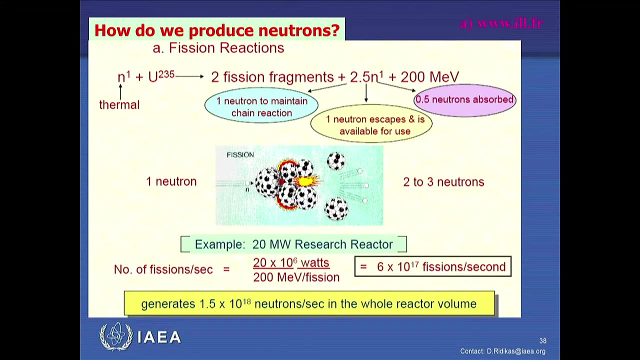 in a scattering area and some of the detectors look as big as that, because you want to do high level physics. with the neutrons coming out, you can study different materials at different temperatures, pressure levels, etc. now I have to tell you the full story. research reactors is not the only. 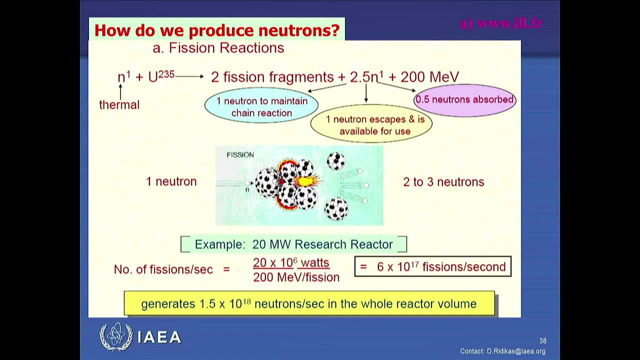 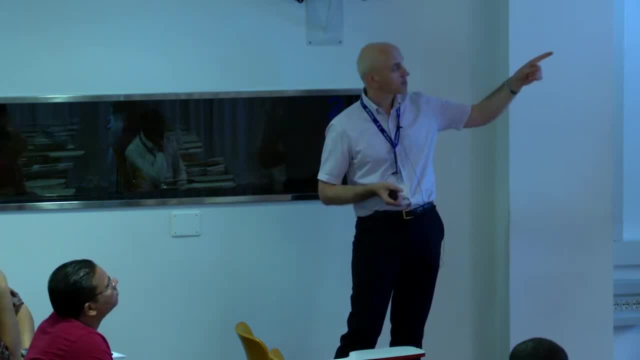 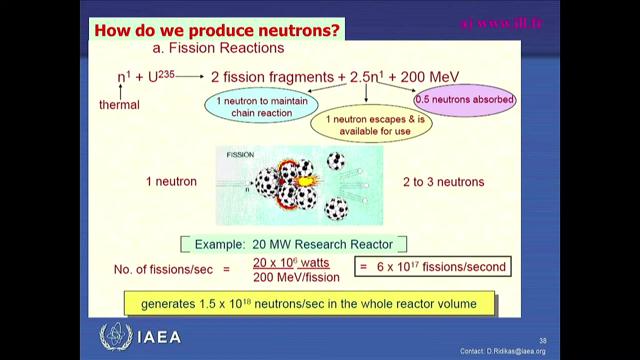 source of neutrons. we can produce neutrons also using particle accelerators. so what is happening in research reactor? you have fission reaction where after each fission you emit on average two and a half neutrons per fission. so some of these neutrons need to maintain. 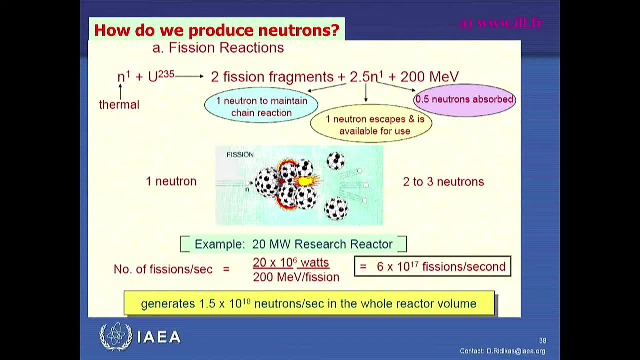 chain reaction and then some of them are absorbed and some of them escape or can be used externally for research. what we are doing and that still allows chain reaction to continue. yeah, that's the, the principle. so 20 megawatt research reactor on average creates this amount. 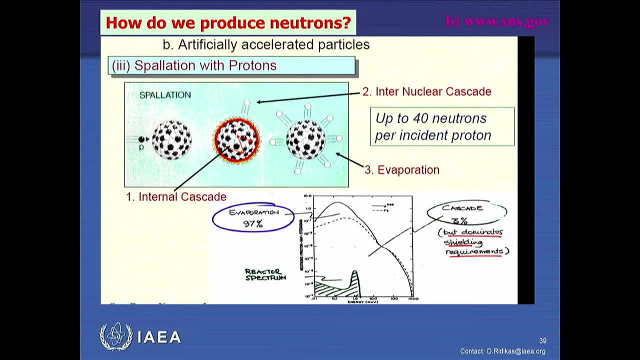 of neutrons per second, so it's enormous neutron source. now you can do similar way by accelerating proton. neutron proton, that tells you something different. okay, proton to very high energy, interact with heavy metal target and after each reaction you will emit up to 30- 40 neutrons. 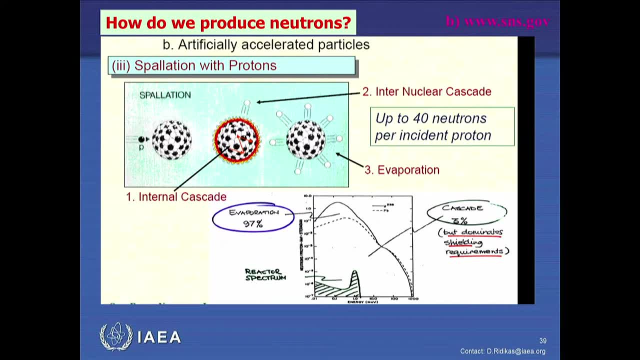 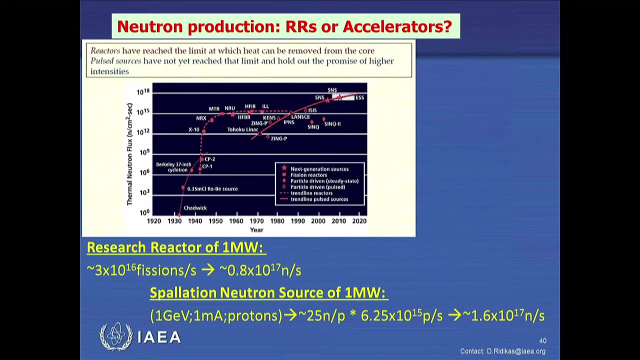 per incident proton. if you have high intensity proton machine, it allows you actually to create equivalent neutron source compared to one megawatt power reactor. so you can the message here: you can produce neutrons in two different ways: without nuclear material, without criticality, accident potential criticality. 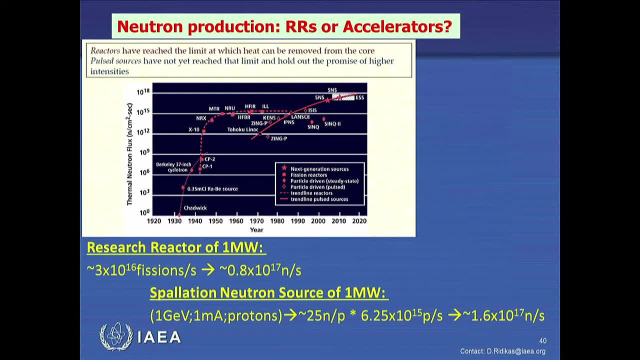 accident or incident. but how far you can go with two technologies? neutron has been discovered by accelerator, not by reactor, so they have one point plus right? yeah, then reactor technology, the starting first. critical assemblies in russia and us went very fast and reached neutron levels to 10, to the 15. 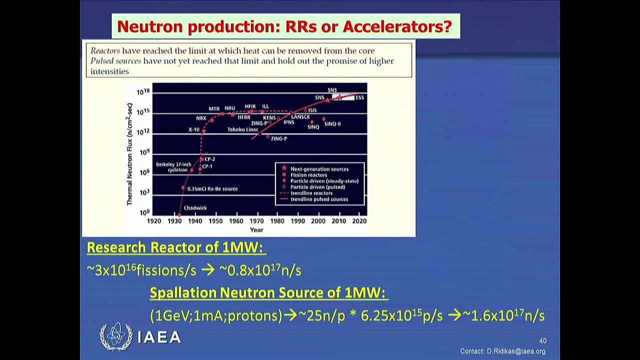 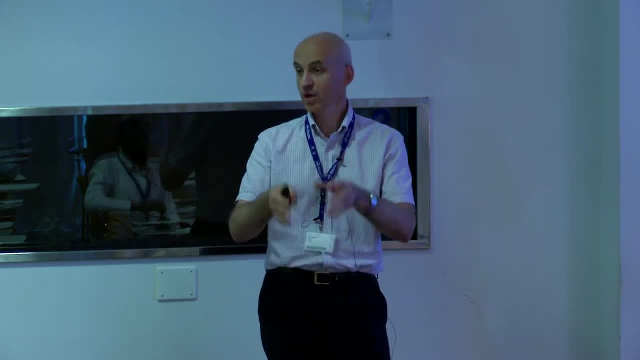 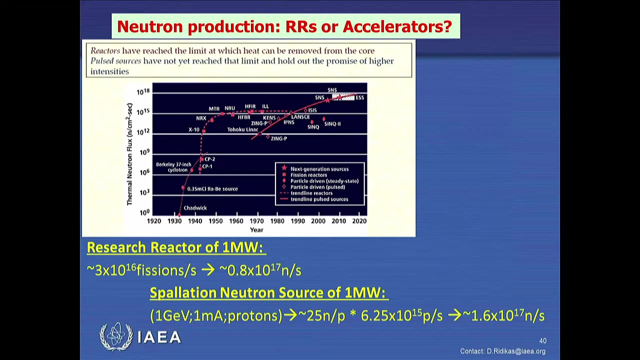 which is typically 20- 50 times more than any nuclear power plant operates today. that's why i said with the research reactor you can predict the future because neutron flux available is much more in research reactor than mtp. but that has reached the limit because we have 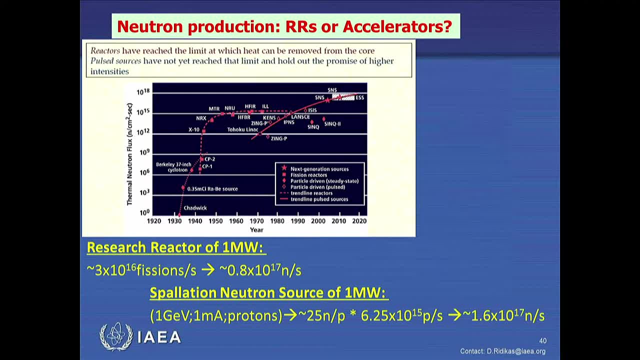 problems with heat removal. so if you want more, the fuel will melt because we're not able to take away, neither geometrically nor technologically, the heat from the reactor fuel. so we need a major breakthrough in technology and thinking how to create higher neutron fluxes using little. 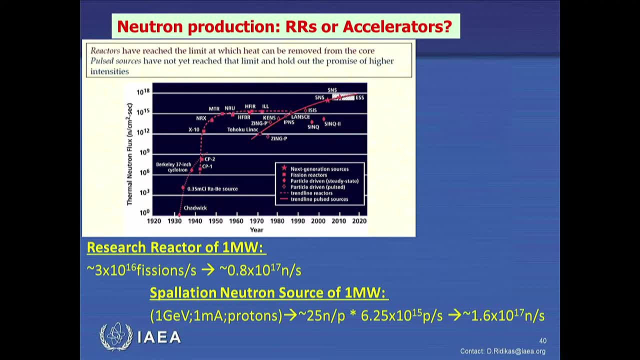 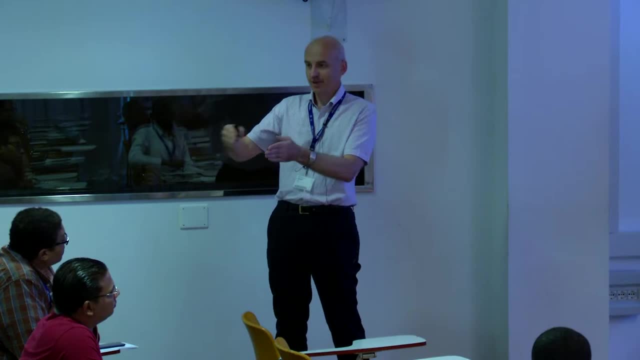 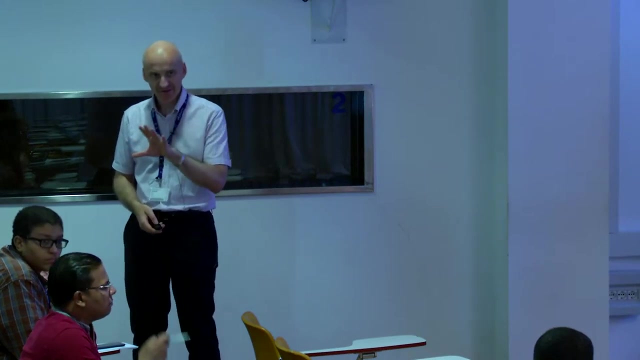 shattered technology accelerators can do that, but they do that only in post mode. they can create neutron fluxes two orders of magnitude higher than that, but for very short period of time, and then they use this time without neutrons to cool the target. okay, yes, i will go now. 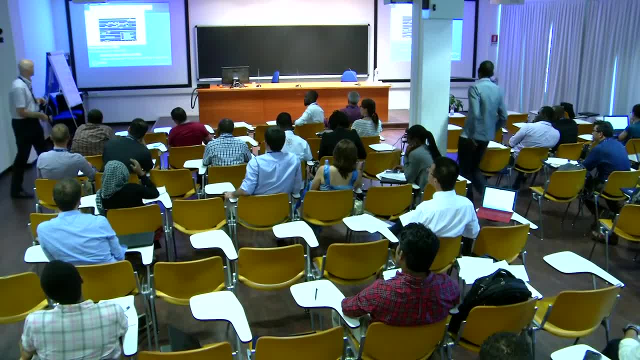 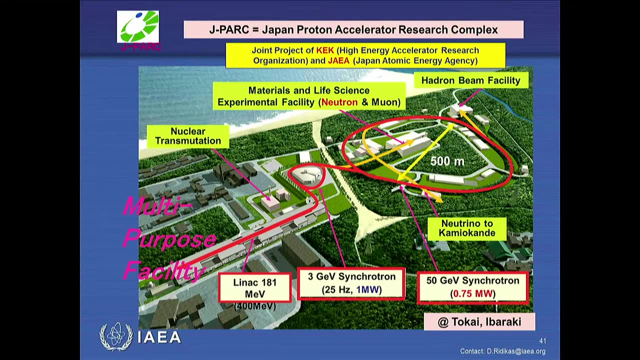 typical example what we're talking about, what kind of technologies we're talking about. research reactor can fit in this building easily with all equipment. critical core: you need to have a high energy particle accelerator. you need irradiation target and even more they itself. the target technology looks like: 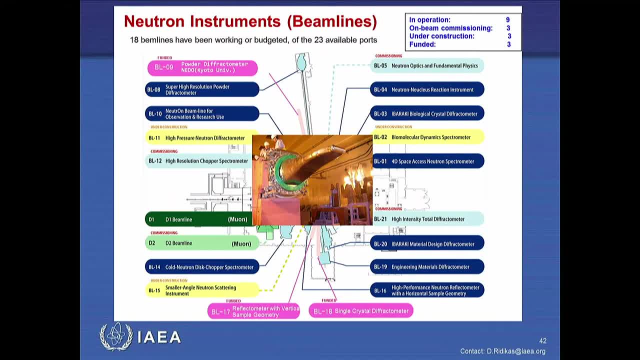 that that's a liquid mercury target with 20 tons of liquid mercury circulating and this is the size to receive one megawatt proton beam to create neutron flux equivalent to the research. so it's possible, but this is a billion project compared to the hundreds of millions. 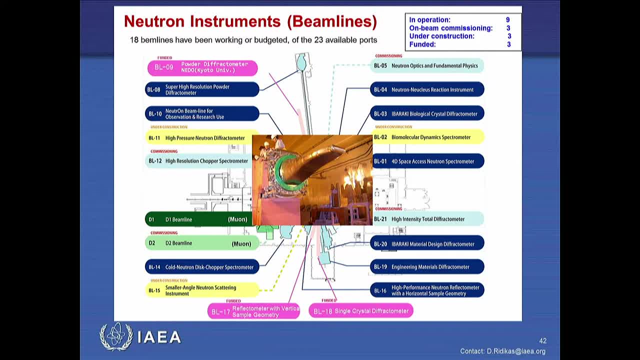 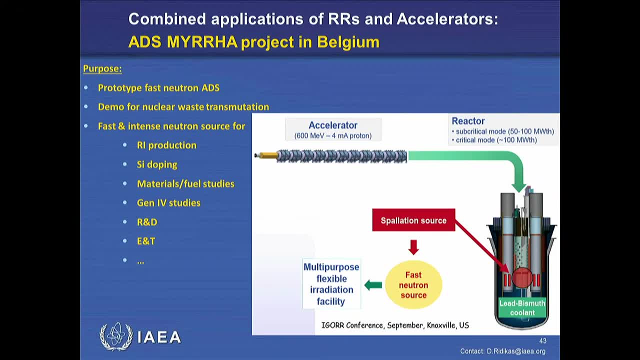 for research right, so meaning not every country can afford that for research purposes. you can combine both accelerator and a reactor. why would you do that? why you cannot run them separately, while there is good features of both of them. this combination allows you to run subcritical core. 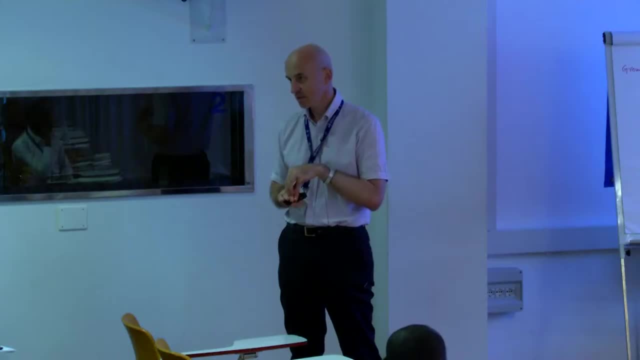 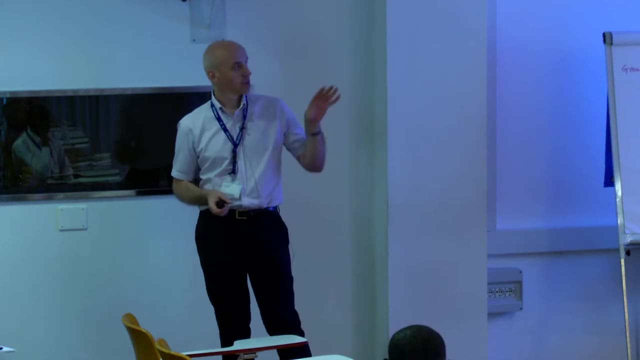 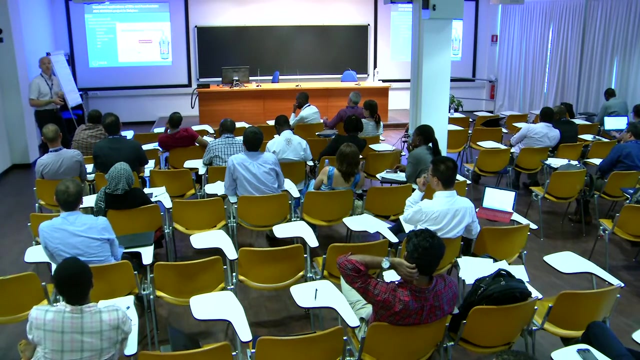 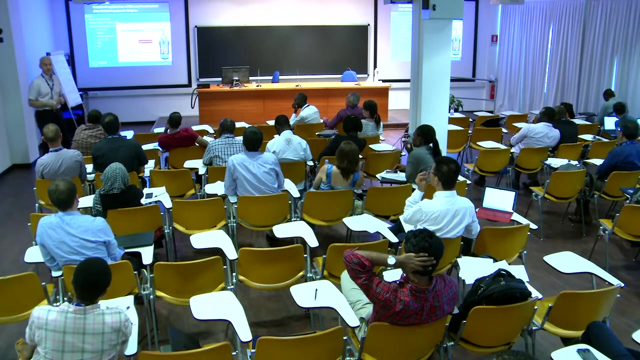 because of the external neutrons coming from accelerator. that means this. so that allows you to do that. otherwise it works like a typical good neutron source. certainly it's going to be even more expensive, but you don't pay money for nothing, right? you pay at zero, you pay. 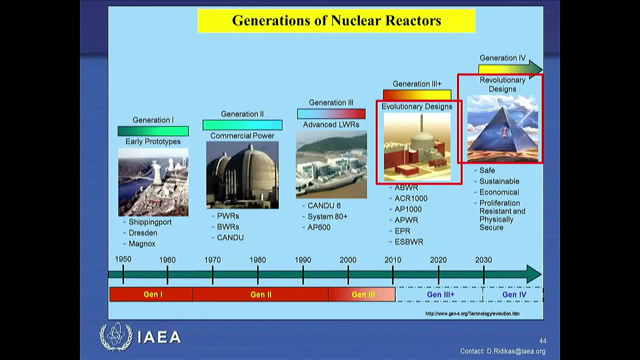 for zero risk. so you would have to be prepared for the second question, what you will get during your maybe i don't know, maybe that was done randomly, but be prepared. these are typical pictures. maybe you've seen that already, i don't know, or, and some of them: 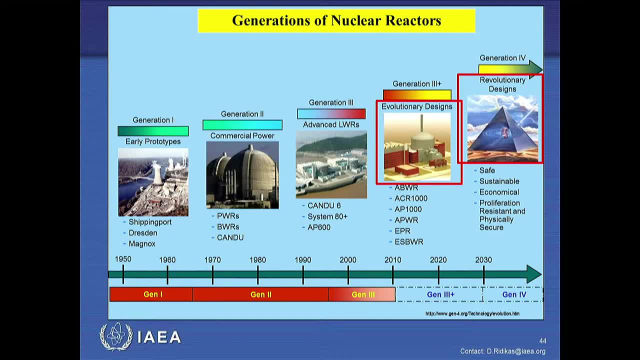 generation three plus. what does it mean? it means that, compared to generation three, we have not added substantial breakthrough in the technology. we improved in safety, we improved in fuel efficiency. that's why this design is called evolutionary, but there's no major change in the technology. so if 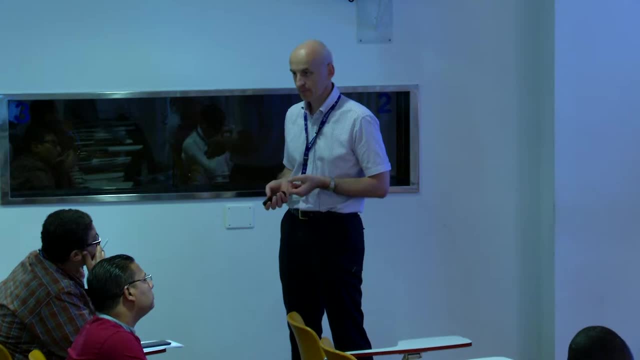 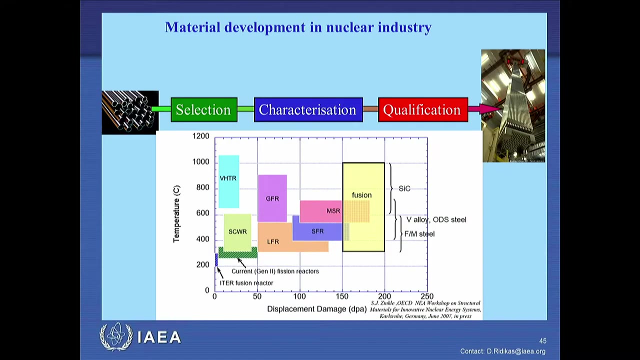 you want to go to generation four, you need to make a revolution in nuclear technology, and one of the aspects why we call it revolution is that we will work with completely different materials, because presently, operating materials for light or heavy on industrial scale, we're not able to. 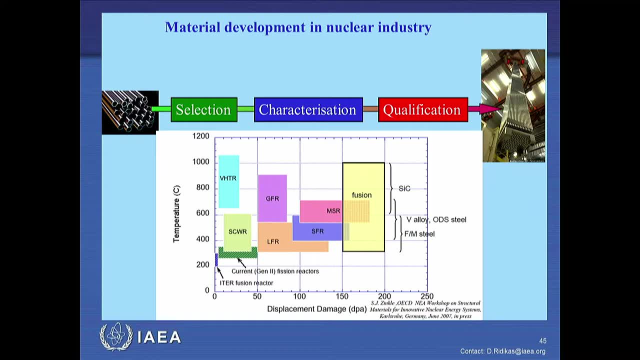 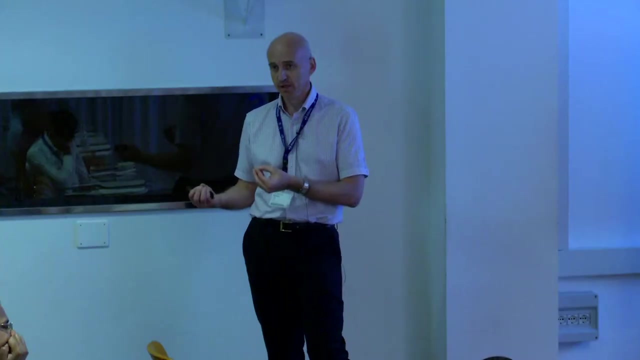 do that because we don't know yet which materials to use. we can do prototyping, we do some tests, but at the moment we are not able. there are two parameters. one is easy to understand: these new systems. many of them will operate at much higher temperatures. then we 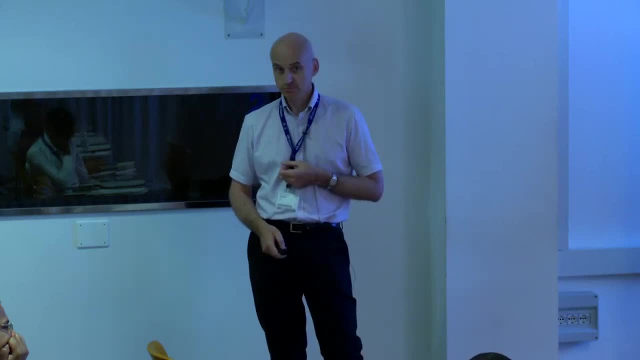 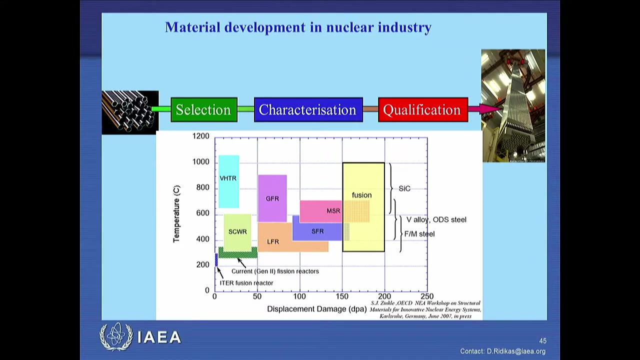 know which materials to use, being steels, alloys, etc. now, if you want to go to very high temperature reactor, gas fast reactor, molten salt reactor- some of these are not thinking about the matter and most of these today are limited to 50 dpas for the 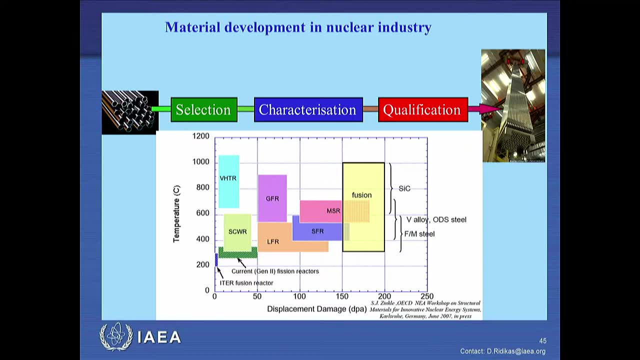 entire life of the material to be radiated. now, if you want to go to fast reactor- fast neutron makes more damage than thermal neutron to the material. you need to have structure materials which are able to withstand higher energy. you are receiving a lot of information and it's 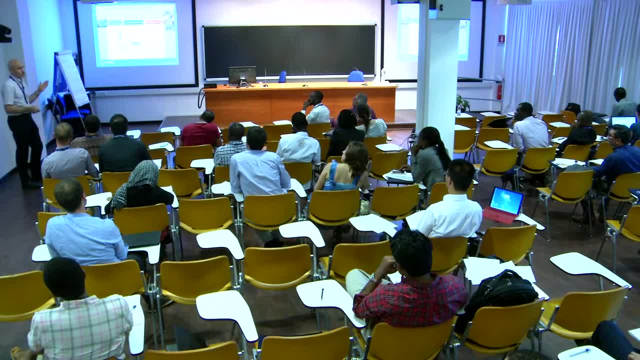 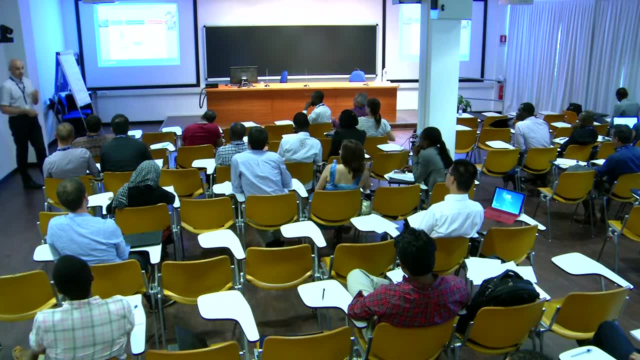 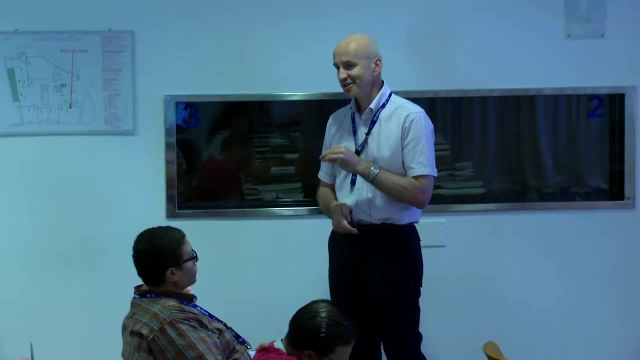 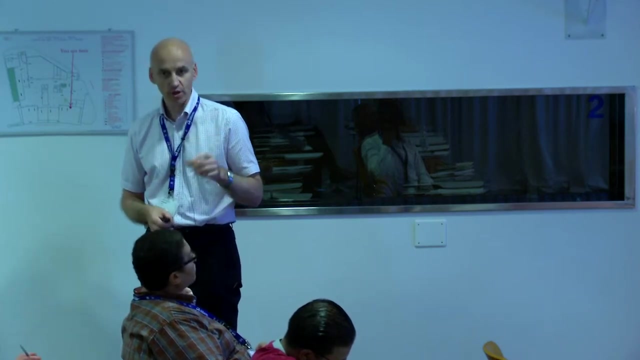 okay, you don't understand everything because i know some of you are not really nuclear. background message here that if you want to do research you need to have a very high flux. you can have neutrons- thermal or fast- and you can irradiate materials in a realistic 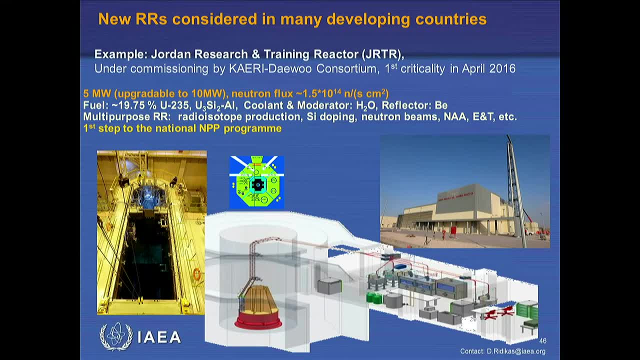 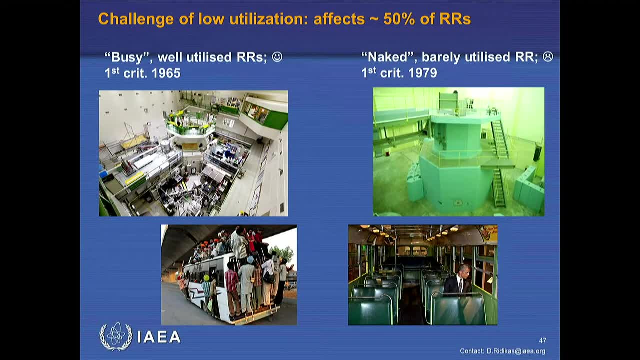 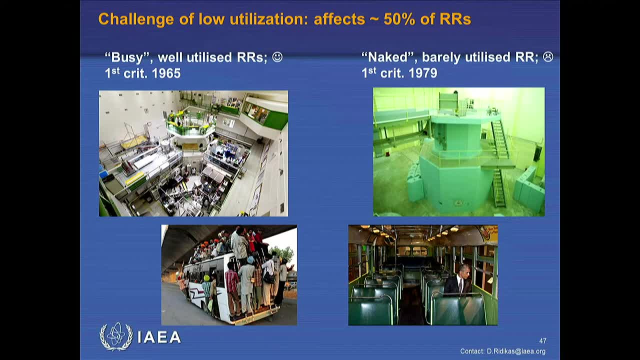 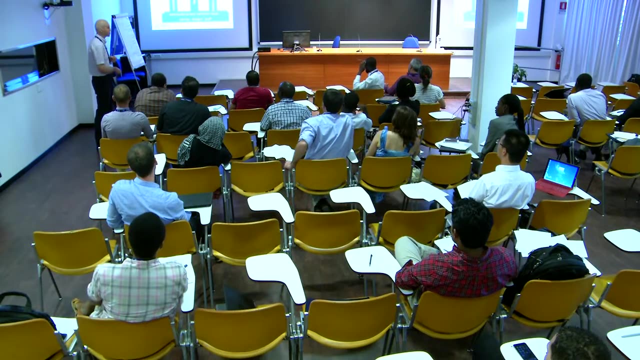 in a number of countries. I'm not saying you have to equip a reactor like that, but driving a bus with one passenger it doesn't make a lot of sense either. So we need to think about new strategy for research reactors to build on two important 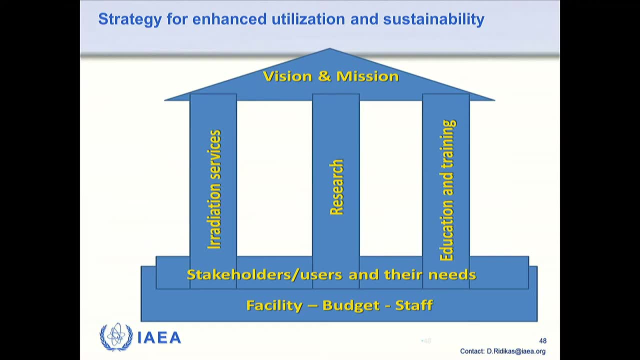 foundations, the user who is requiring access to the neutrons, who is your stakeholder justifying existence of your research reactor? So we need to clearly know whom this research reactor is going to serve. Based on that, I will design and adapt the facility, with the budget and with the staff. 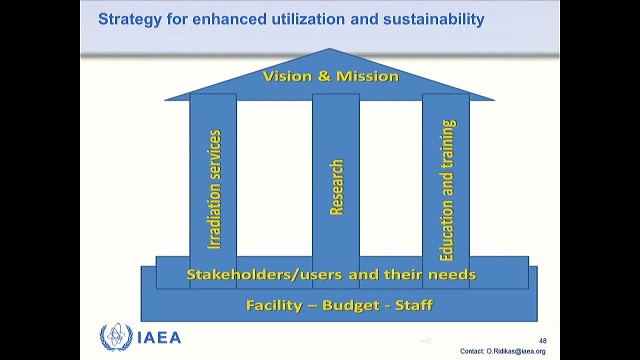 So these are two important factors. Thank you. The next slide: Use of nuclear technology. I'm going to first explain the changes we'll be taking, the benefits of nuclear technology, And then I will explain the impact of nuclear technology on the environment. 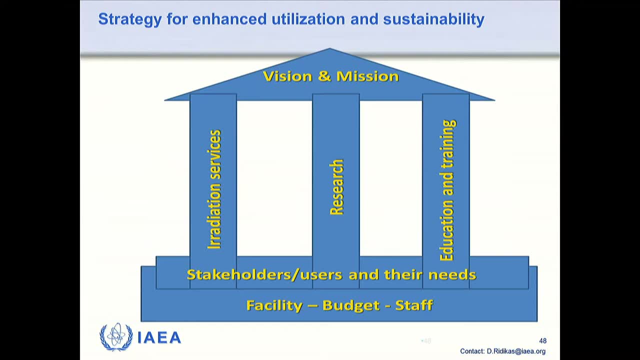 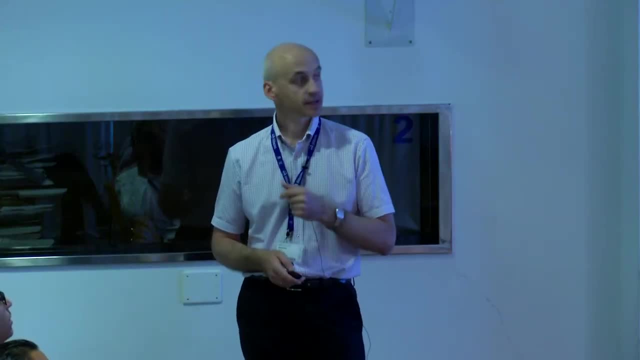 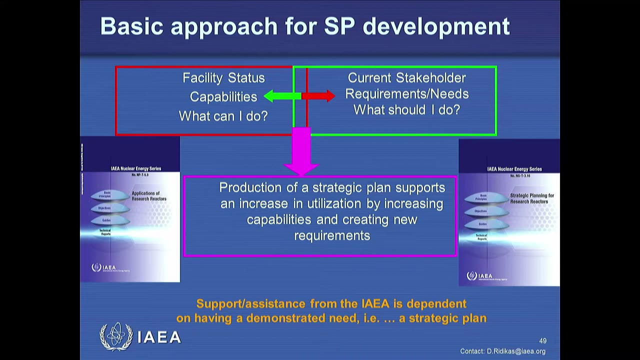 I want to start by explaining how it affects the environment, if you will. Well, I think we are seeing a lot of potential changes in the environment. Think of it as a nuclear power plant. almost we can design the right facility, and all that contributes to the strategy justifying a research. 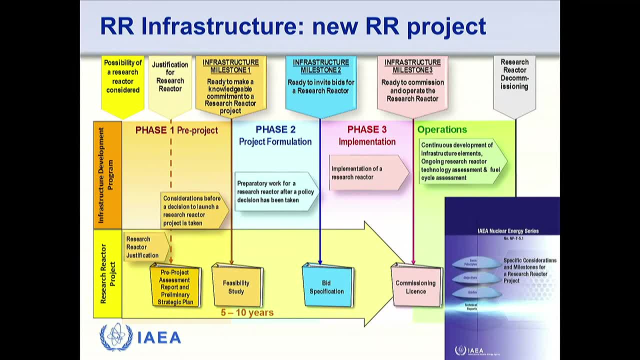 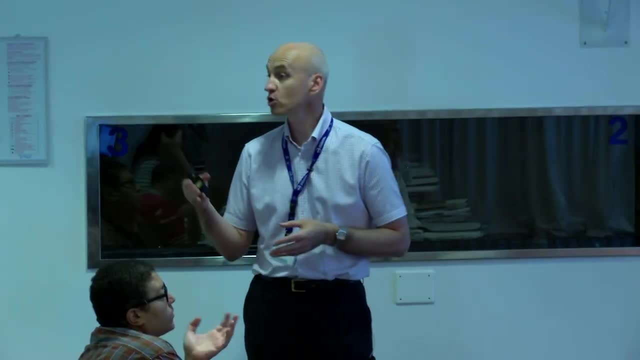 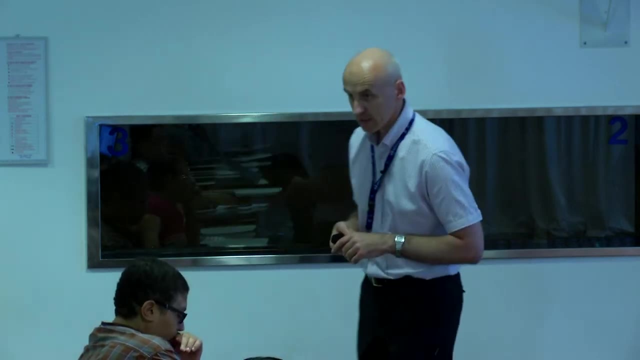 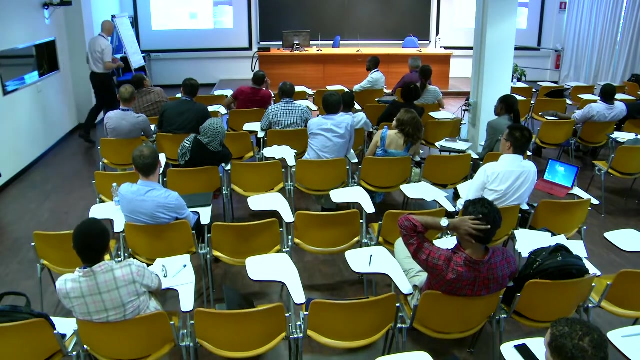 reactor and ensuring its efficient utilization for the future. research actor project is a nuclear project, so milestones approach applies also to building, considering building and operating a research reactor as well. research actor has a nuclear fuel, so security, safety and safeguard regime applies to research reactor facility as well. therefore, we have a consistent approach. 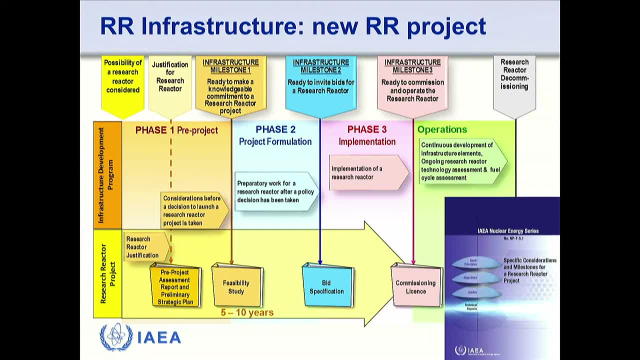 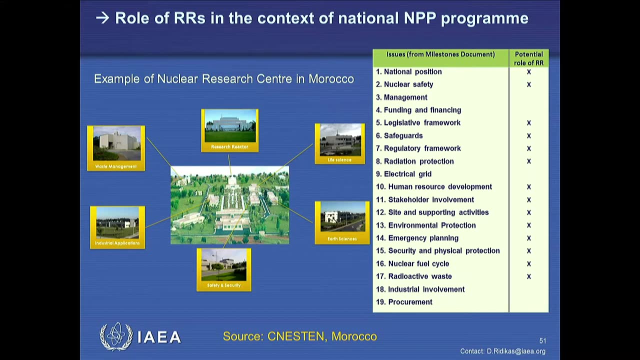 how to help member states to develop new research actor project using almost identical milestone approach as to mtp, where we also have 19 different issues and indeed member state appreciates that. saying that, going through 19 infrastructure issues and building a research reactor, that's a step forward to cover, maybe not completely, but in part. 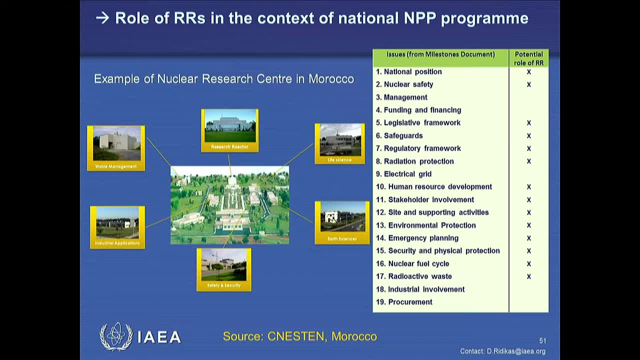 in preparation to the future mtp, and this is exercise for morocco. when they did, they say okay out of 19 issues- majority of them at least- we considered, we touched, we progressed and we feel more comfortable now to go for mtp. i believe that the same applies to 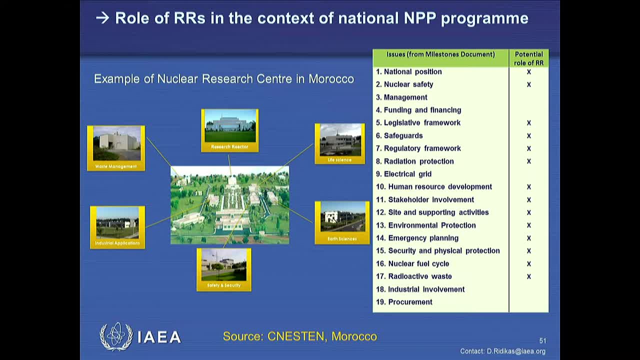 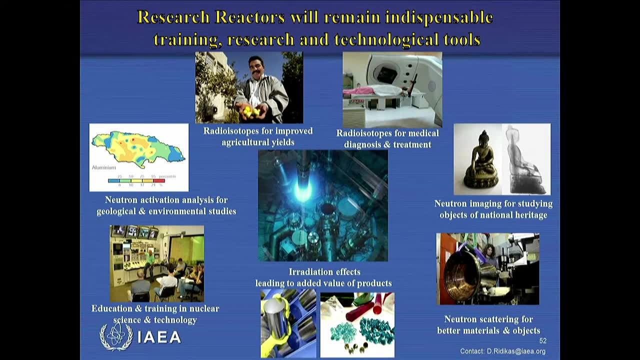 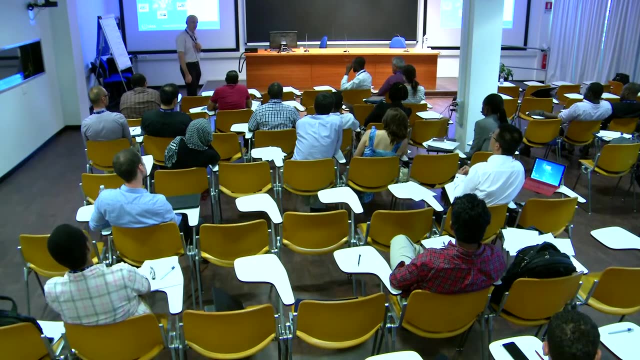 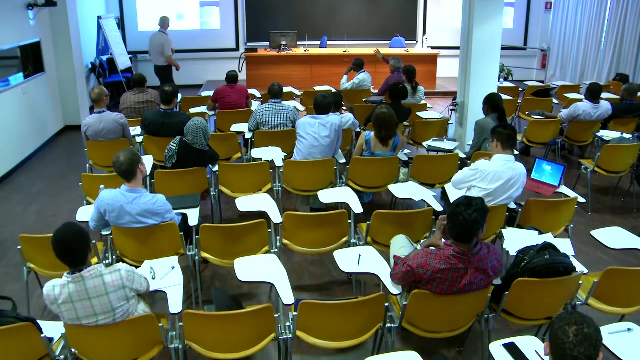 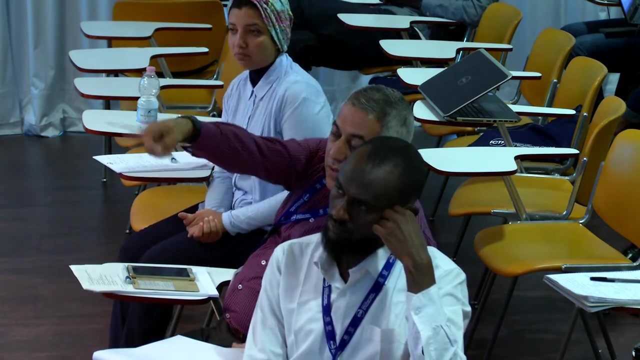 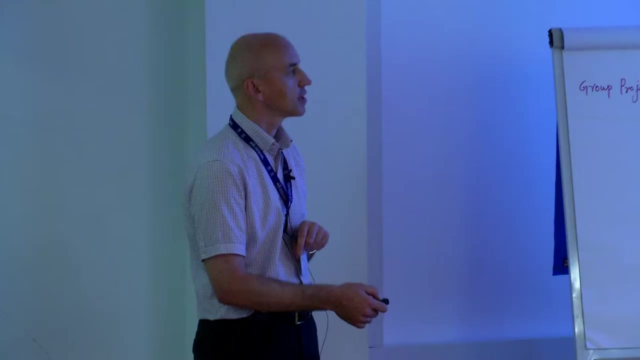 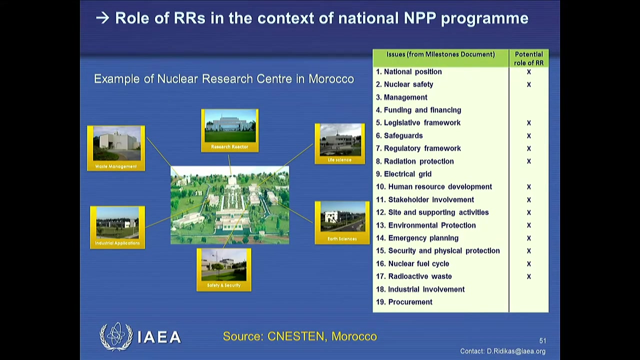 jordan- and these are two new newcomer countries- recently went through research reactor and now making future steps for the national mpp program. yes, yes, pre-re Italo strategic plan even before the decision is made. it's not, it's on the utilization: yes, this is 19 infrastructure issues of mpp. so issue nine, electricity grid, is replaced by utilization. uh, issue. that's the only name of the issue or different issue, that is their name. if you look at the also need this good الم, sacrificial possibility. you continue, please you, thank you, protec all the thank you. the only name of the issue or different issue, it's that one by know middle paper, brown pointed. the issue with the number 1 thing one, the number of neighborhoods. taker kalyan means cuttingâm прид Passafaloc, building the move forward. it'sREP LIFTO where it would refreshing start and then cross that timeline. so you are outли nostri me grad plus 3 in mid australia area. ATP executive agency. 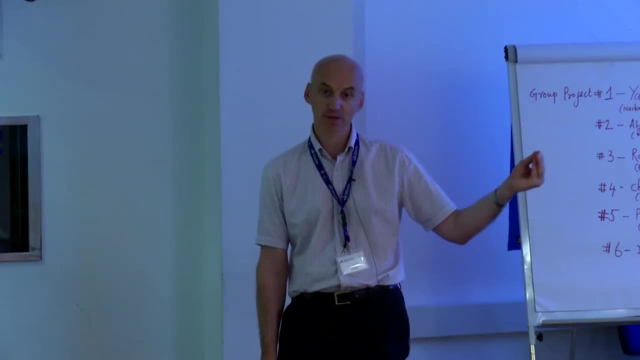 원� popular network. we developed a single supply sector. this is in the itcom, that's the only name of the issue. different. It's a different issue compared to- because, as I said, NPP electricity research reactor, everything else except electricity. 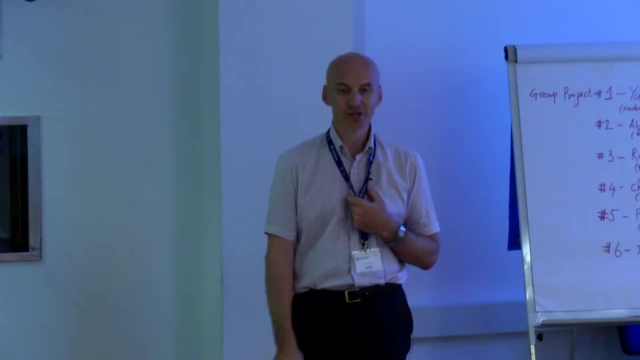 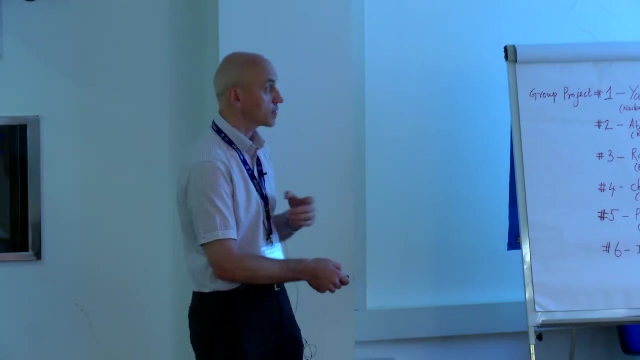 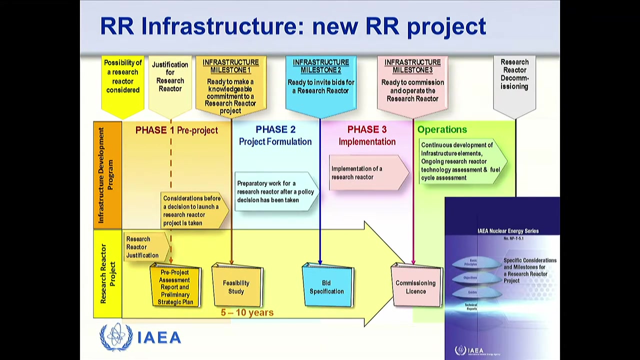 On the issue nine, which is called utilization: Yes, Of course It should be even in the phase one, before that helps you to make a knowledgeable decision. Your strategic plan has a role: to help you to make knowledgeable decision. Once reactor is constructed, strategic plan will guide you how to utilize the facility. 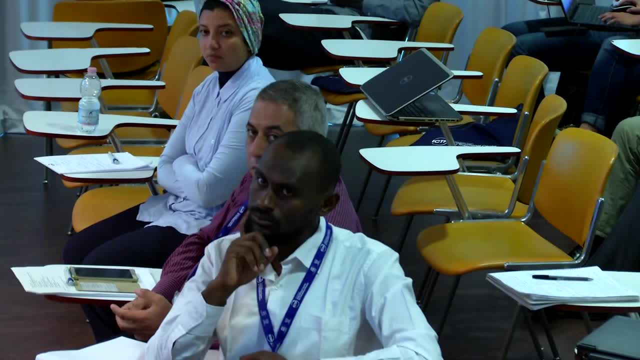 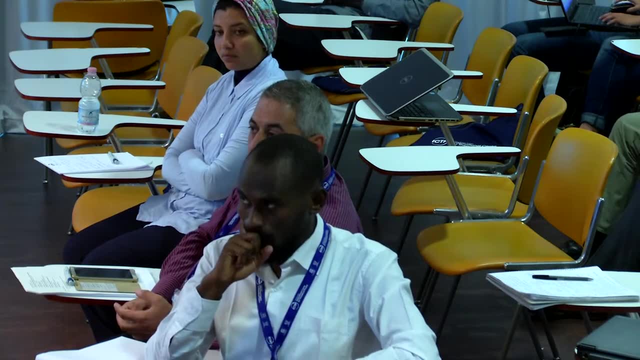 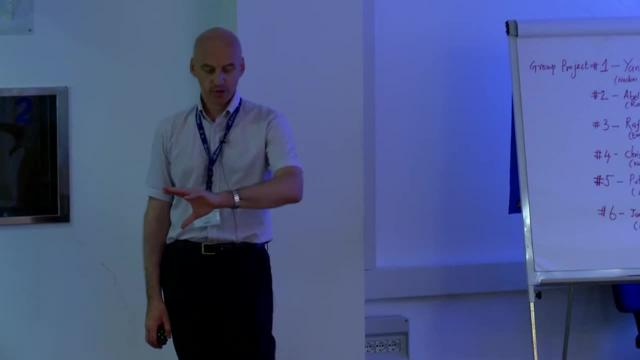 efficiently. So there are different roles of strategic plan. as the time goes through your project. All that is explained in this milestones document for research reactor project. Okay, I think I'm done with my first presentation. I would need another 10 minutes for second short presentation, but I'm ready to take. 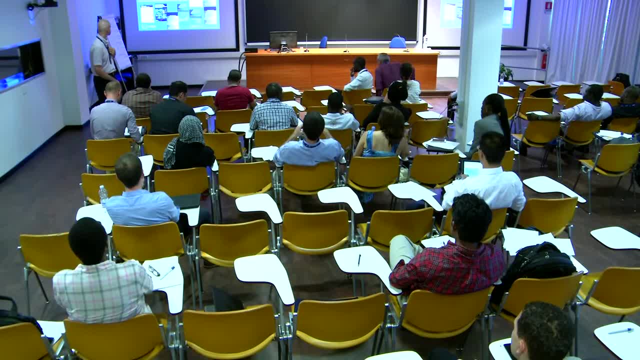 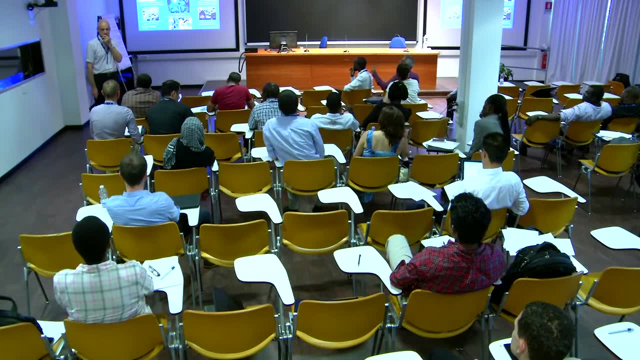 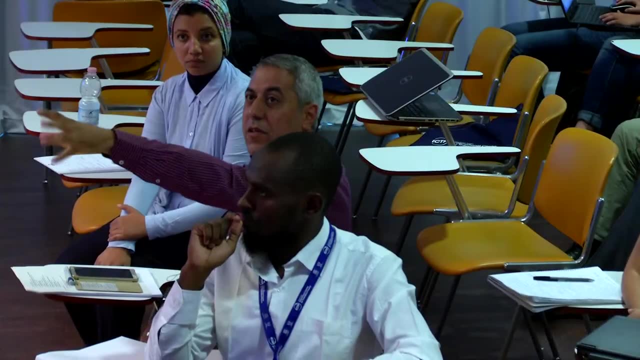 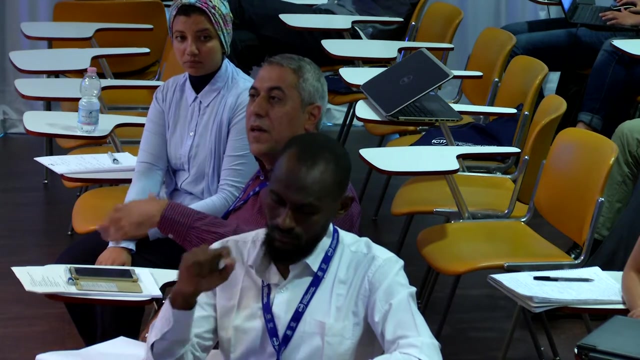 any questions or remarks? Okay, Yes For the presentation. Yes, Yes, So do you know? there's many, there are many types of Yes. I mean So how, and even for the future of the generation. 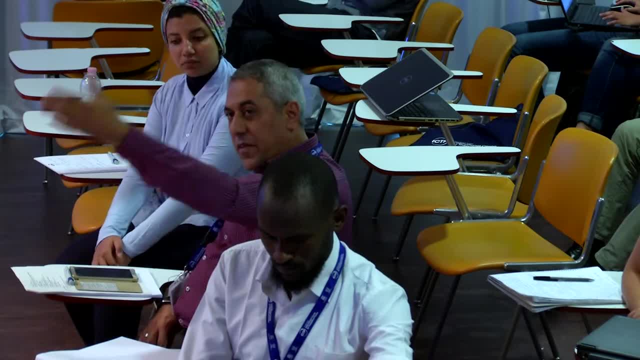 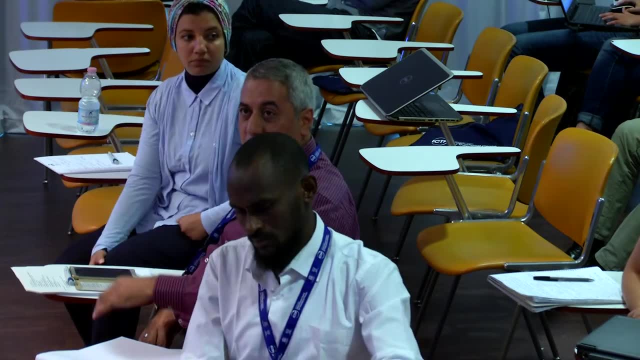 Yes, So what is the safeguard? How can they do from the design of The safeguard regime applies to any installation where the nuclear material or radioactive sources are in place. So, for example, if you have a nuclear power plant. Yes, 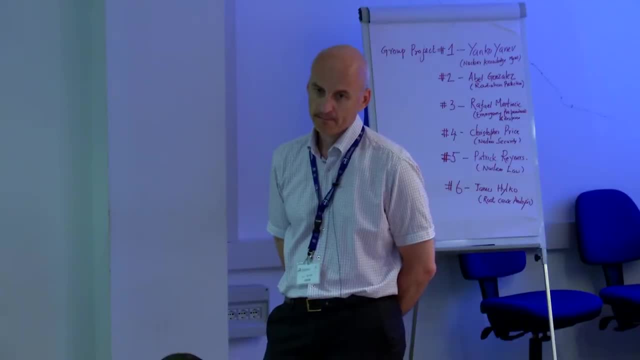 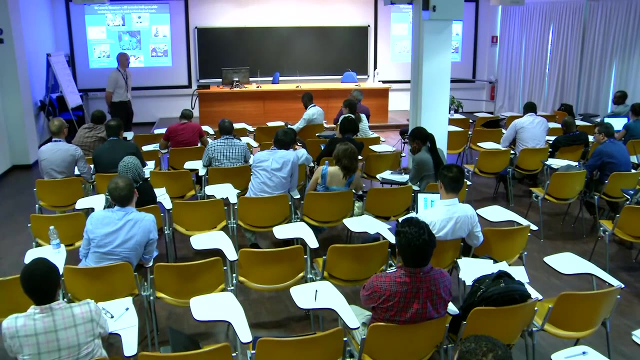 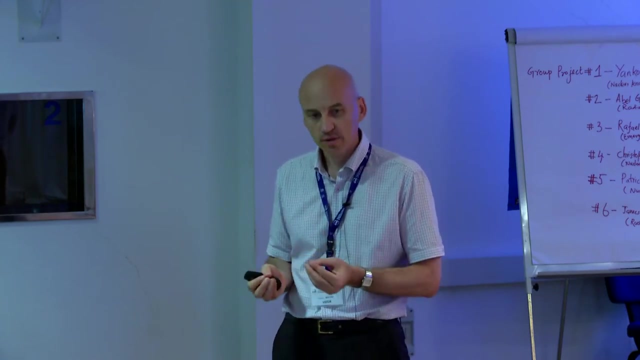 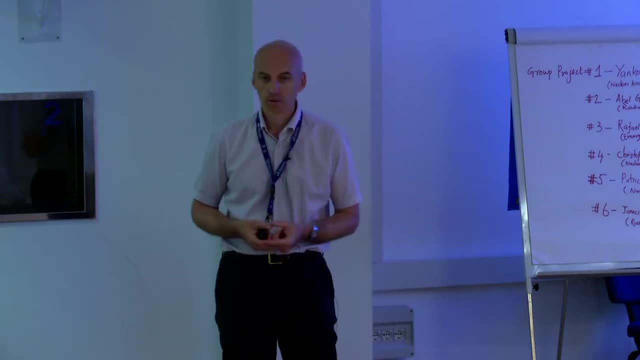 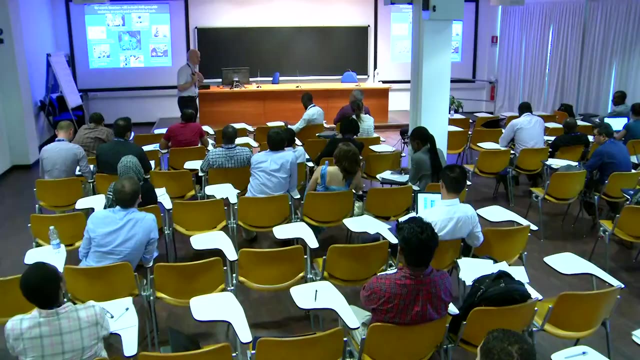 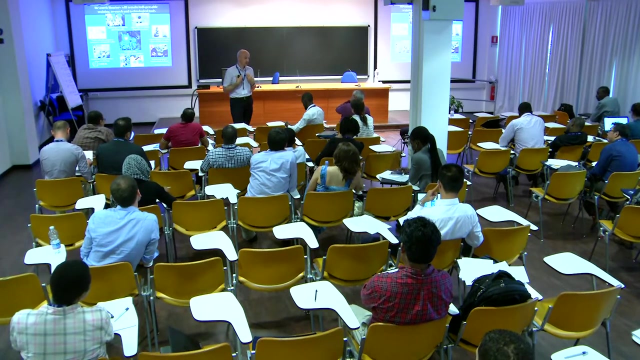 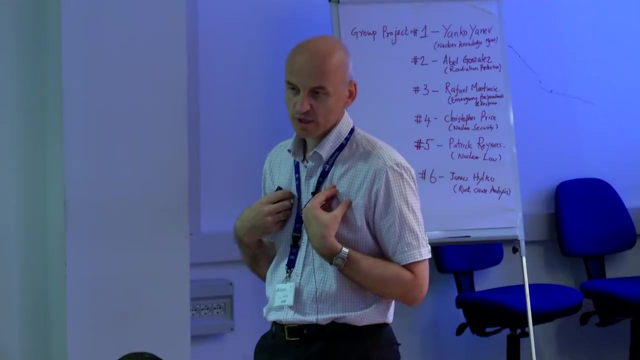 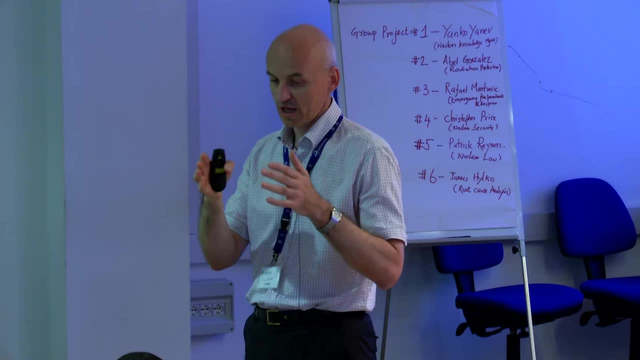 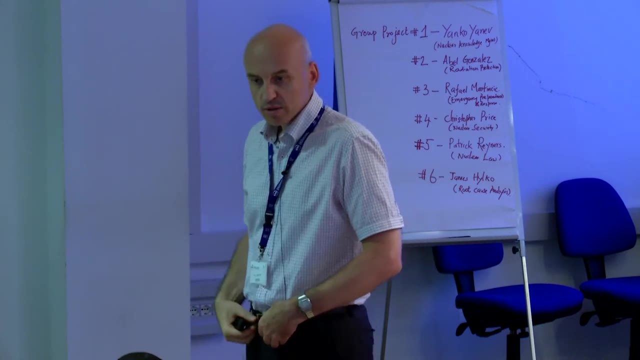 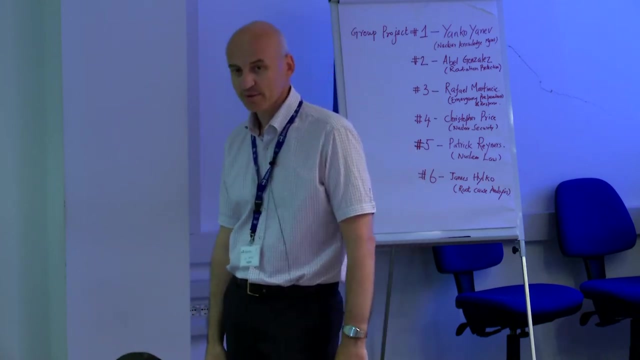 personal opinion, an even bigger challenge than the facilities where you have load and unload of the fuels. When you have liquid molten salt running all around and reprocessing, extracting fission fragments, maybe sometimes a bit of plutonium, that's a different story. 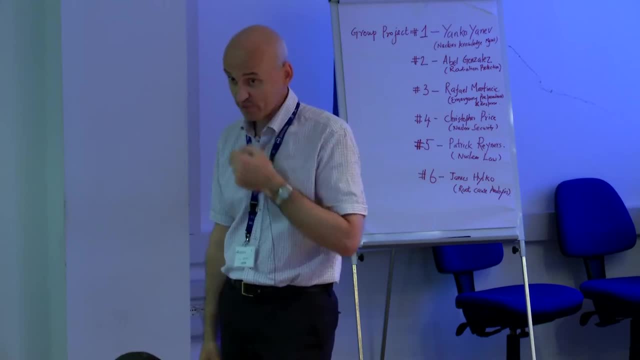 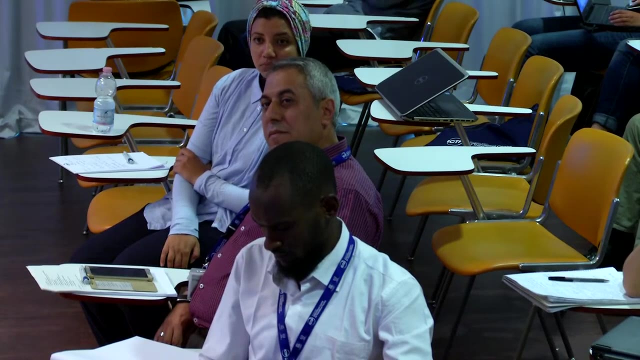 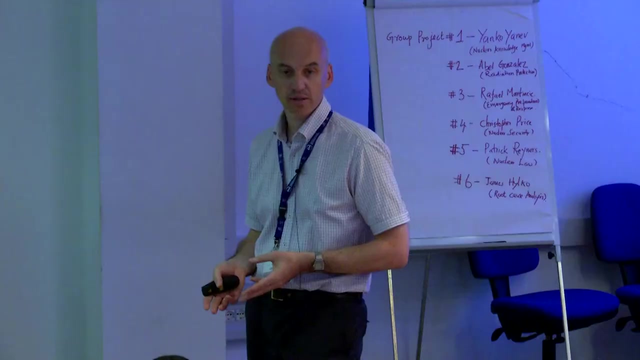 These designs and concepts, in my personal opinion, will be more challenging than we have with present technology. It brings many different features. They can operate with natural uranium, but natural uranium only from the beginning, because later on you will have closed cycle sufficient plutonium generated or 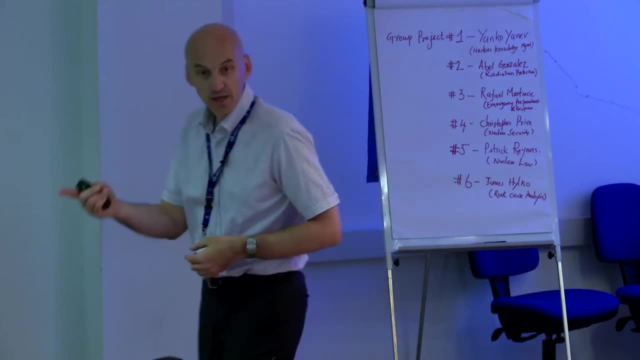 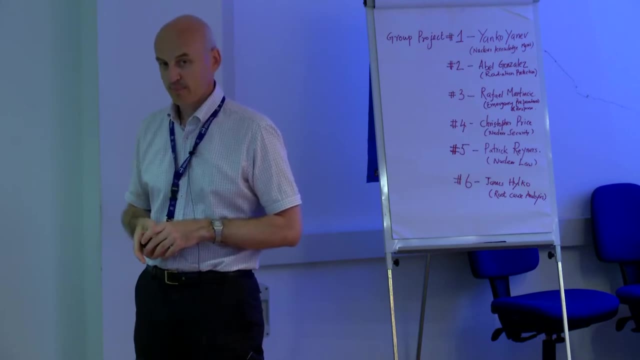 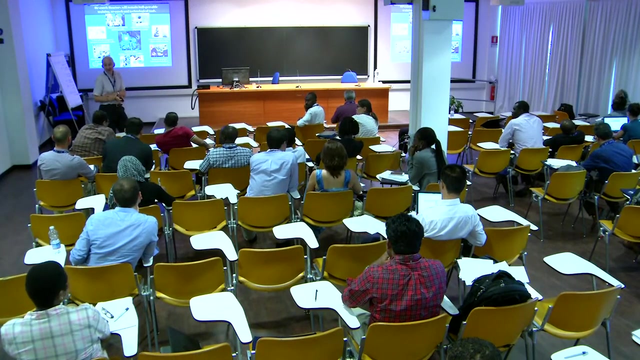 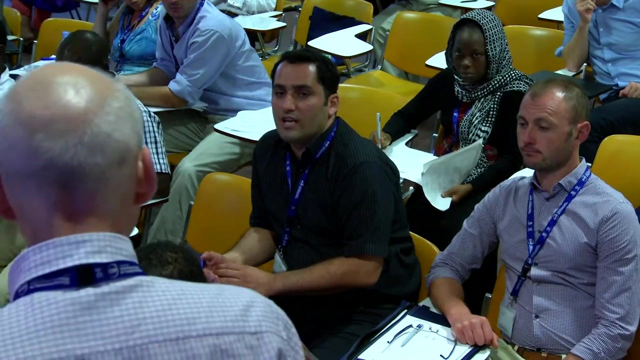 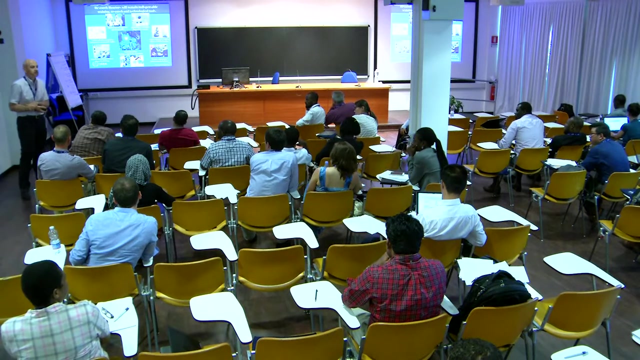 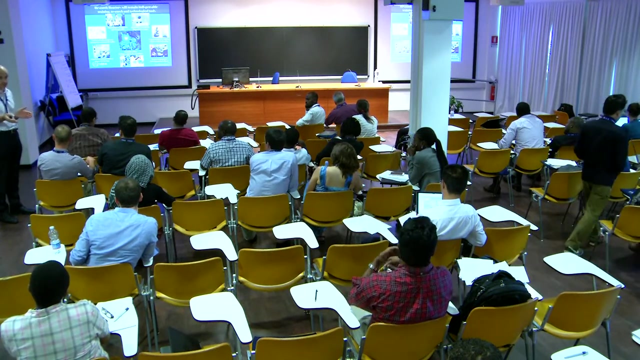 uranium-233 generated to keep the chain reaction at equilibrium core configuration. So challenges will be there. We will have more work at the agency with these concepts: Correct, Right, Yes and no. There is a challenge for the safety also with the new reactors. 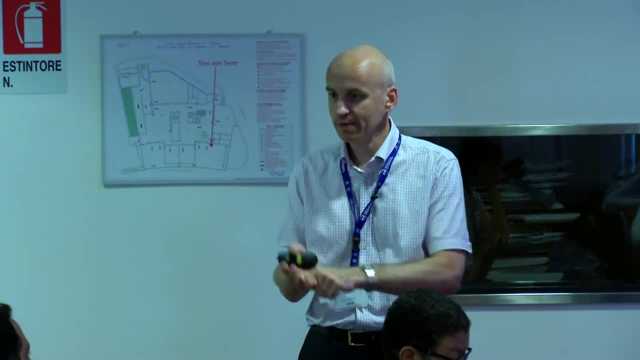 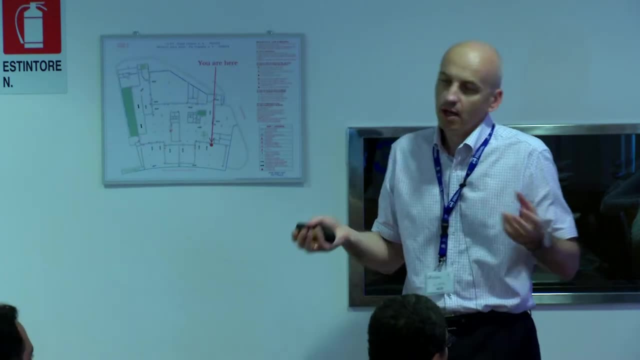 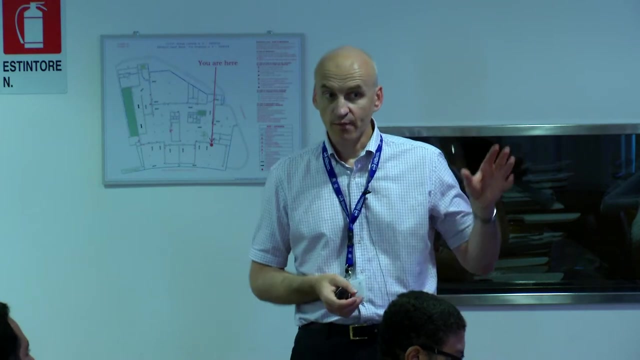 Safety, yes, Depends on a system in place, experience of the staff, design of the facility itself. So this always there's- I don't want to say challenges- Is the situation what you can control if you control properly. Now for the facilities which are old, which did not have 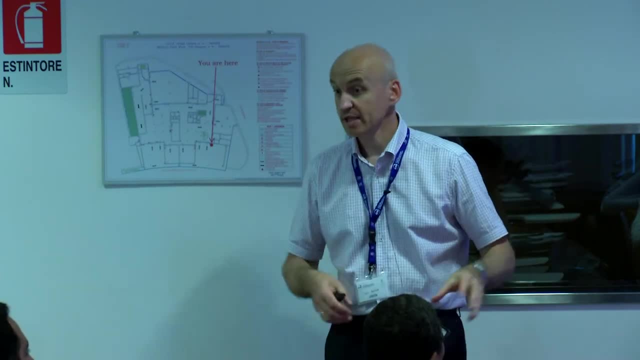 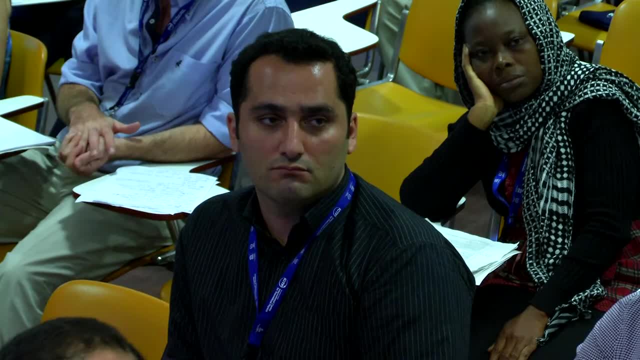 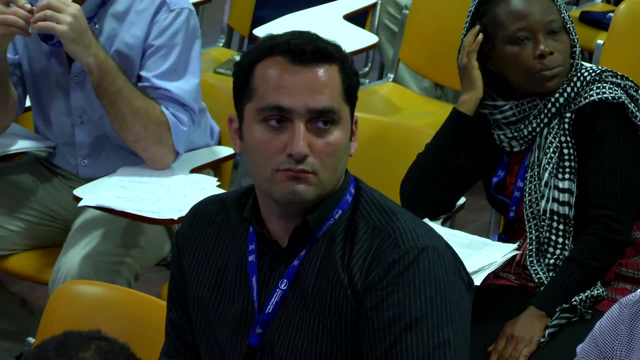 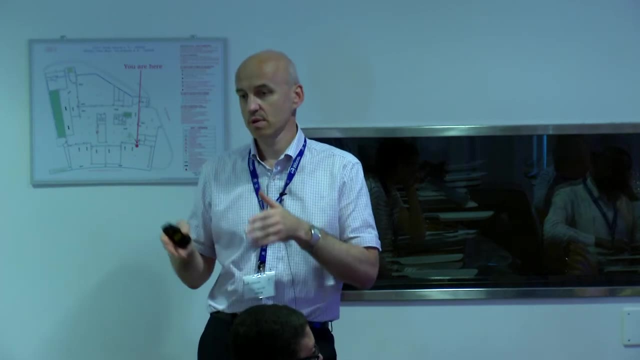 these facilities may be operating one day per week, So there are no normal shifts. Information sometimes is not properly kept. There are more challenges in such situations. I would say call facilities, But we know a few old facilities: 15 years after operation still they run more than 300 days. 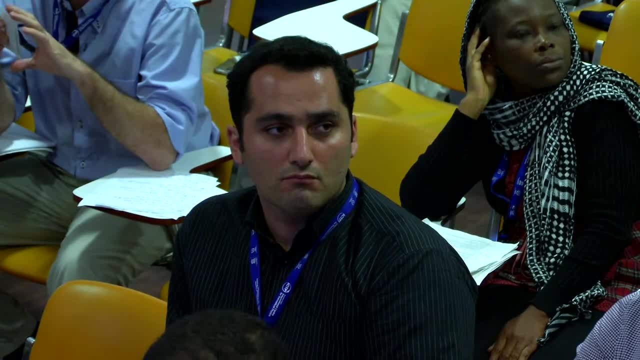 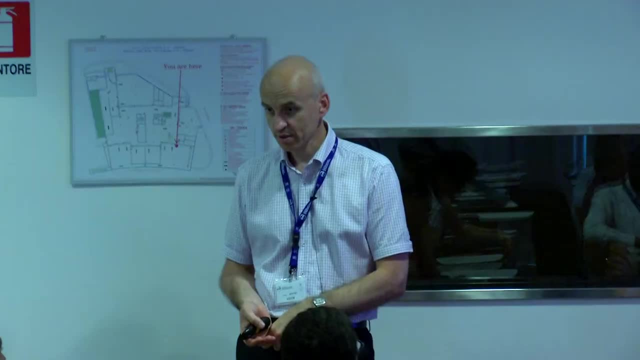 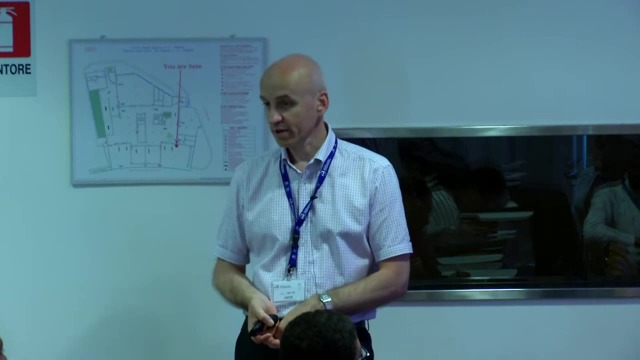 24 hours, seven days per week. today, One is in South Africa, and this is a major contributor to the world's Molybdenum-99 market. They run more than 300 full power operation days and contribute to 30% of the world's markets of Molybdenum-99, and its facility is more than 50 years old, So it's possible. It depends. You can drive an old car forever if you manage and take care of the car for a long time. It depends again. Because in some cases major refurbishment projects will require sometimes more money than the facility was built. So then it's a policy decision. You might go through the strategic plan from the beginning for such a facility and say: do I need this facility? 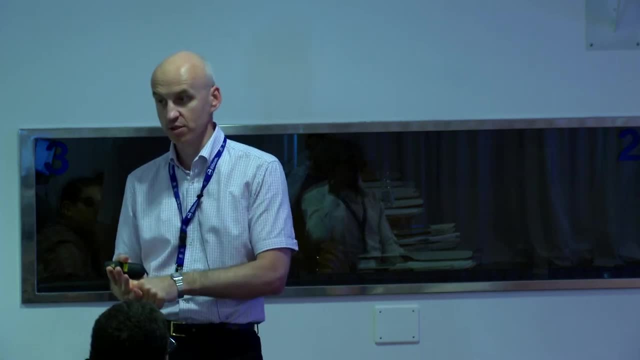 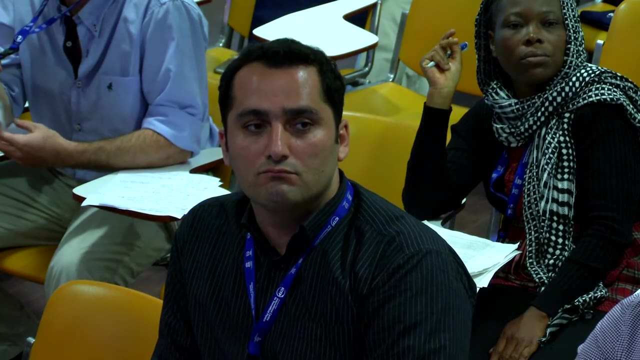 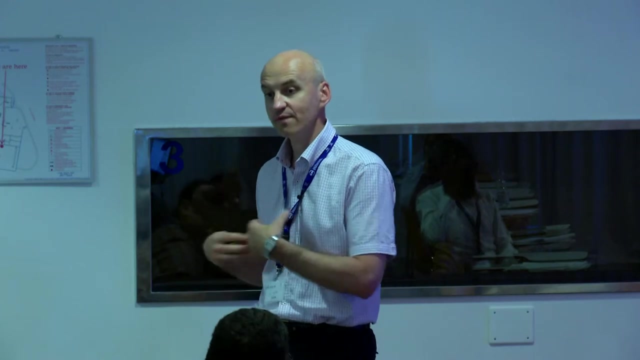 Do I have sufficient arguments to continue its operation? Because everybody knows it costs me $500,000 or $2 million to keep this facility- including staff salaries, just like that- in a safe mode. not necessarily operational right, But do we need, can we justify this spending in some cases? 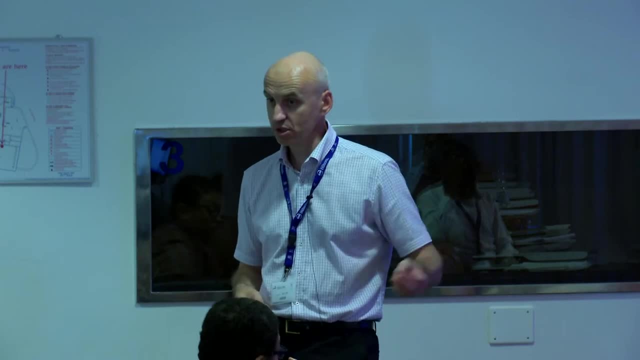 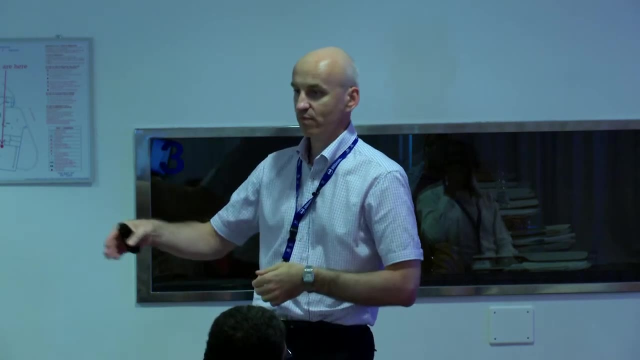 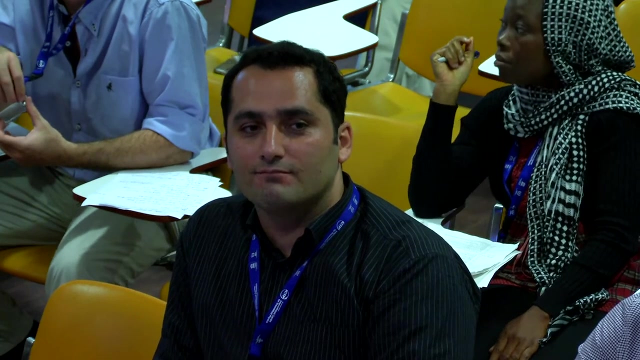 In some cases yes and no, And then decision can be: OK, we go for refurbishment, We update it, upgrade it and use it properly, starting from year plus three, or we shut down the commission. It's a strategic point. 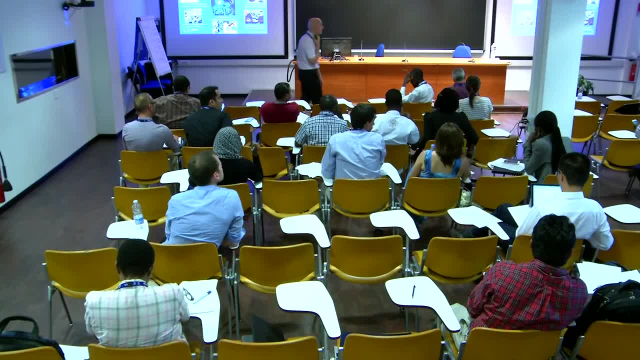 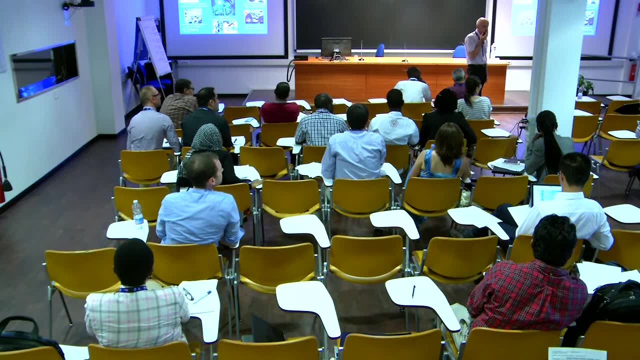 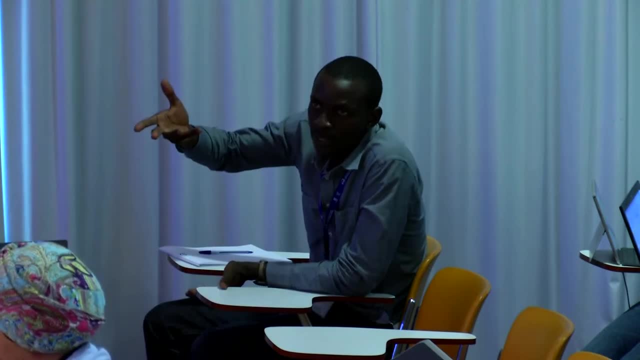 Yeah, Thank you for your clarification. My question is more of an indication in terms of the, I would imagine, take an example of. We advise them. what experience, what are the challenges, What I'm imagining. I want to buy a car. 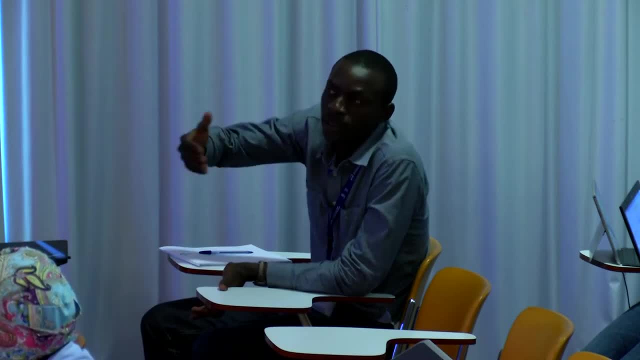 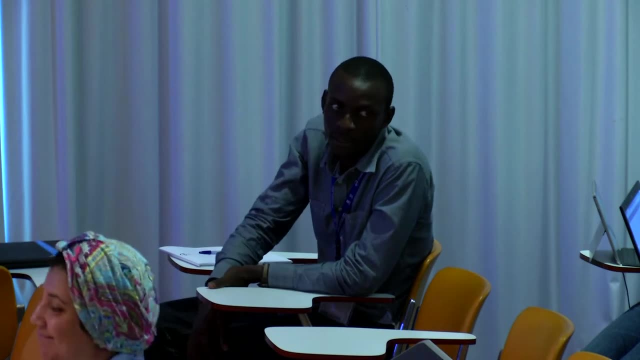 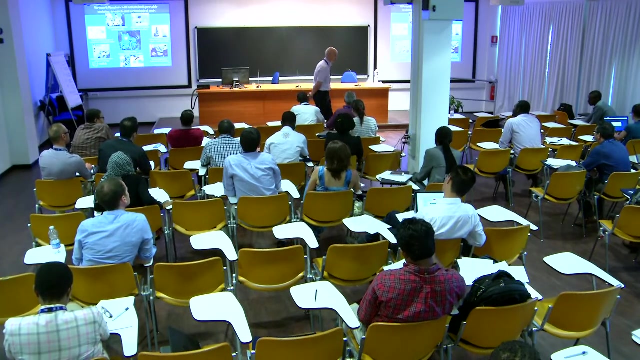 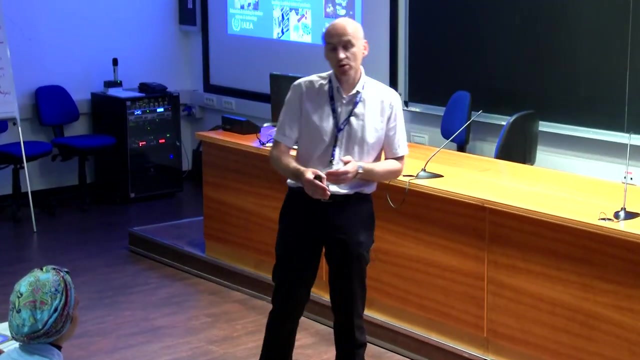 I don't have all that big money, But then I'm tempted to buy a motorbike. Yes, it's a very similar experience. It depends for which purpose you would like to have a research reactor As a toy For doing some experiments time to time, or country goes for nuclear power. 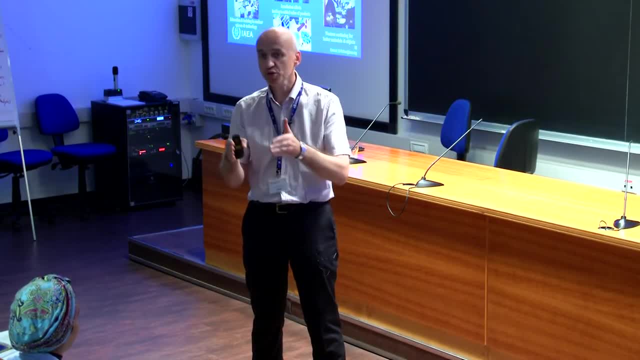 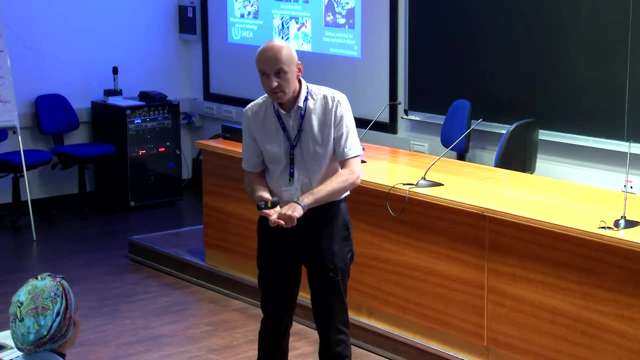 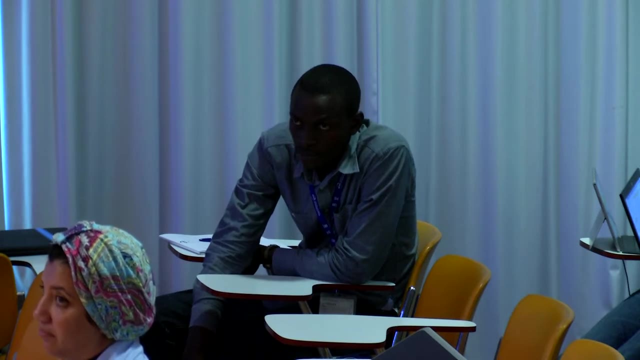 And I see this facility well designed to train nuclear engineers, safety authority specialists, protection specialists, future managers, et cetera. So if I define the role for this particular purpose, I will design a reactor of low power, low operation costs. Operating team one shift And I will spend most probably $50 million for reactor And I will spend every year for this type of reactor maybe $200,000, $300,000 per year And my utility company will pay for me because their budget is much bigger. 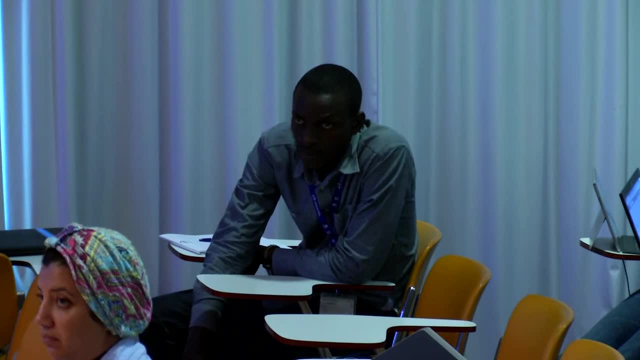 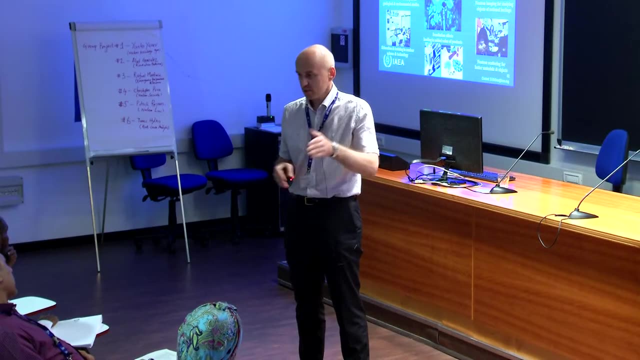 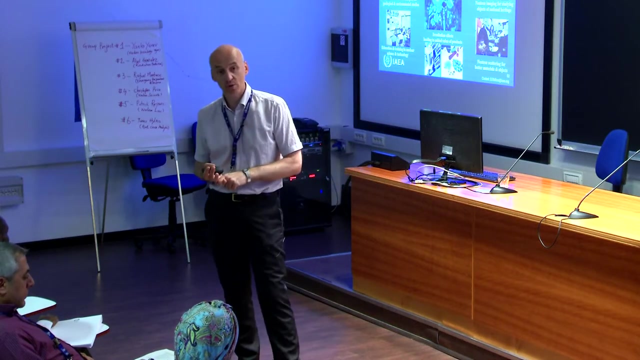 And they see the added value for their human capacity building in this facility. This is a hypothetical scenario. Now countries don't like one single use facilities. They say this research reactor, even at this small power, can do much more. It can do neutron activation analysis. Analysis of one sample on commercial level costs you $50.. So if you analyze, typically reactor can analyze easily. if there is a market up to 1,000, 3,000 samples, you see how much you can earn. But remember what I said in the beginning. 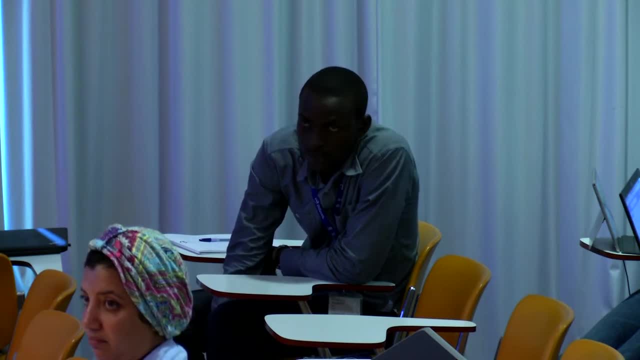 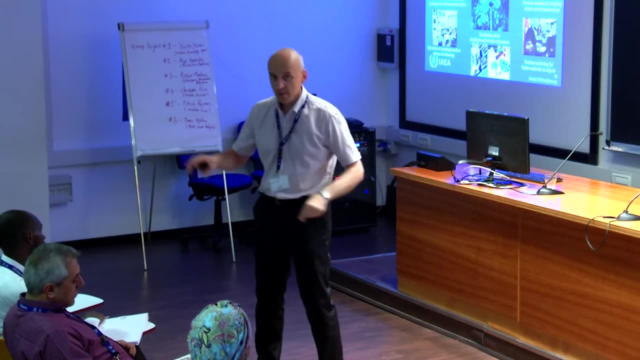 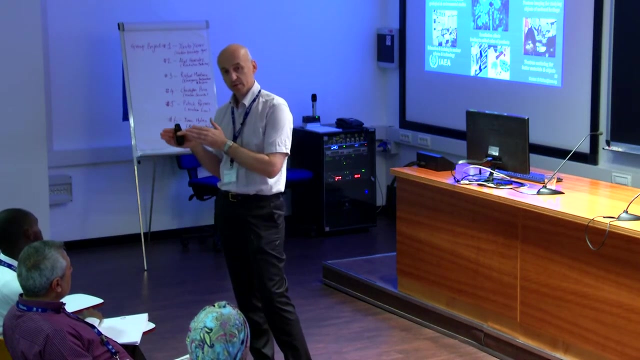 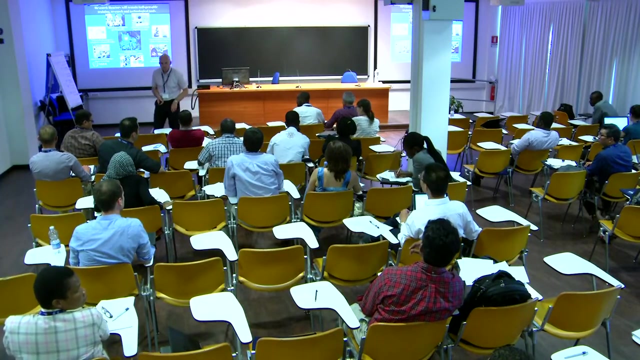 Research reactor will never generate sufficient revenues to cover operational costs. I'm not speaking about capital investment costs: shutdown, decommissioning and final waste storage facility. You will always require government support and funds. Yes, New generation Jordanian. 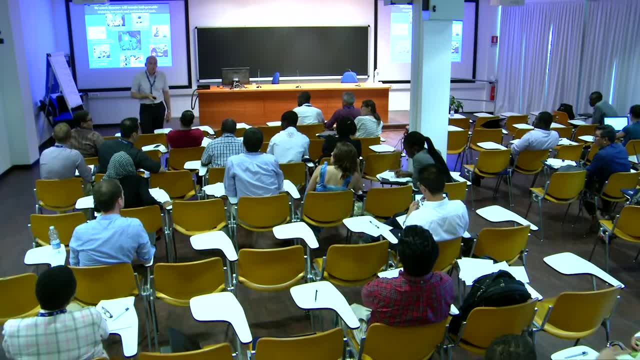 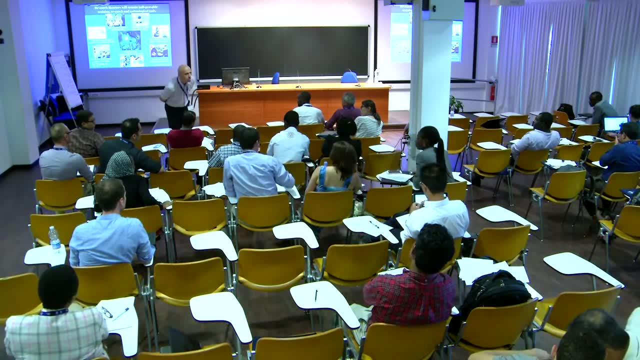 Jordanian. Yes, What? Sorry, If it has, Of course It would. It depends where in the reflector you place your pneumatic system: Closer to the core, closer to the fuel element or more further away in the reflector. 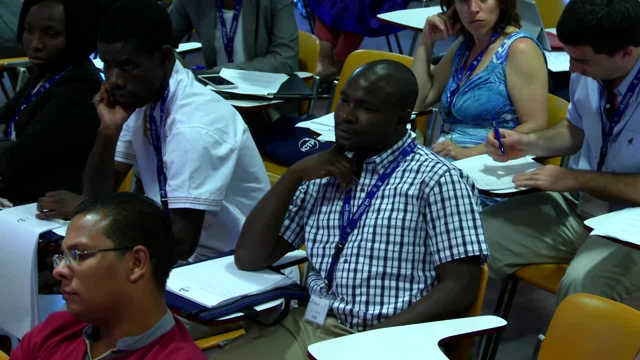 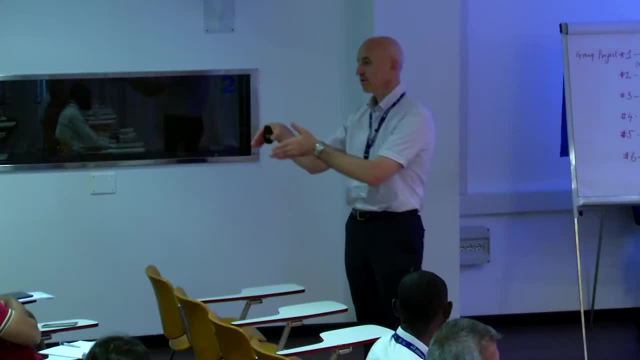 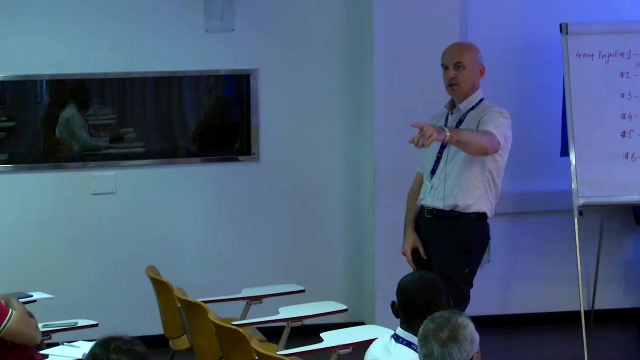 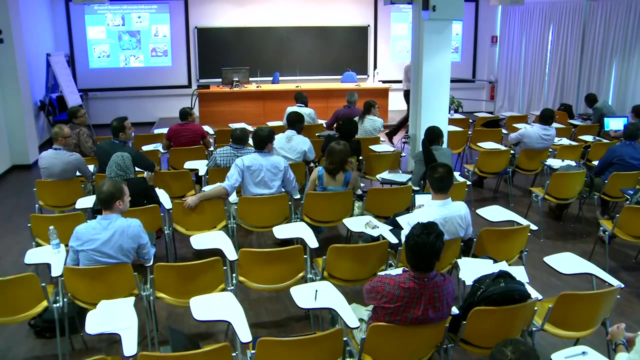 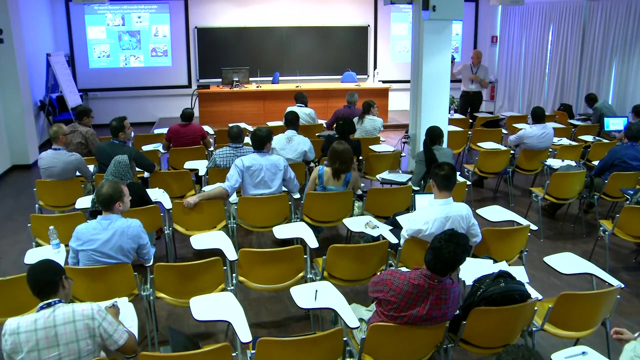 And then moderation rate is different and you will have: Yes, It's pre-designed. He is far-away, So I can see him hardly, so please yes. We cannot do better than today can be done by just exactly what. you reach the limit: 100 megawatt. Because you cannot. for the same reason, what is limiting factor is power density. So to have 200 megawatt reactor, you explode your core. Geometrically it's much bigger Power. density is lower, So you can have more power, but you will not increase in the flux. So that's the thing. And you do neutron recalculation. so you know this one. Why are you asking the question? 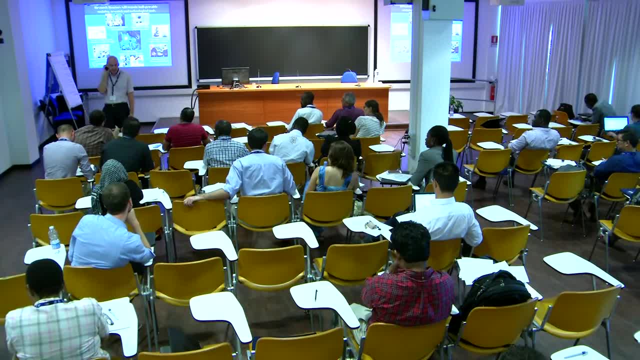 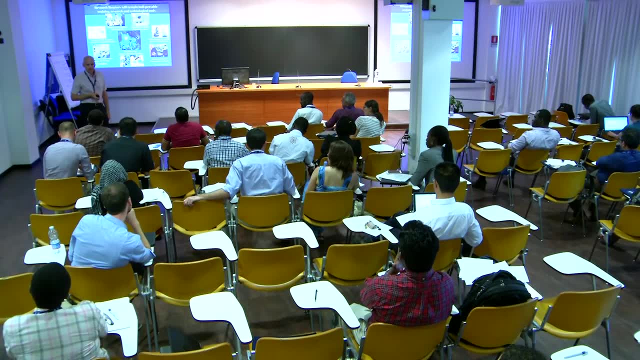 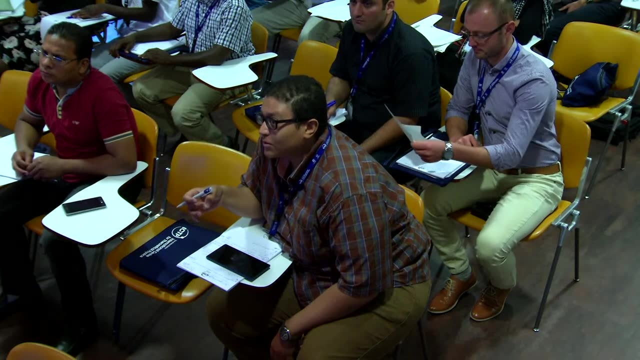 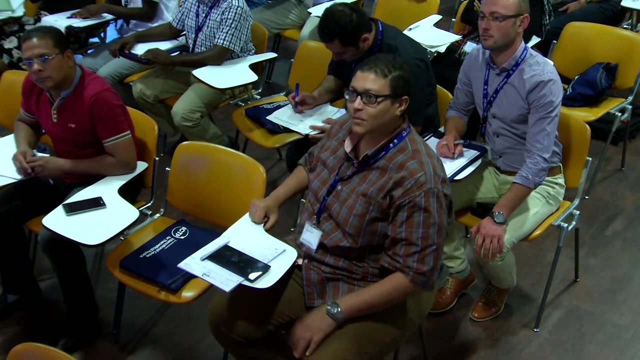 Yes, Correct. Really, how are they going to enlighten the reactor? To my best knowledge, I'm not nuclear engineer, I'm nuclear physicist. You need external source coming from americium: beryllium, plutonium, beryllium. 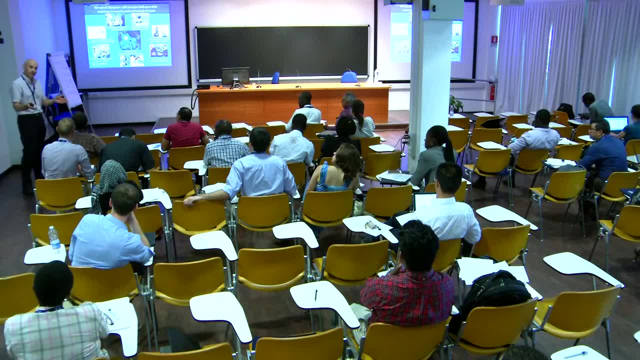 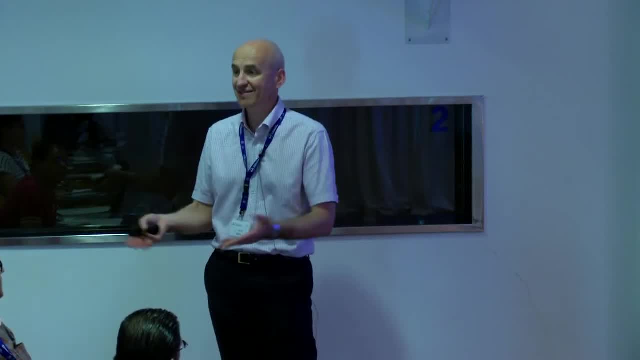 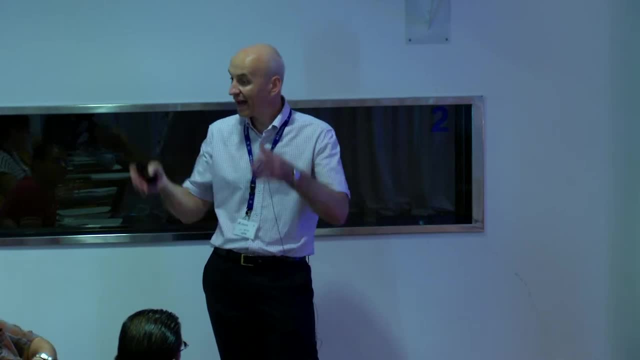 for this kind of technology, Or they might have a spent fuel element which can serve as external neutron source, But you need external neutron source to enlighten. So if they spent fuel element and has sufficient high level actinides which are spontaneous fission emitters. 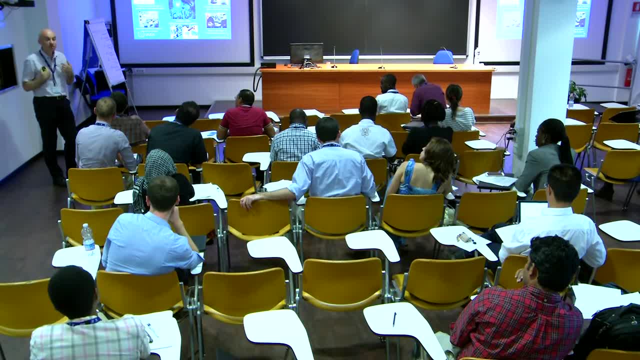 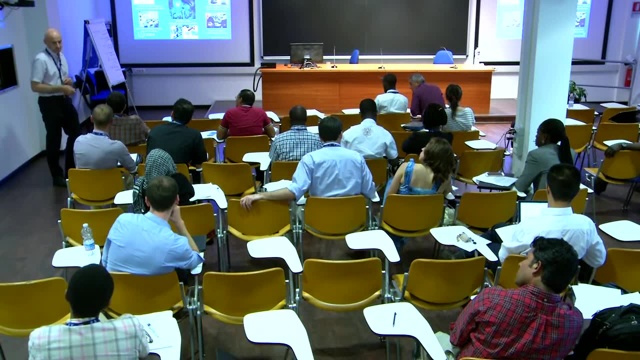 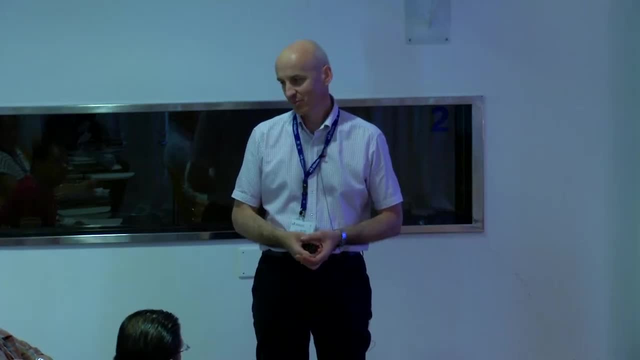 you might enlighten the reactor? Only physics thinking, not engineering thinking. So I would say they would need external neutron source, Otherwise they cannot start the facility. They have some secrets. No Yeah, This is Russian design for Egypt. I can check. 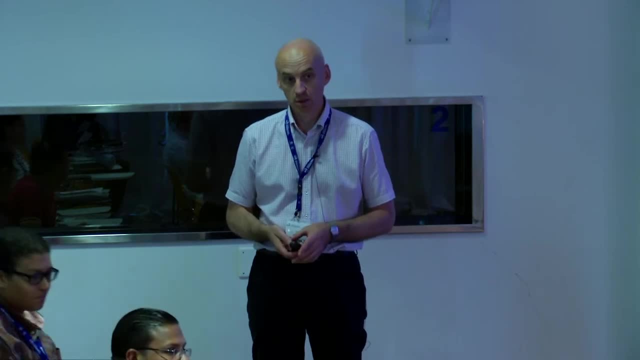 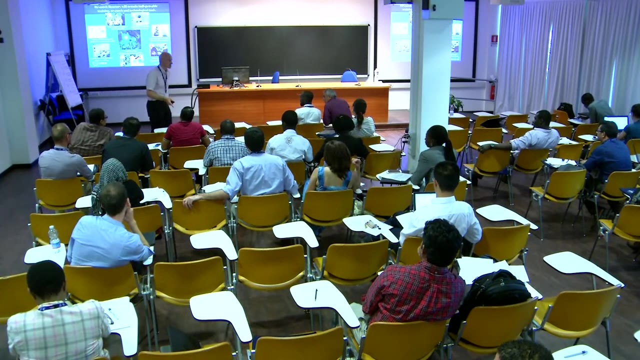 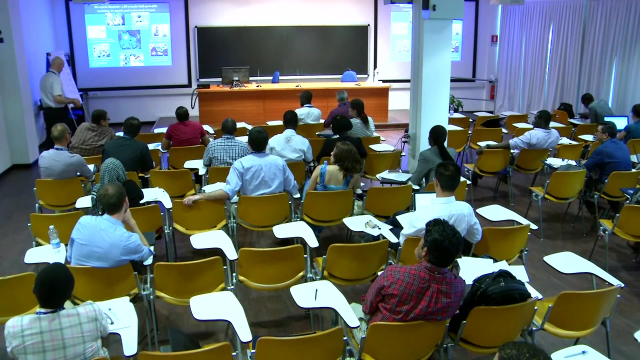 Maybe I can give you the answer, But at the moment. But I think they're external, Should be, Should be. Maybe this is internally external. All right, I think I need. I have five minutes for the. I'm not going to finish the next presentation. 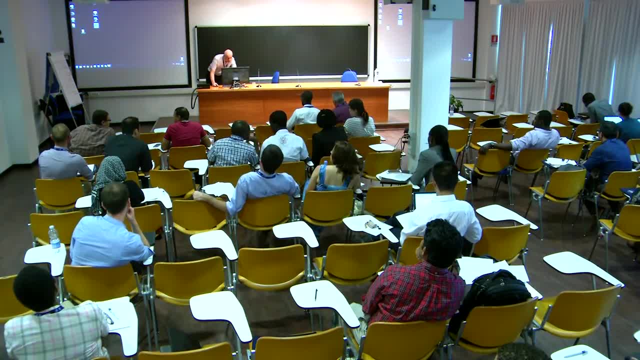 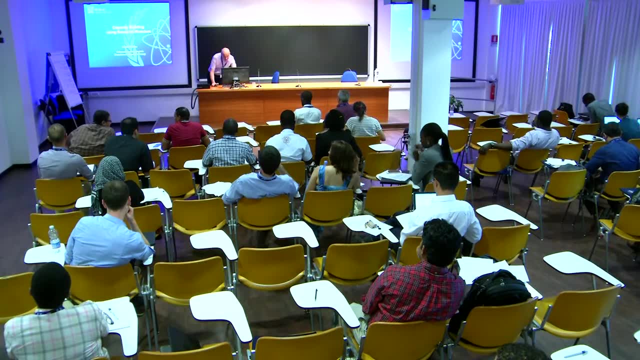 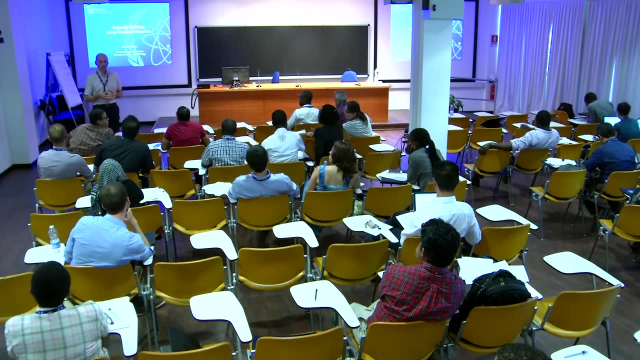 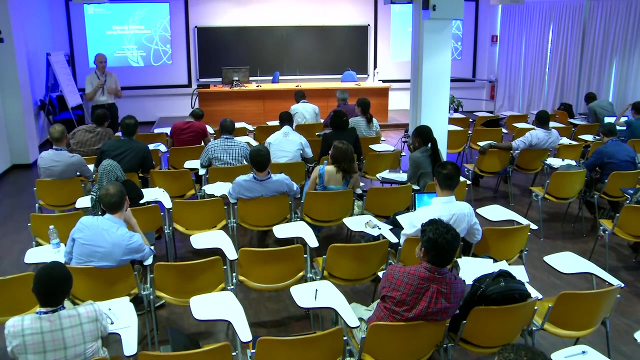 Thank you That time. I think this lecture I hope reached the objective what I said. I had some challenge to keep you awake And to show you that research reactor can do many things except electricity generation. I think this is done more or less. 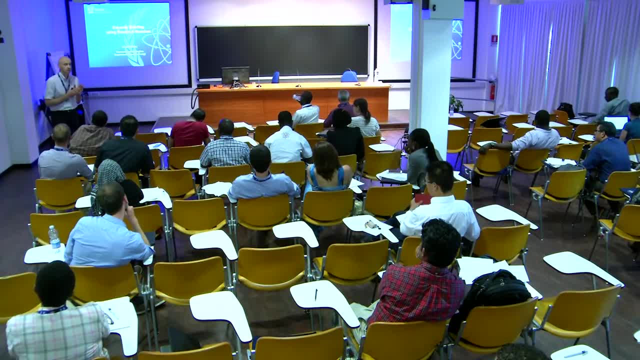 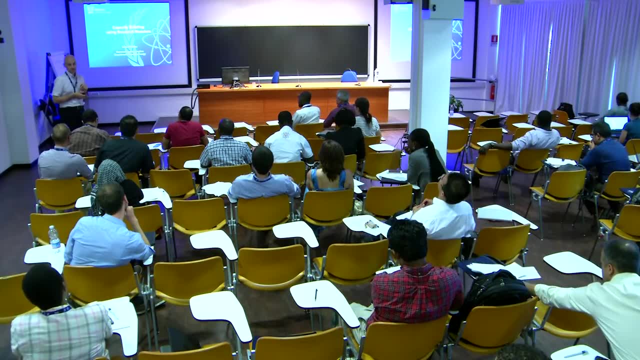 So what? I'm going to say that we have four major actions at the agency where we help member state to use better research reactor And it's one of the major For capacity building, And I will just highlight these instruments. And this presentation, I believe, comes with an old package. 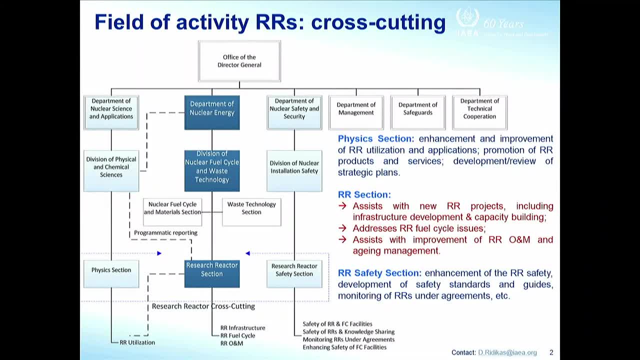 So you can study that Or you know. this is just about cross cutting research, Shackle the complex machine. so you need to take care of utilization. That's Department of Nuclear Science and Applications. You need to take care of the reactor itself. 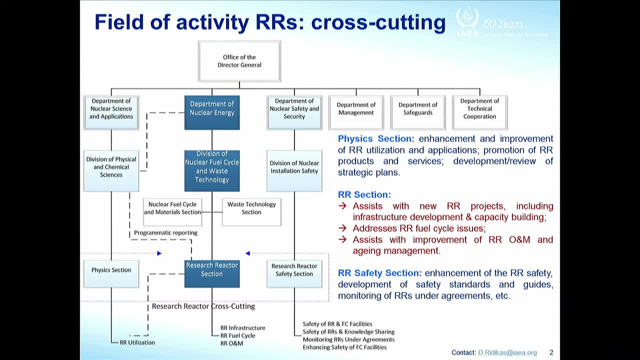 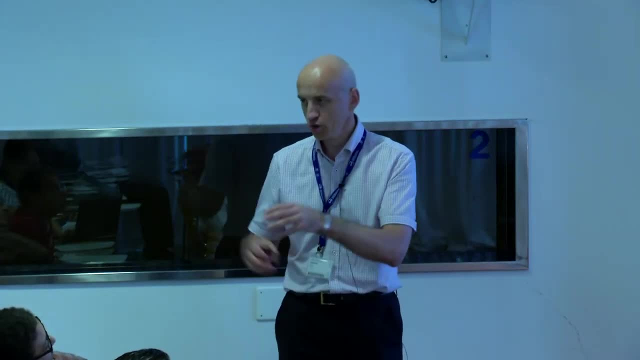 Operation, maintenance, Fuel management infrastructure. That's within the Department of Nuclear Energy and Safety, So that's within the Department of Safety and Security Security. I forgot. Now everything has to be said: safety and security. This is a new inseparable term within the agent's language. 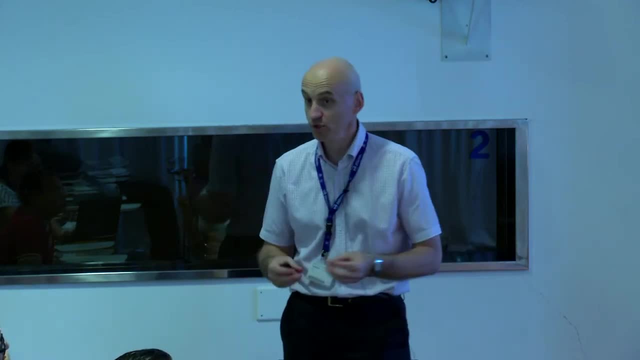 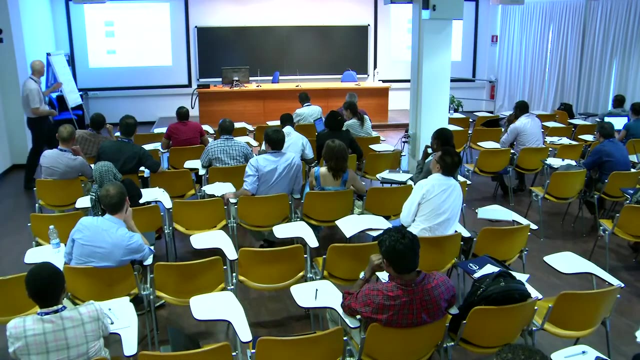 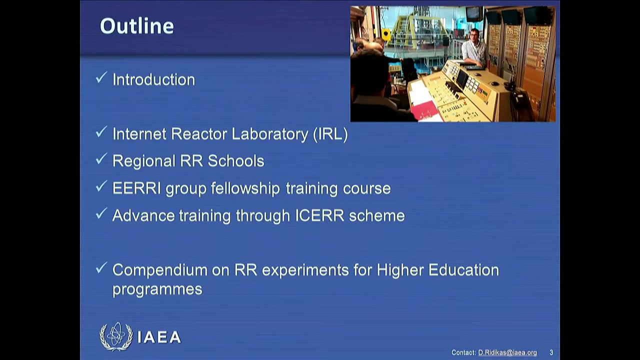 And of course, safeguard, because you have nuclear material. So a research reactor is like NPP, where you have so much different areas and technical expertise. That's why for research reactors we created a cross-cutting group all along the departments within the agency. 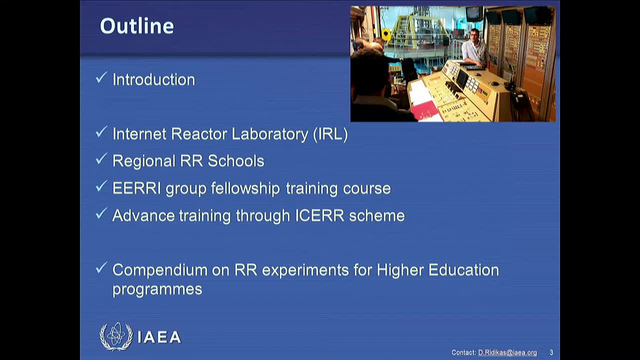 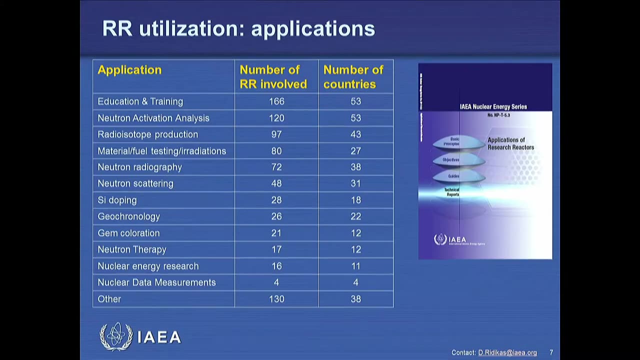 I wanted to introduce you to Internet Reactor Laboratory Regional Research Reactor Schools, Eastern European Research Reactor Initiative Group Fellowship Training Course, advanced training through the international centers based on research reactors. This has been shown. this has been shown. this has been shown. 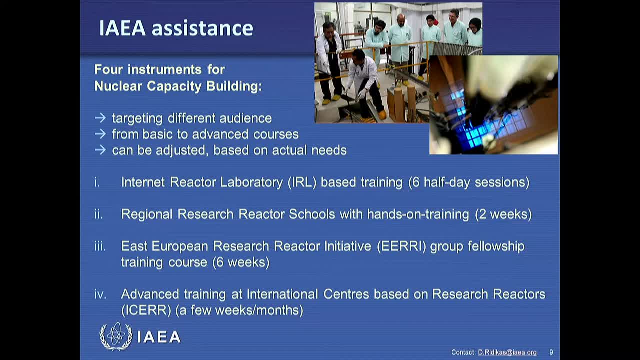 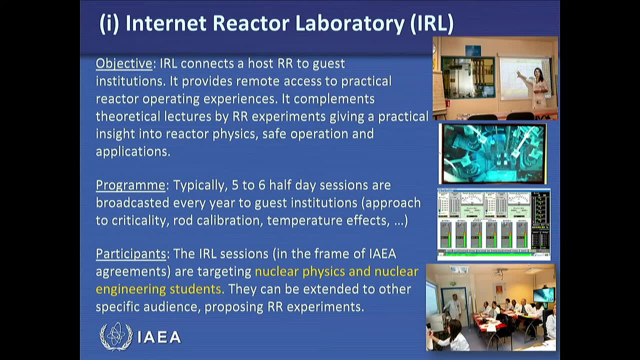 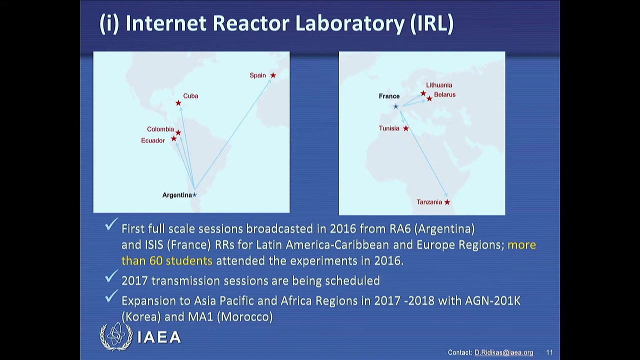 Again these three main instruments. Very quickly. I explain you the concept of Internet Reactor. Reactor is there in one country, Students are there receiving video conference and also signals to perform the experiment. Where we are standing with this project We are running successfully since last year two host organizations. 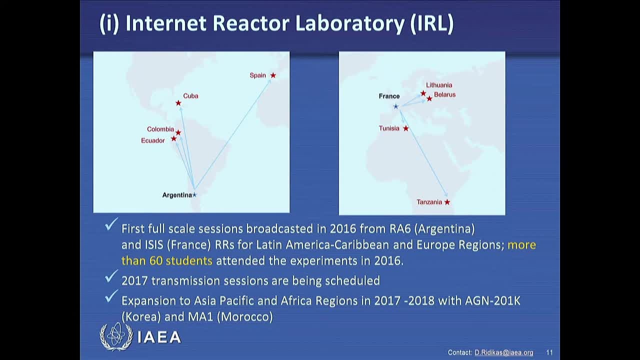 In Argentina, Research Reactor, And in France, Research Reactor, And they are delivering course on periodic basis to Europe and Latin America. These courses are in Spanish And here to Europe and to Africa, So typically simultaneously we can offer the course. 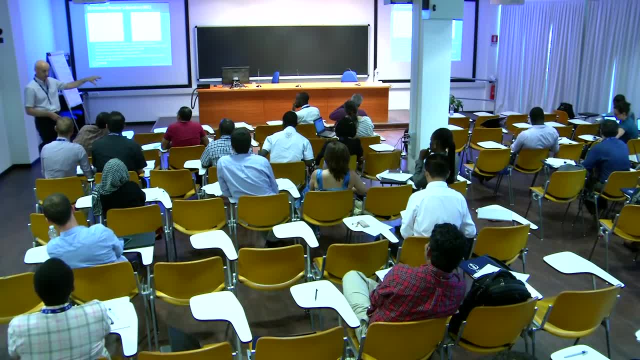 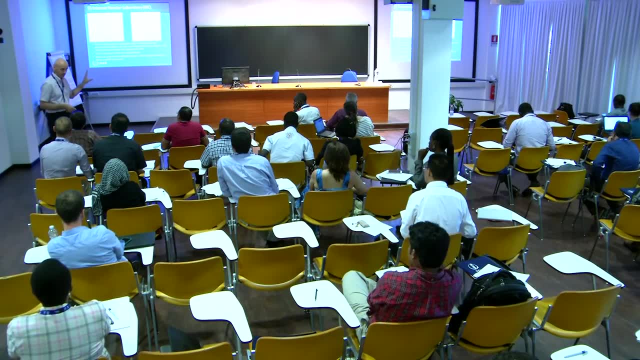 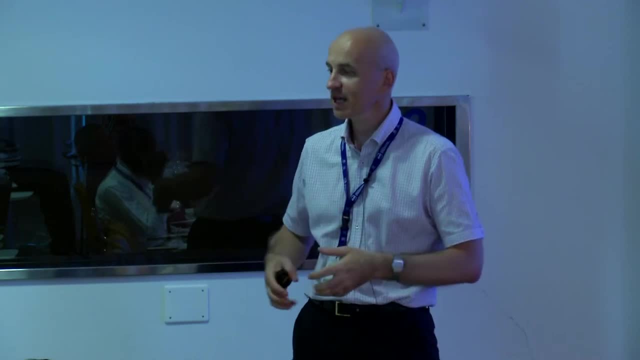 from Research Reactor experiment to four or five guest institutions. That means class of 20 students Four times 80 people are watching the experiment and participating in experiment. This is what we call efficient way of teaching. It's not the same like being on a reactor and doing experiment. 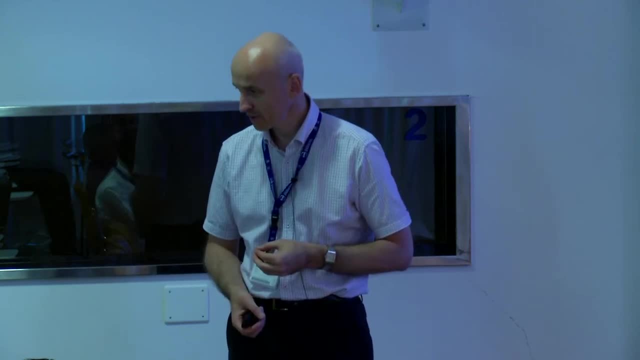 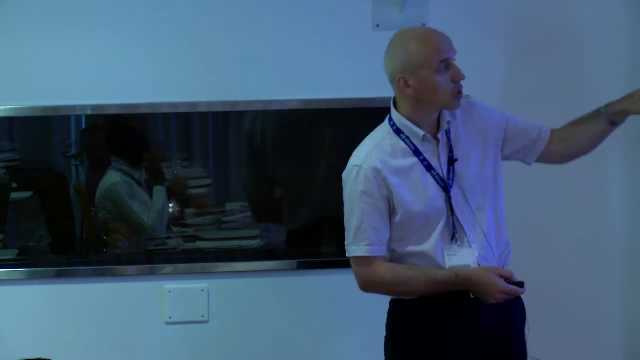 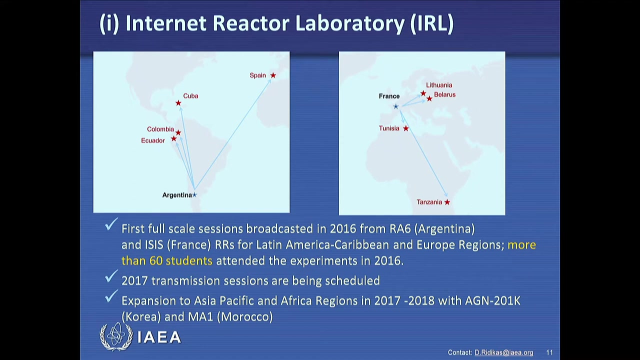 But you also can count how much money we save in terms of investment for sometimes near the same outcome. We are planning to work with Korea, So we can cover Asia Pacific region, And we are planning to work with Morocco, So we can cover African continent. 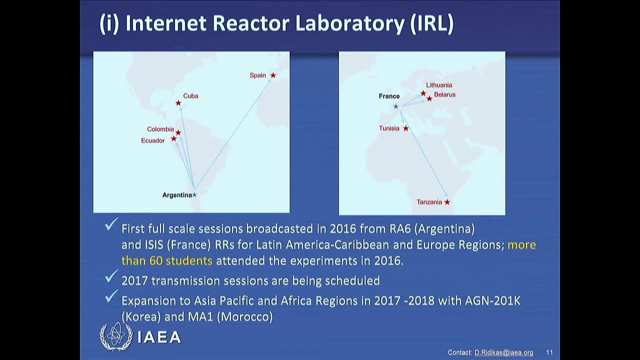 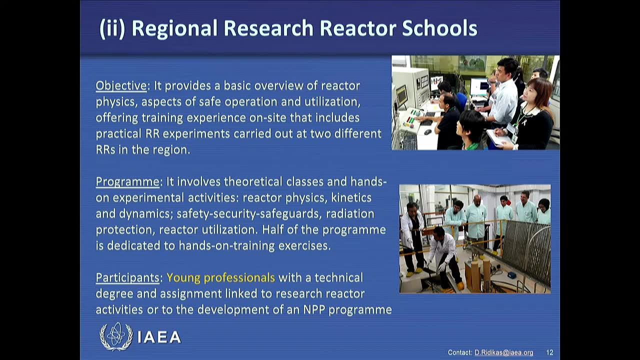 So French reactor can concentrate on Europe. Okay, So that's our future for the IRL, We promoting and assisting organizing regional reactor schools. The idea is that in two weeks course up to 15 trainees can go to two different reactors in two different countries. 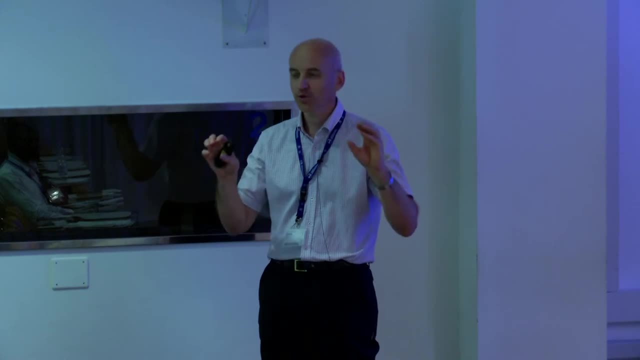 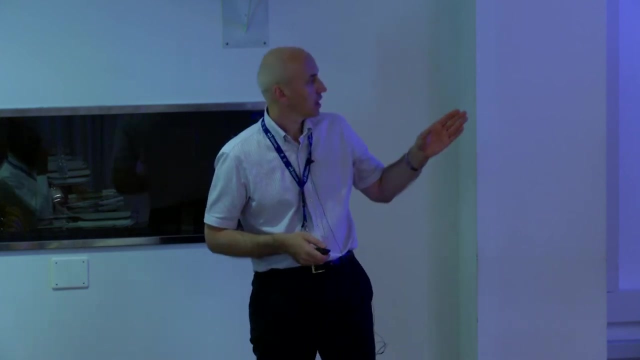 Somebody said to me: Research Reactor have so much designs. Even for the same design, you will notice that the same experiment is performed differently. That's why it's Research Reactor. Yeah, So we are successful to bring students to Safari 1 in South Africa. 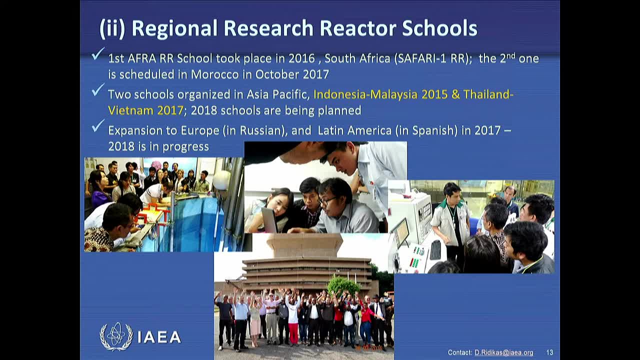 where we organized the first Afra Research Reactor school. Next school is scheduled in October in Morocco, So we're bringing students to another reactor in Morocco. We had two schools in Asia Pacific- Indonesia, Malaysia. one week in each country, A different reactor 2015.. 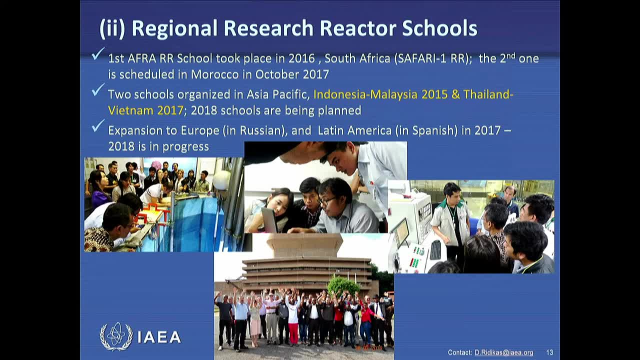 Thailand, Vietnam this year And we're planning the course for 2018.. Most probably coming back to Indonesia and Malaysia, We intend to expand this kind of hands-on training for Russian-speaking countries in Europe in cooperation with Russian Federation, and in Latin America and Spanish. 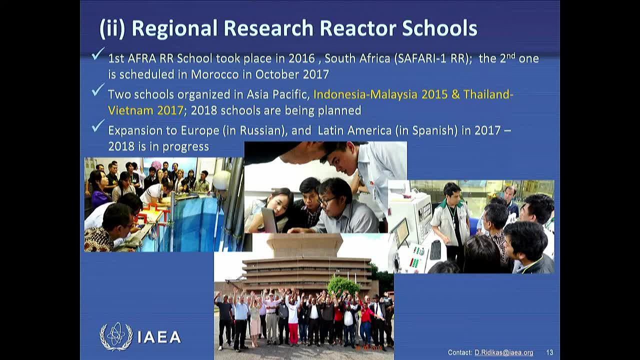 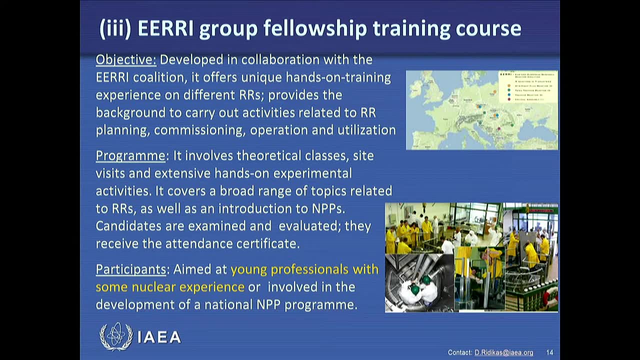 These are real hands-on training where students go to reactor to perform experiments, etc. Eastern European Research Act Group Fellowship Training Course. this is advanced course. It's six weeks course compared to two weeks course, where you go through everything what is needed for the future Research Reactor team. 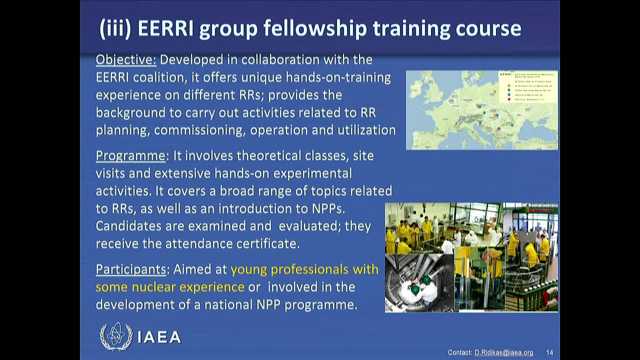 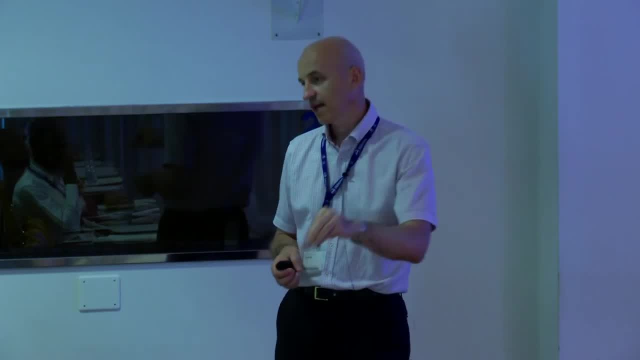 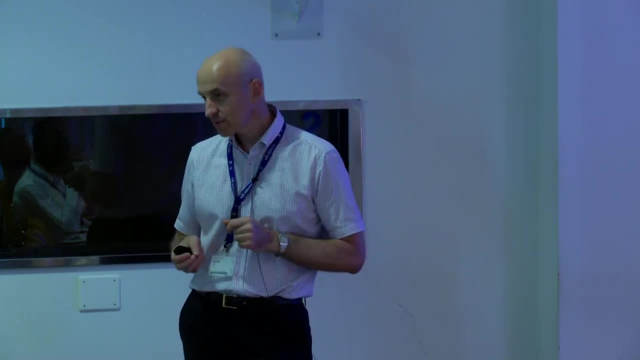 Yeah, It goes from theory to experiments: operation, maintenance, control, fuel inspections. some part of safeguards is covered: safety, security, etc. So this is very comprehensive course, typically for the future Research Reactor operating team In six weeks, at least content-wise. 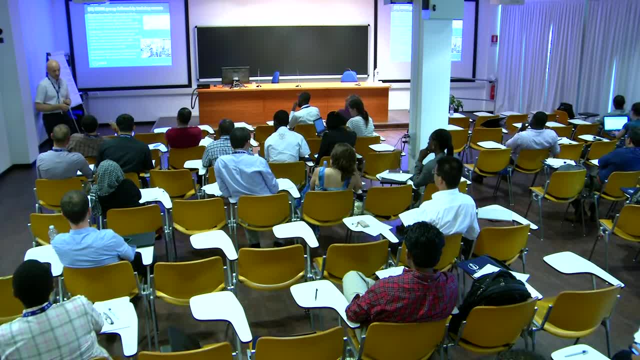 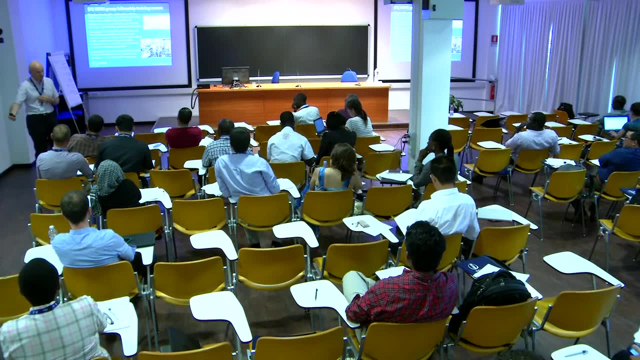 you will experience what does it mean to work at Research Reactor? absolutely Now, volume-wise, you will need much more. You might need maybe one or two years, depending on your background, to be part of the team, including receiving license as a licensee. 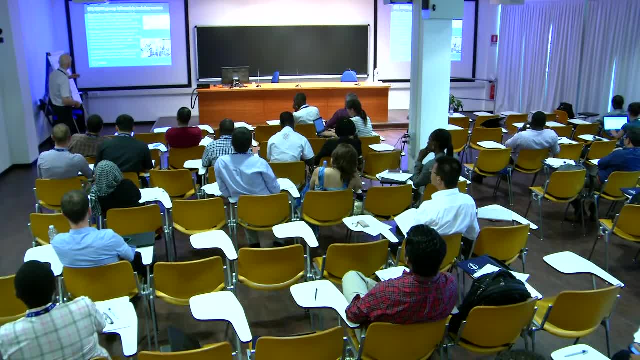 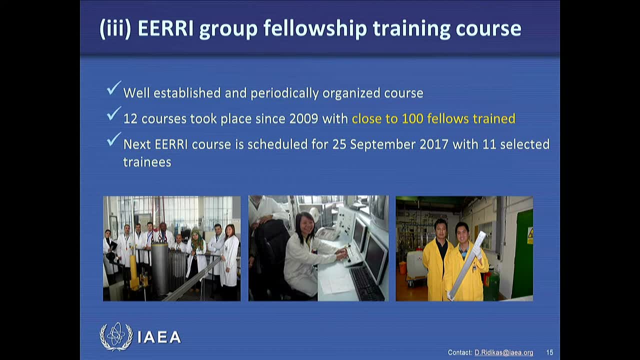 for Research Reactor operation. So this course has been organized since 2009.. We in total- because this is hands-on, we can accept maximum up to 10 trainees. We train close to 100 fellows And the next course starts. 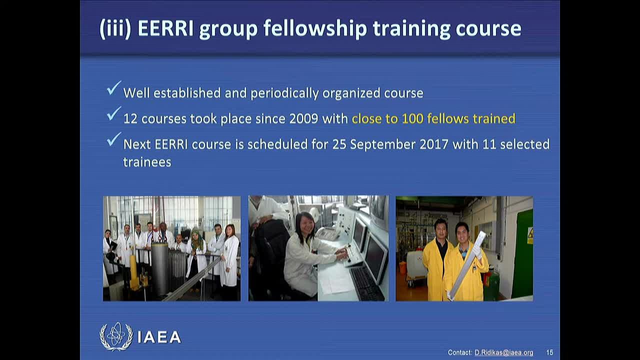 we just finished selection. 11 trainees are going to Triga Reactor at Atom Institute in Vienna and Budapest Technical University Reactor in Hungary, in a combined course for six weeks starting on 25th of September. We have created and started designations. 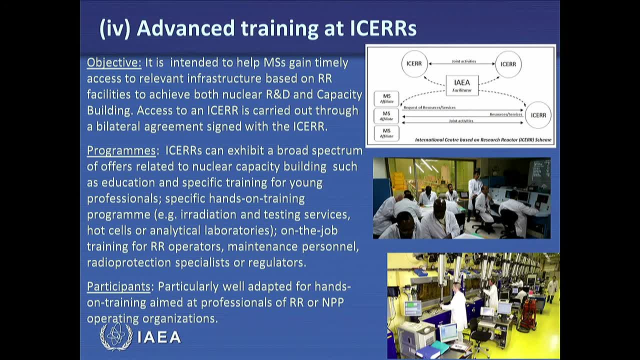 of international centers based on Research Reactors. So these are capable facilities which receive a recognition from the agency that they are state-of-the-art facilities as long as it comes to nuclear technology- Not nuclear technology in general, but based on Research Reactor. 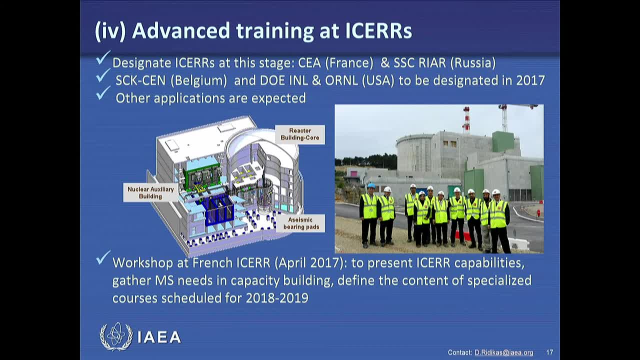 So we have given this recognition to CEA in France and RIAR, the Russian Federation, And we are about to recognize Belgium Center and two DOE labs in US- Idaho National Lab and Oak Ridge National Lab, where the Research Reactor is a key component. 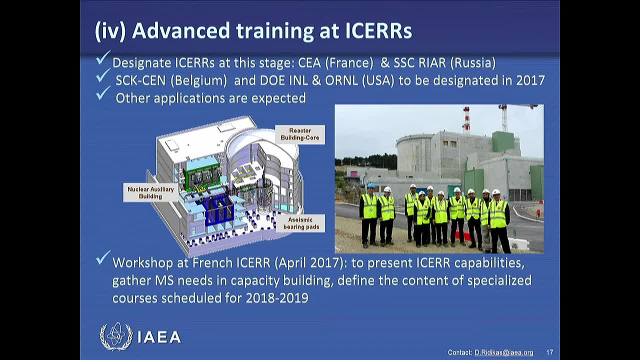 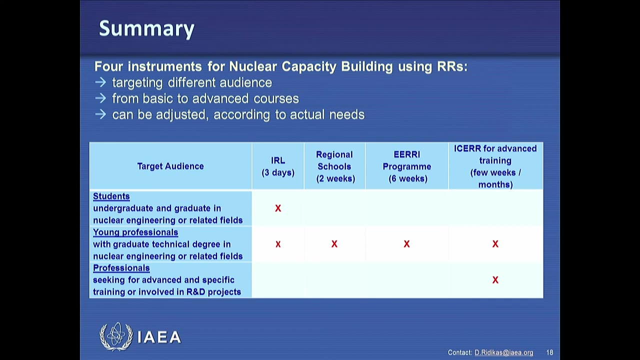 for the organization. So we can propose, thanks to these designated centers, advanced training and access to these facilities for the countries who need participating. So, in summary, we believe that these four important instruments will cover at least part of your needs from the member states.